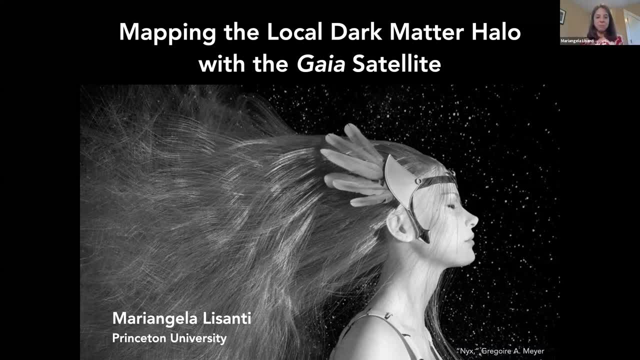 So you'll just have to kind of keep an eye out for when she makes an appearance again later in the talk. But I want to start off with a bit of history. Our attempt at trying to map out the dark matter in the Milky Way really started in the 1970s and 1980s with work by Vera Rubin and collaborators. 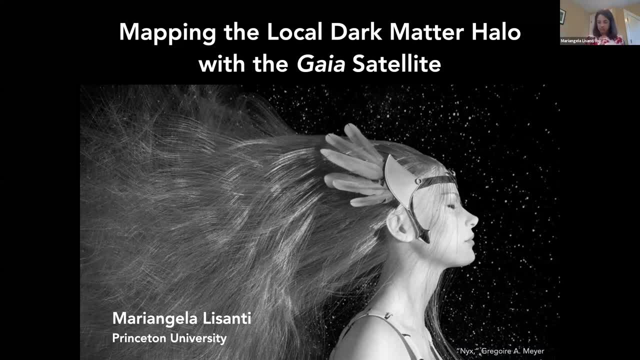 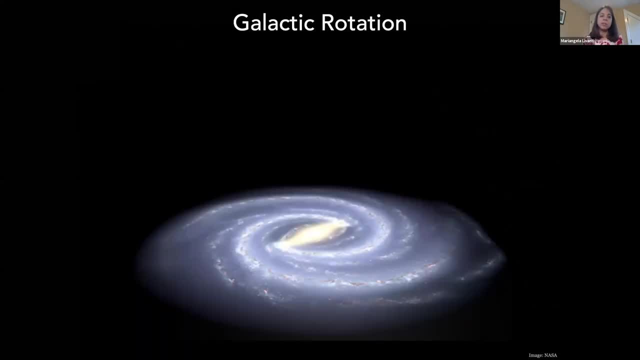 My slide is not advancing one second. There we go, By Vera Rubin and collaborators, where they were looking at rotating change, rotations of galactic disks, And what they found was the fact that as you move further out, farther away from the center of the galaxies, the rotational velocity of, let's say, gas that's in. 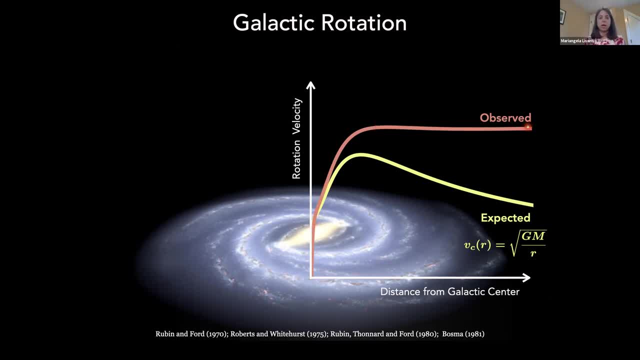 that galaxy seems to asymptote, And that's contrary to what you'd expect if you were predicting the motions of that gas or those stars based purely on Newtonian gravity. Newton's theory would predict, in contrast, that the rotational velocity would fall off at large radii as 1 over square root of. 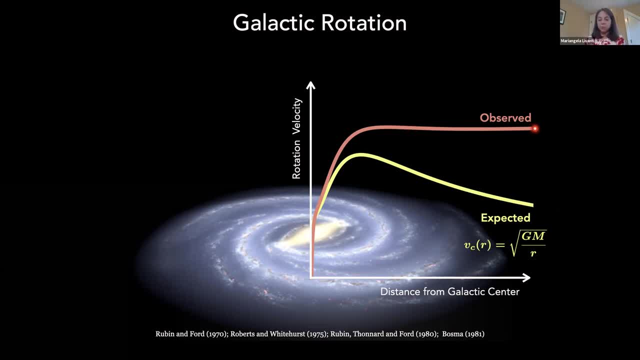 r. So this discrepancy between the observed rotational velocity and the expected rotational velocity really strongly indicated that there was some new, exciting thing that was going on, And there were several possibilities for how you can explain this. So one is you might say: OK, well, perhaps my theory of gravity is incorrect And I need to go back in and modify. 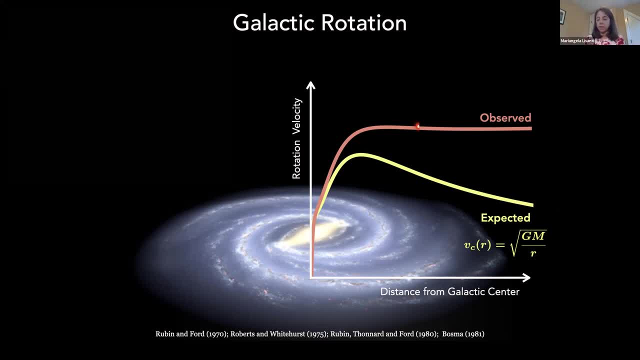 Newton's law, essentially to give me the pink curve here as opposed to the yellow one, And there has been some work, extensive work, on this since these early periods. They face a number of challenges. One big challenge is that they haven't been able to consistently reproduce data that we're getting. 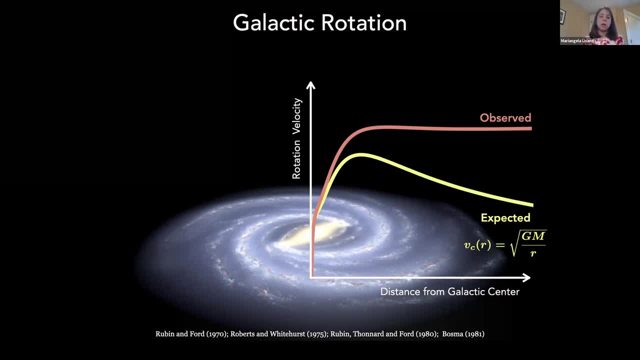 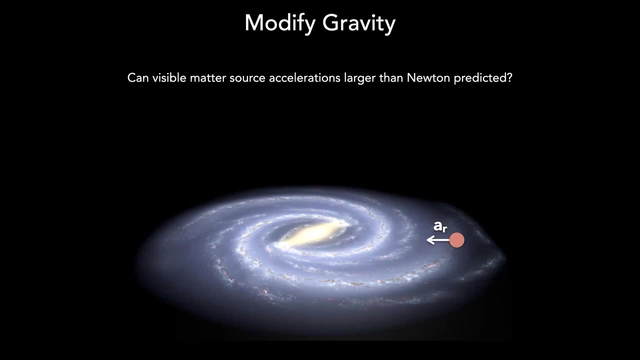 from the early universe, so from cosmological observations. But another challenge also comes in closer to home, so to speak. In particular if we just look at stars, the motions of stars in our galaxy, what these modifications to Newton's laws of gravity? 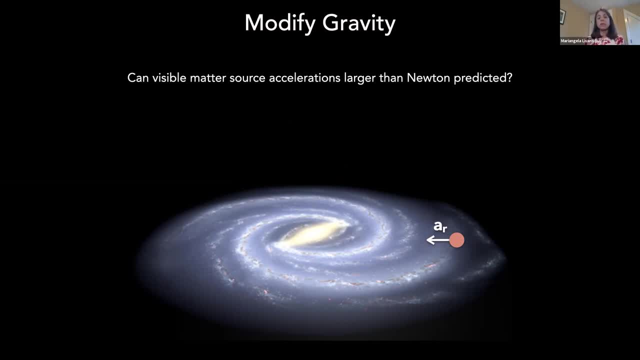 seek to do is to explain the fact that the radial accelerations of these stars is typically much larger than we would predict using Newton's laws. So you modify Newton's laws to try to give you an enhancement in that radial acceleration, such that you could then reproduce. 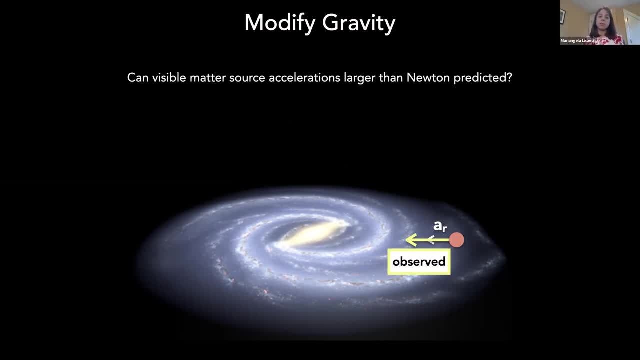 the rotation curves. Now, what these theories also do is they will have a consequence on the vertical accelerations of the stars. So if you have a theory that needs to predict a larger radial acceleration, what it does is it simultaneously predicts an enhancement in the vertical acceleration of the stars, And that's something that we can actually just go out and look for in the data. 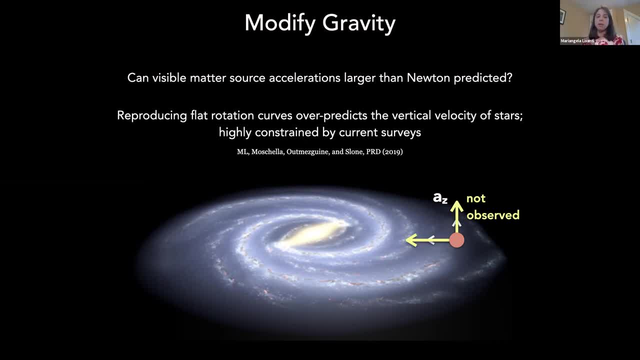 Especially locally near where the sun is in the Milky Way. we have some really good data on the vertical accelerations of stars, And what we find is that the vertical velocity of the stars is not enhanced to the same degree that you would expect from these modifications to gravity. So there's a number of challenges, then, to making this particular avenue work. 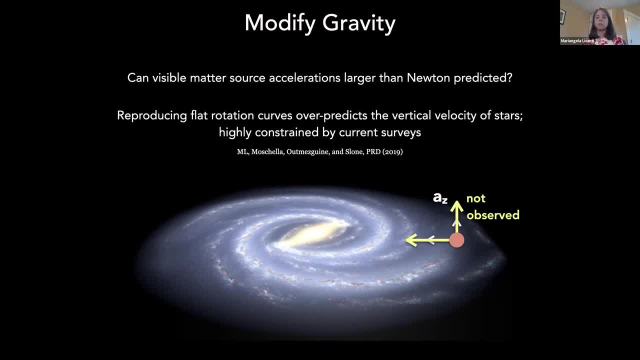 The alternate is to posit that there's additional matter in the galaxy, So to say that beyond the visible matter that we can see in the galactic disk, there's something else that's out there that's enhancing that total mass. And when you 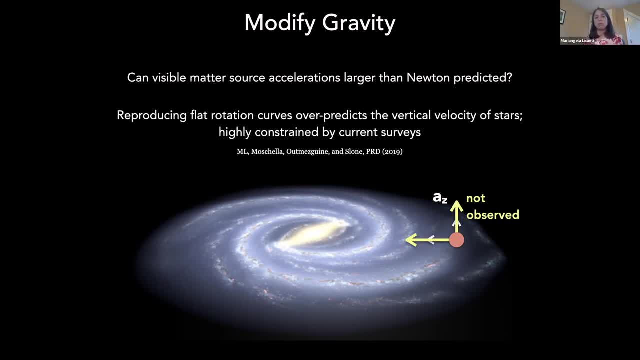 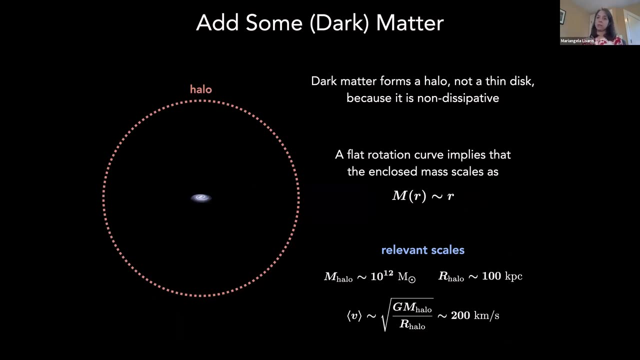 increase the total mass, then you should be increasing the rotational velocity of the stars and then that would be consistent with the rotation curve data In this picture we add in- we call it dark matter, this new matter that we add into the galaxy. dark because we don't see it. So that's in contrast to the visible matter that's in the disk. 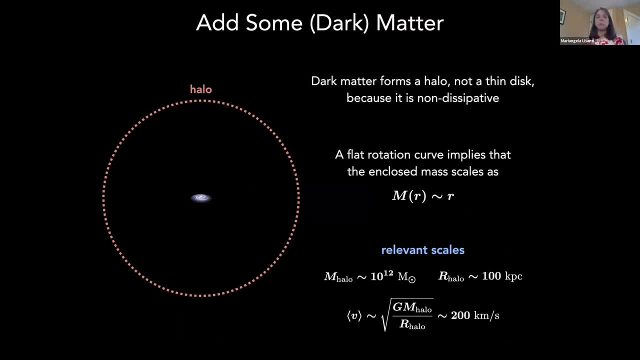 And in order for this additional matter to be able to explain the flat rotation curve data, it implies that the mass that's in this dark component needs to increase linearly with radius, And the picture that we have in mind here is that we have our own galaxy in the center. 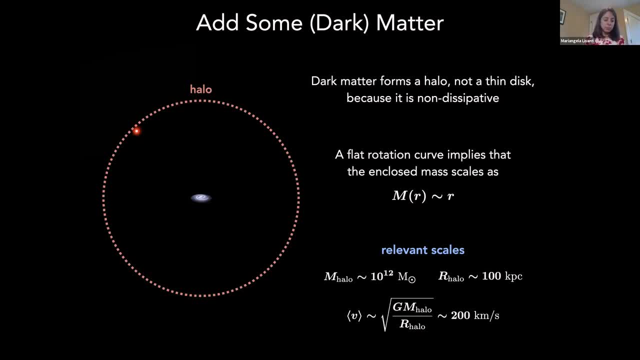 here. so that's the visible part of the galaxy and it's surrounded by a massive halo of dark matter. The scales here are actually really large. The scales here are actually really large. The scales here are actually really large. The scales here are actually really quite dramatic, in the sense that the radius here for this dark halo is almost about with the predicted radius for that dark halo is about 10 times larger than the observed radius of the disk. 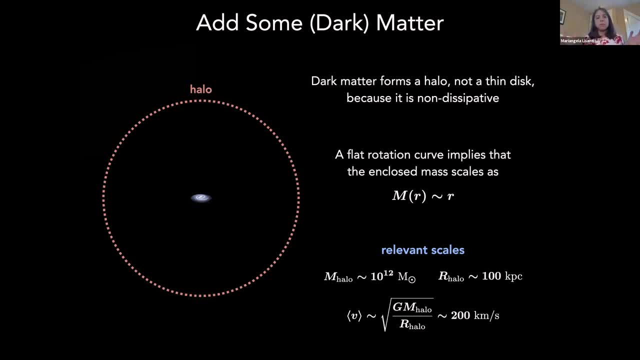 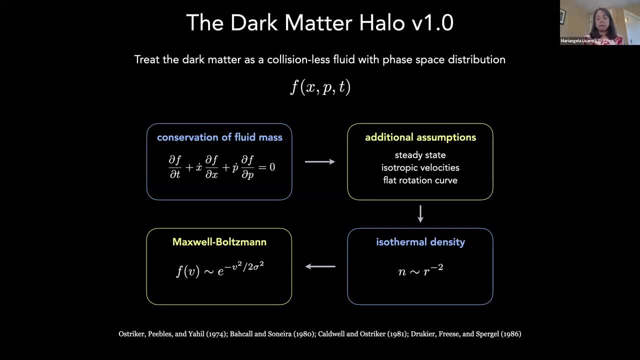 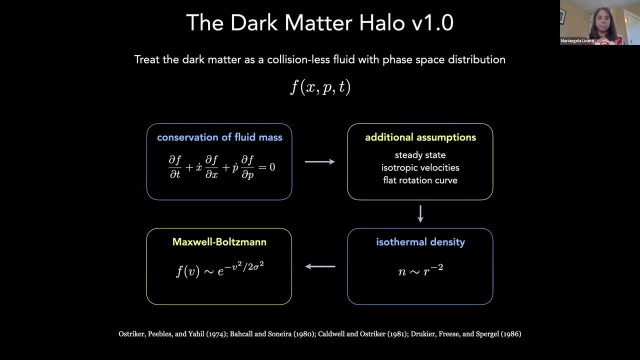 So this is essentially some kind of isothermal distribution for the dark matter. So this is essentially some kind of isothermal distribution for the dark matter. So this is essentially some kind of is uniformly distributed the dark matter. So this is essentially some kind of is不对. 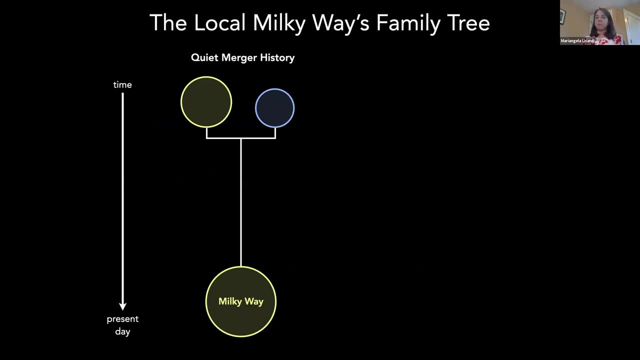 So this is essentially some kind of issequently any type of time. So this is essentially some kind of isumph. So this is essentially some kind of isumph as a as a family tree in some way. So the way galaxies like the Milky Way grow over time is by 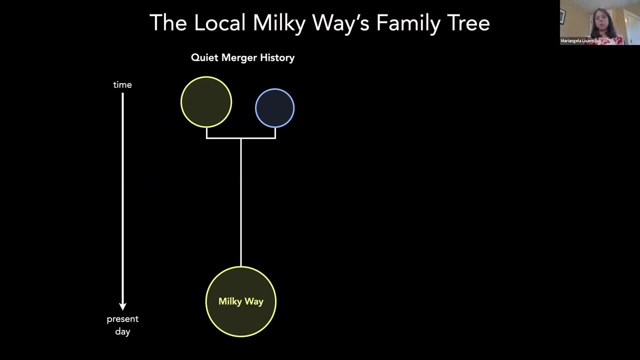 eating up smaller galaxies. Those smaller galaxies that get eaten up essentially end up donating their matter, both their visible matter, their stars and their gas, and also their dark matter, to us, and then we, we in turn, grow bigger. And you know, as of you know, looking back in time, we, 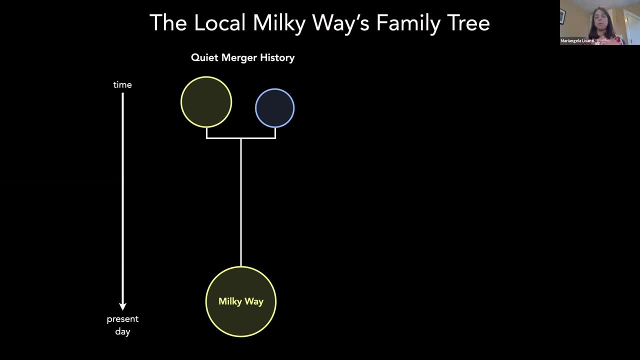 essentially want to be able to reconstruct that history of how our Milky Way formed by figuring out what all of these other galaxies are that we. we ate up in the process And, when you think about it, there's a variety of ways in which this can occur. So there's one extreme where the process 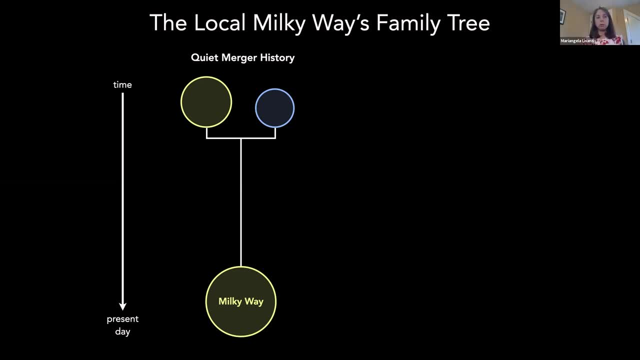 is really fairly quiet. So, for example, at some very early time you had two galaxies that combined together. then they pretty much just sat there. The system just had enough time to come into equilibrium. Nothing much else that happened. And then we have the Milky Way that we observe today. So that limit we'll call sort of a quiet. 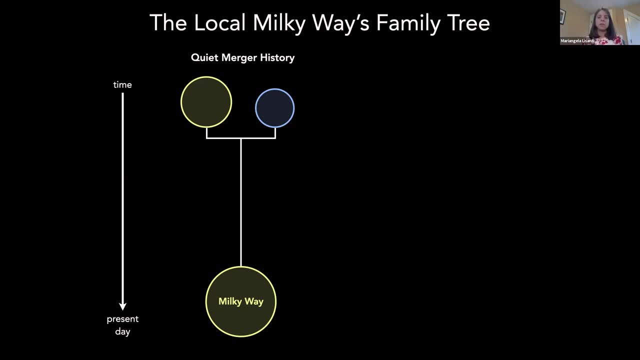 merger history. There isn't very much that's going on, And we can contrast that with a much more active picture of how our galaxy could have grown up, where a bunch of galaxies could have combined together, you know, up until very close to the present day, ultimately giving us the Milky Way. 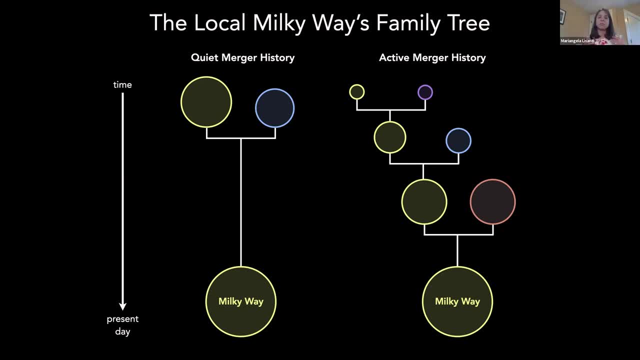 that we see today And in this limit the history of the Milky Way is very similar to the history of the Milky Way. The Milky Way is much more active. The system does not have time to kind of come into equilibrium because it's always just getting bombarded by some other galaxy that it's going to. 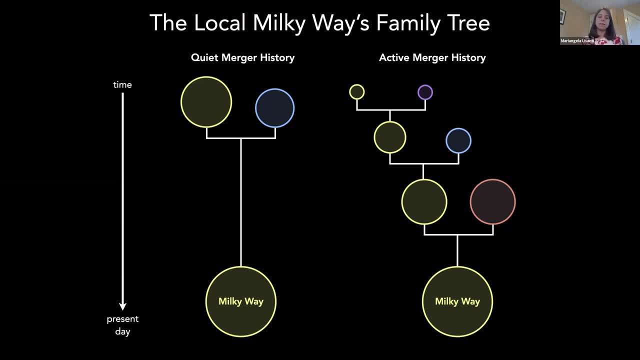 it's going to dissolve and donate its bits, And yeah, so this case here is the one, this active merger history here. if that's actually what happened to the Milky Way, oh goodness, there we go. if that's actually what happened to the Milky Way, then that steady state hypothesis would be broken. 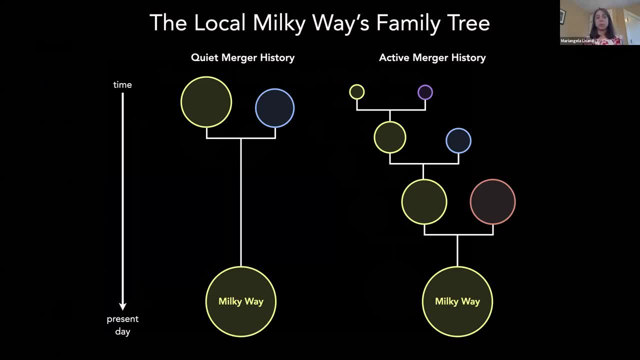 So the steady state hypothesis really only applies in the case where the merger history is really quiet and the system has enough time. the system here being the entire galaxy, has enough time to come into equilibrium and to settle down essentially. So, when we seek to try to figure out or put together a map for the dark matter and the 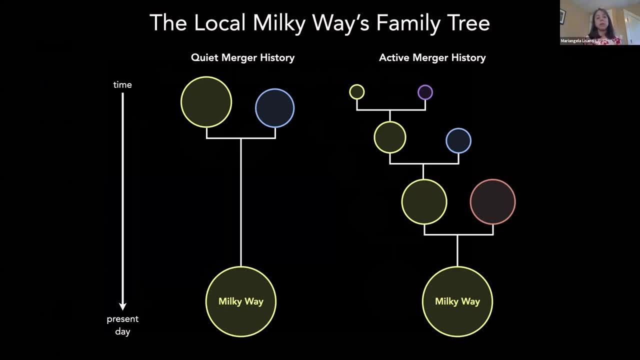 Milky Way. what it really involves us is understanding this formation process for the galaxy itself, understanding whether or not the merger history was quiet or active, understanding exactly what our relatives are, what galaxies joined up to form us, and then to use that information to figure out how the dark matter is distributed. 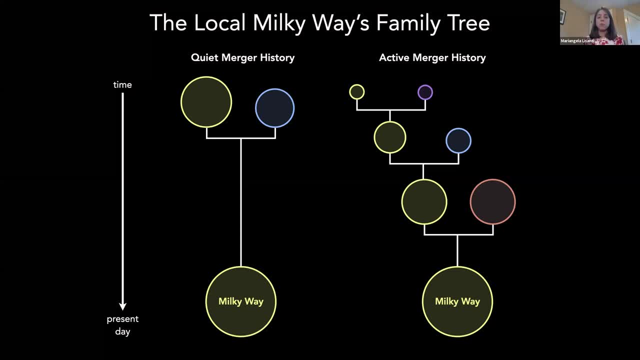 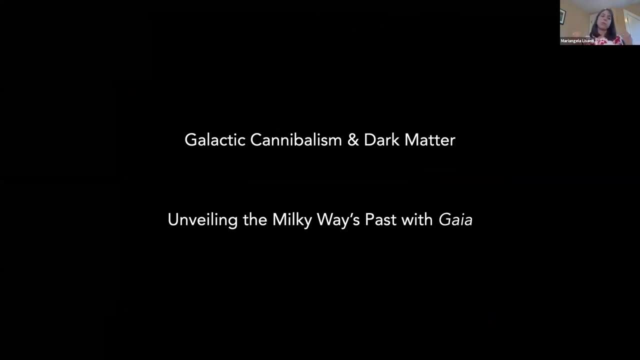 So over the course of this talk- the first part- I want to really just focus a little bit on the theory of how well we'll call it galactic cannibalism, so how our galaxy ate up all of these other galaxies. 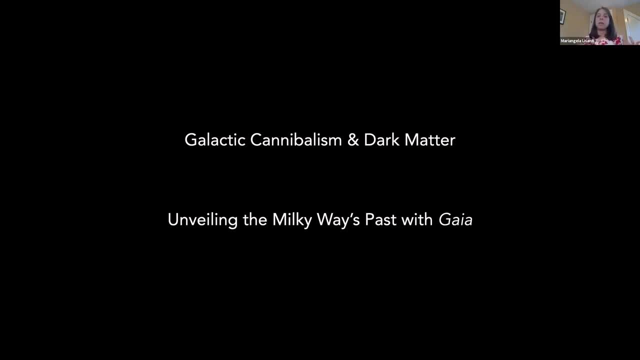 and what should happen to the stars and the dark matter in that process. And this first part is going to be definitely theory-based. We're going to be looking at simulation data and really kind of digging in deep there to understand what's going on in the galaxy. 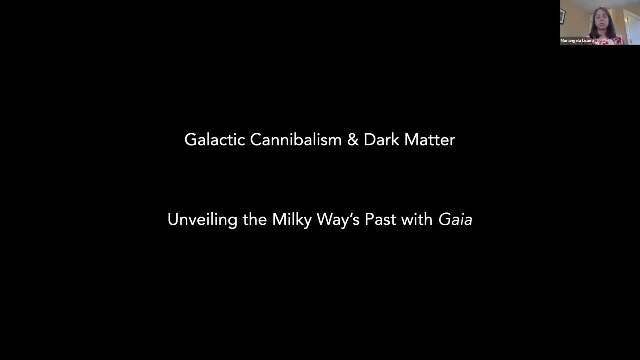 So let's get started. We're going to understand these correlations and how the dark matter and stellar distributions evolve as a function of time, as this merger history develops, And in the second half of the talk we'll be able to build on this theory foundation. 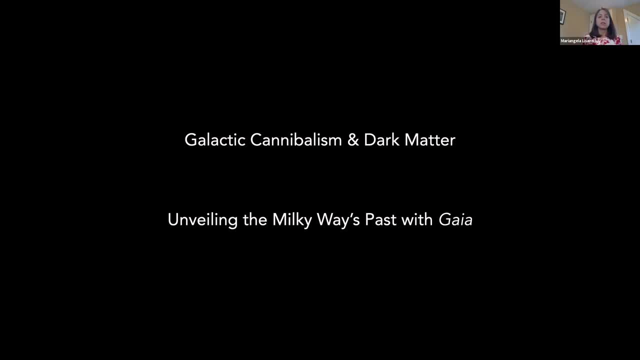 and start looking at data from Gaia to actually, you know, get our hands dirty and figure out exactly what happened in our own galaxy and what the implications are for the dark matter near us. So let's begin by actually just looking at some simulation of how a galaxy forms. 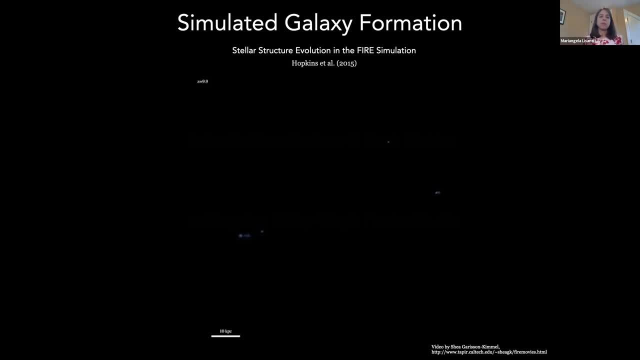 And, as I've already emphasized, in the Lambda-Cole dark matter paradigm, galaxies like the Milky Way are going to form by the mergers of other smaller galaxies. Now the video I'm about to play is going to show you a simulation of this happening. 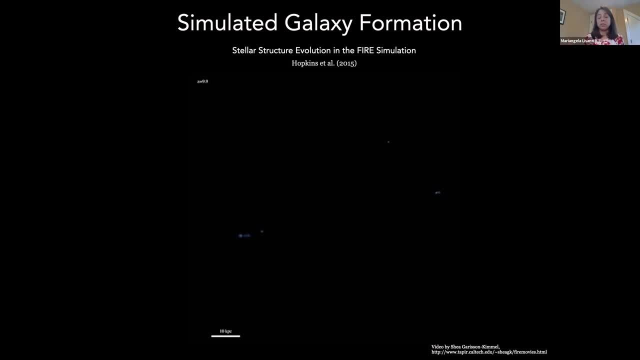 for a galaxy that's very similar. This is a simulation that's referred to as the FIRE simulation, So FIRE here stands for Feedback in Realistic Environments. These are some of the state-of-the-art simulations that we have available today that show how galaxies like the Milky Way form and how the gas, the stars and the dark matter. 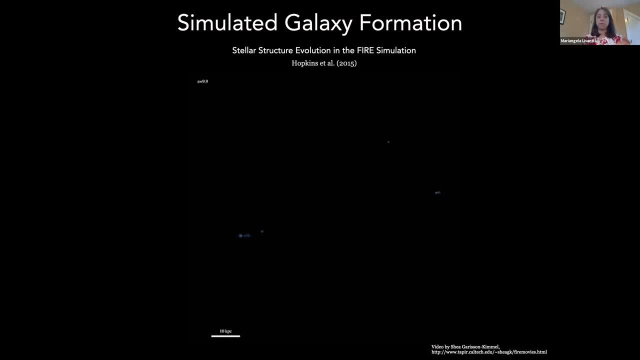 in the galaxy evolves as a function of time, starting from the very early stages up until today. The movement of the Milky Way is very similar to the Milky Way. The movie I'm going to show you is going to just show you the stars. The simulation is keeping track of the dark matter as well, but that's not included in the video. 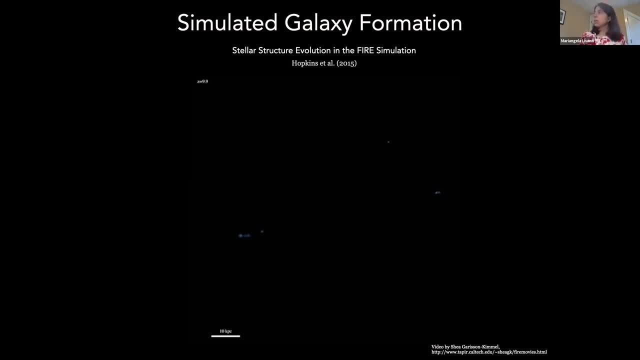 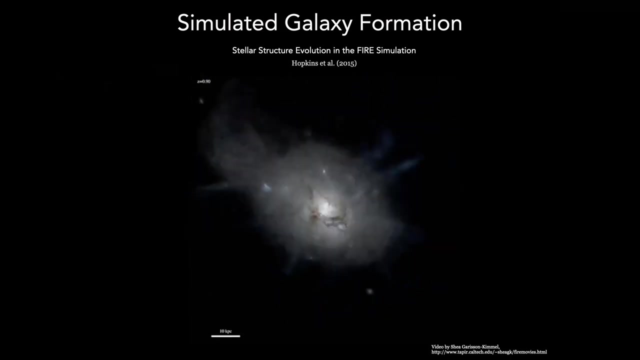 So I'm going to get this running. The bright spots, Oh goodness. Okay, one second, Here we go. So the brighter the area in that movie, that means that you have a higher concentration of stars And what you can see is that there's these. 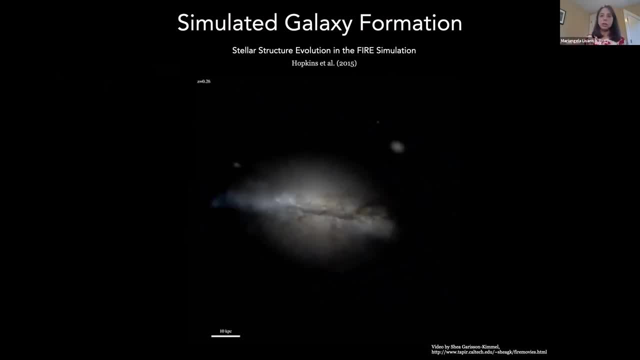 galaxies, so these bright patches that are flying in and they're combining to form that main disk. So let me just play that again, just to emphasize a few points. So in this initial stage there's a bunch of these galaxies that are combining. 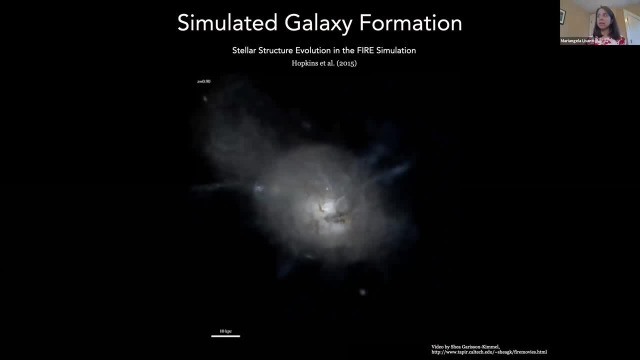 and actually the process is really quite violent and almost sort of chaotic. Once the disk forms and you can identify it, it does seem like things kind of quiet down a little bit. You have fewer of these galaxies, You have fewer of these mergers that are occurring as a function of time. 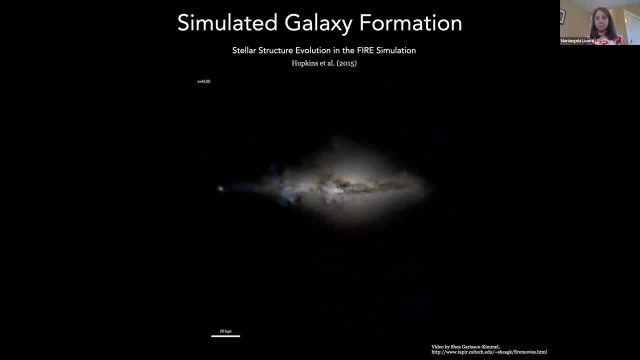 And then this is the way the disk looks today. So these simulations are extremely powerful for understanding how a galaxy like ours could have evolved as a function of time, But they aren't a direct representation, in the sense that we don't know exactly how many galaxies combine to form the Milky Way. 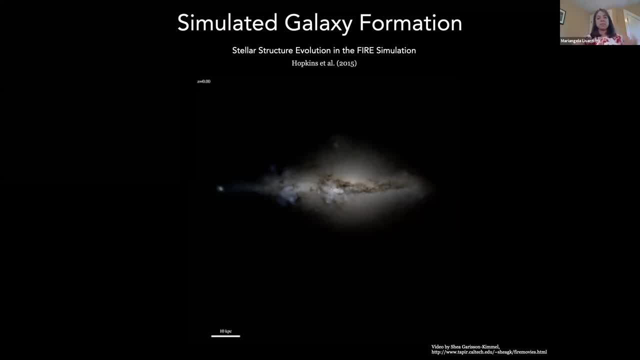 That's what we need to look in the data to find out. But the simulations do give us a realistic example- A realistic example of plausible scenarios, So they're a really good sandbox to play around with and try to understand what could be happening for our own galaxy. 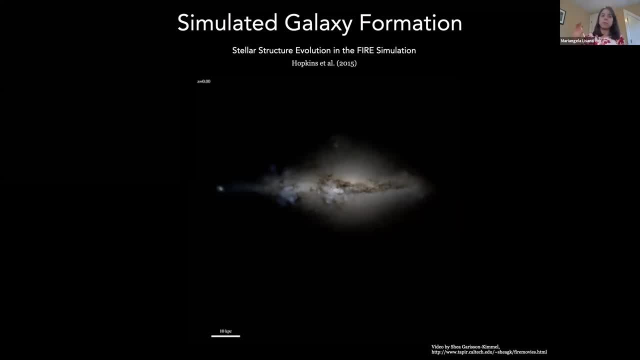 So what I want to do next is to kind of go into the simulation and break it down a bit so that to emphasize what's happening early on, when a satellite galaxy is falling into the Milky Way, and then what happens as that process evolves from there. 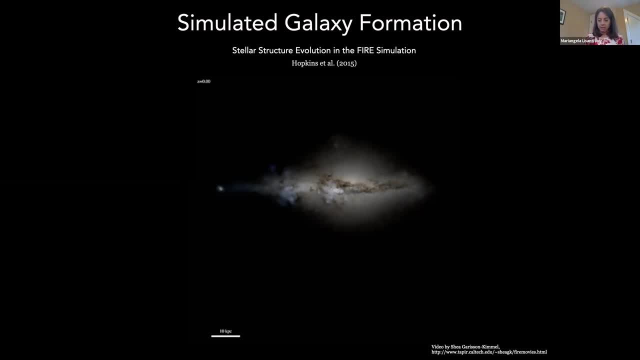 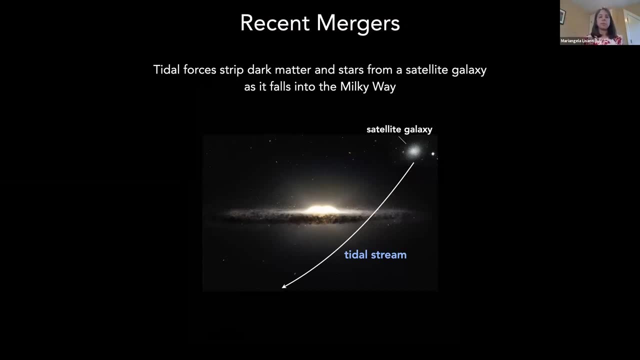 So when you have, Initially, some galaxy that's falling in, it's going to end up experiencing tidal forces from the Milky Way, because that's a much more massive system And those gravitational tidal forces are going to be stripping off dark matter and stars from that satellite galaxy as it falls in. 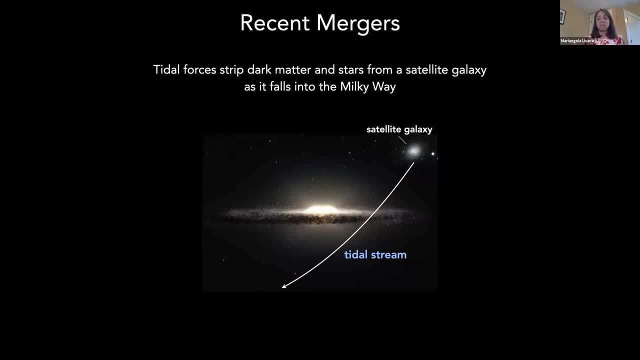 The material that's removed from that satellite galaxy sometimes is referred to as tidal debris: Debris Because it's just sort of left behind, and tidal because it's being removed by these tidal gravitational forces And initially that debris essentially just ends up roughly following the path that the satellite galaxy is taking. 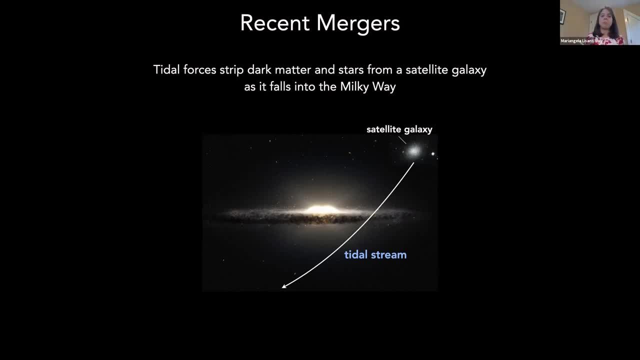 So you can just sort of imagine it being like left behind as a trail behind that galaxy, And we can. We actually have direct evidence of these kinds of streams that form these debris streams that form at least with stars. We obviously can't see them for the dark matter. 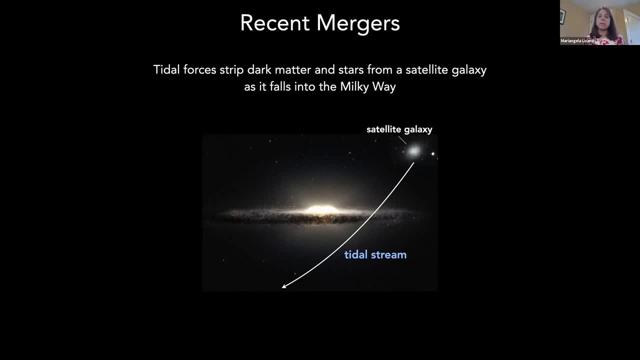 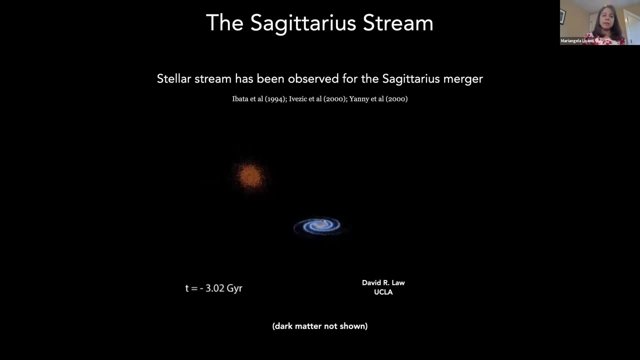 One of the most prominent and spectacular is arising from a known galaxy that's in the middle of being eaten up by the Milky Way. It's called Sagittarius And in this next video here, I'm going to show you what the process looks like. 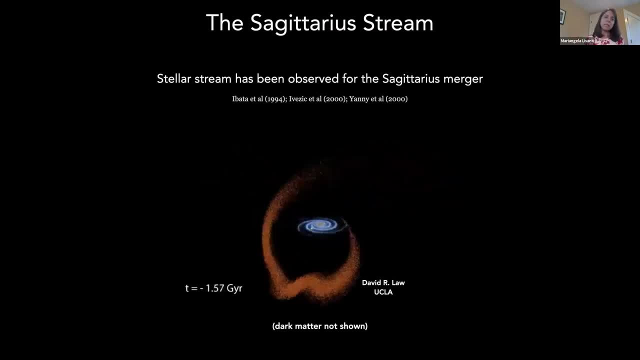 So this is a simulation of Sagittarius as it's falling into the Milky Way And you can see that, as it's being disrupted, it's leaving behind this trail of stellar debris And we can actually see in data these different, these individual loops. 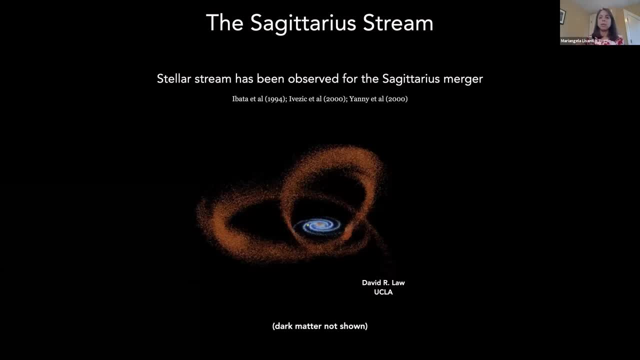 And those loops roughly trace out the path that's taken by the Sagittarius galaxy. as it's falling in Now, Sagittarius is pretty spectacular. We can make out these large loops. We also can still see the galaxy today, So it hasn't gotten completely digested yet. 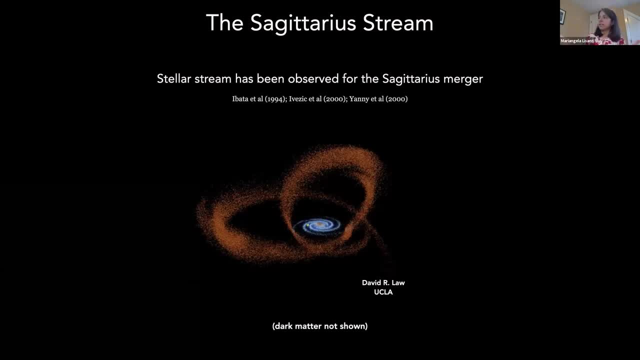 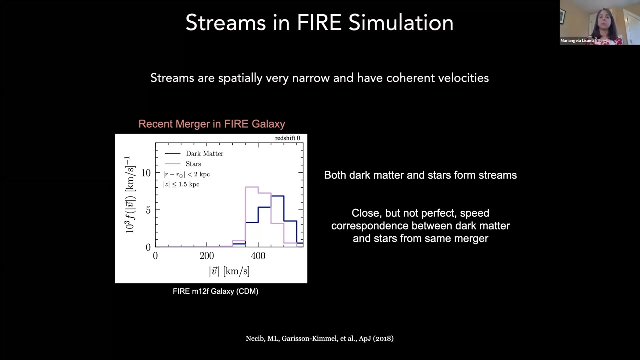 But it's just a really nice example of how you get these beautiful structures that form during these merging events in the galaxy. So what we can do in the simulation data, so in the fire simulation- is we can go in and find candidate streams that come from some merger event. 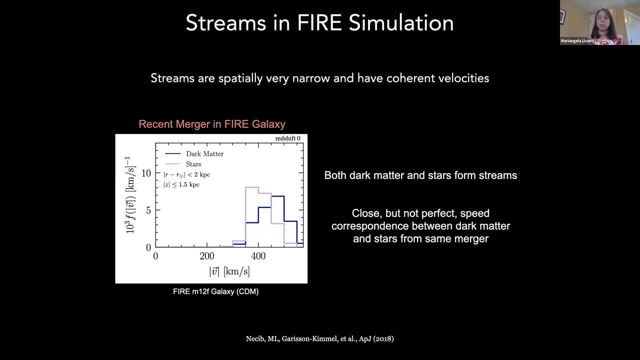 And we can look at how the dark matter and the stars from those streams interact And we can look at how the stars from those streams behave In general. the streams that form will typically be very narrow spatially, which you could have already seen from that movie of Sagittarius falling in. 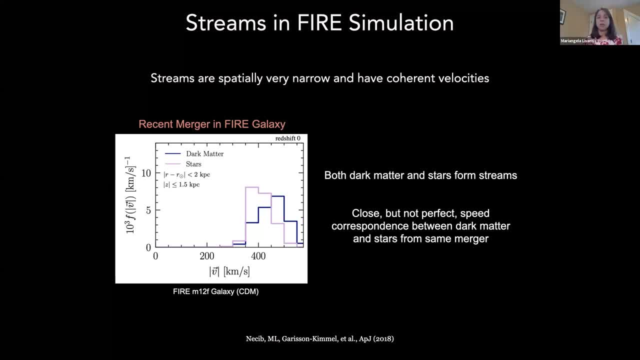 And also they typically end up having coherent velocities. So all of the matter in that stream tends to be flowing in one direction pretty coherently. And when we look in the fire simulation and we find candidates of stellar streams and then also look to see what the dark matter in the associated stream is doing, 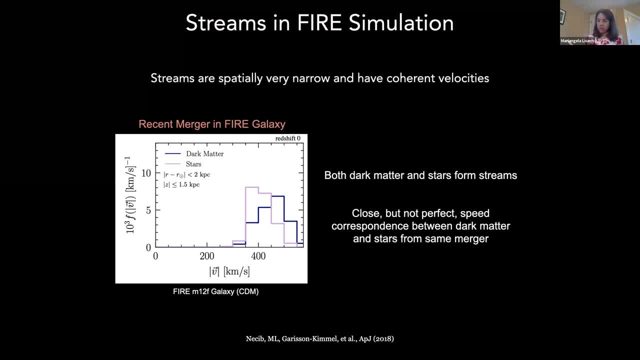 we indeed see, as illustrated here in this plot, the speed distributions for the stars which are shown in pink are pretty coherent. So they're peaked here, for this particular example, around 400 kilometers a second, And then also for the dark matter, the velocities are fairly coherent. 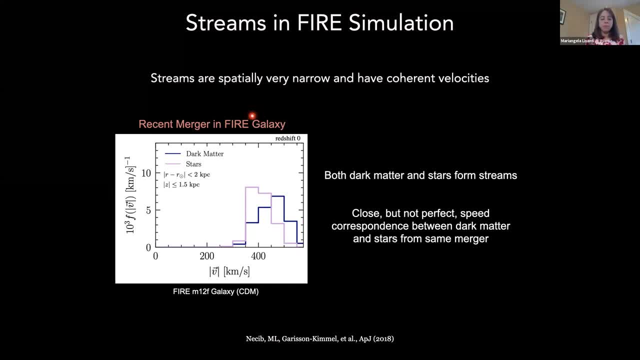 So in this particular example that I'm showing here from fire, you have both dark matter and a stellar stream that forms. We see this in the coherence of the velocity speed distributions, And one point I do want to make is that both the dark matter and the stars have roughly approximately similar speeds. 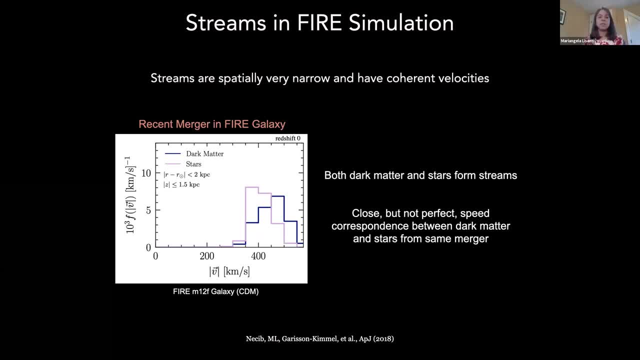 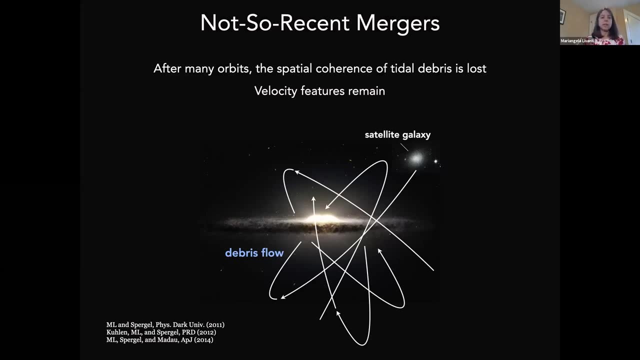 but the correspondence isn't perfect, And that's something that we generically see when comparing features in the dark matter and stellar distributions for some of these very recent mergers. Now let's go back to our little schematic. here We have our galaxy that's falling in. 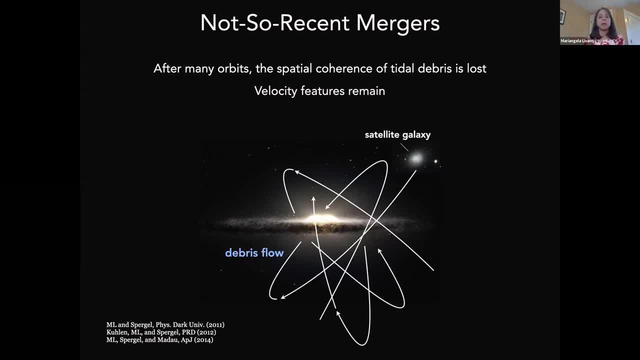 Now we're just going to sort of image what happens after the system evolves a bit. So the satellite galaxy, as it falls in, will make orbits around the host And in this process, where it's orbiting around and falling in, it's losing all of this material stars and dark matter. 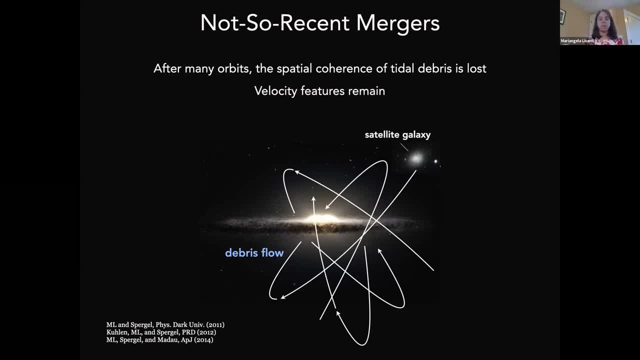 And all of that material is essentially falling in. It's essentially kind of getting mixed up together. It's starting to form kind of a little blob of stuff in the region. You can no longer make out individual streams because it's all getting wound up. 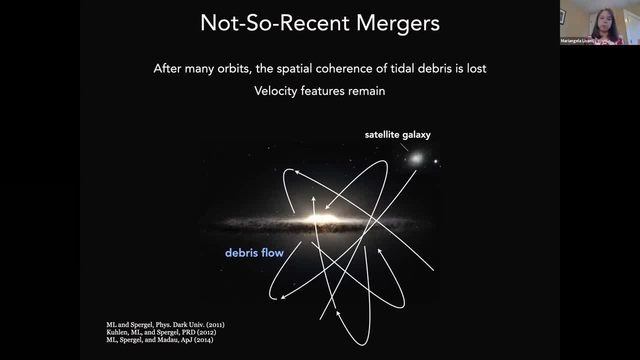 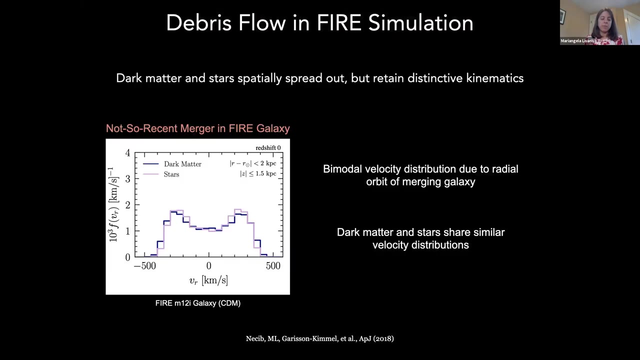 So the spatial coherence in this case just gets washed out. But interestingly, you do end up seeing some interesting velocity behavior that survives And that ends up being key for being able to actually identify the fact that such a merger occurred in the past. 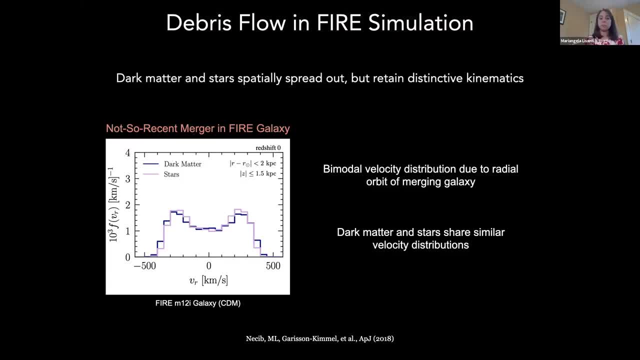 So in our fire simulations we can identify some of these not-so-recent mergers, So ones that sort of came in and have had some time to evolve and orbit around and fall in And what we find in these cases is that spatially there's nothing interesting to see. 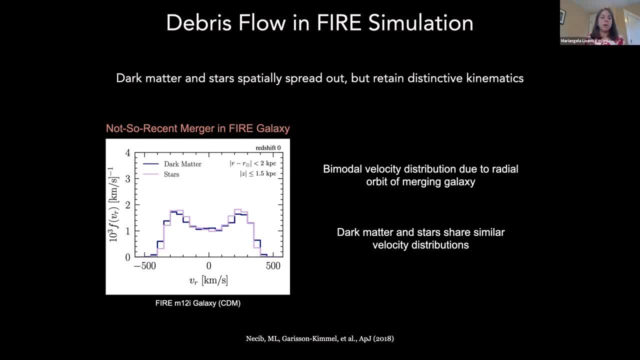 All of the material is kind of just all spread out. The stars, the dark matter is all spread out. But when you look in the velocity space you still end up having some interesting features. So for example, in the figure I'm showing here, 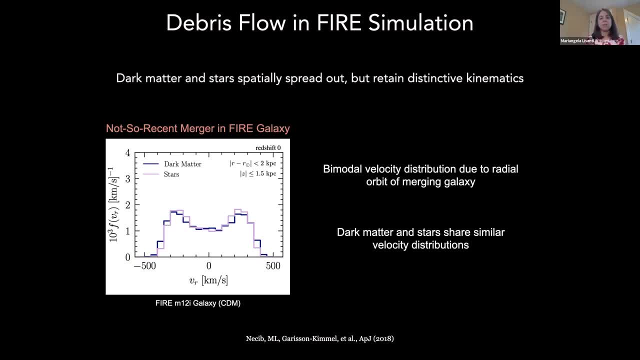 this is a plot of radial velocities for material that's been stripped from one of these mergers, And both the dark matter and the stars have this kind of interesting shape There. it's a bit bimodal, And that bimodality that you see there is actually a function of the orbit of the satellite that came in. 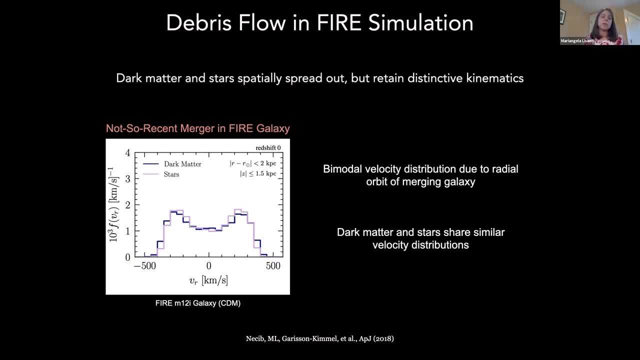 So this particular shape that you're seeing here in the velocity behavior is actually coming from the fact that the orbit of the satellite is pretty radial. Also, for these older mergers, the dark matter and the stars actually have a pretty good correspondence with each other. 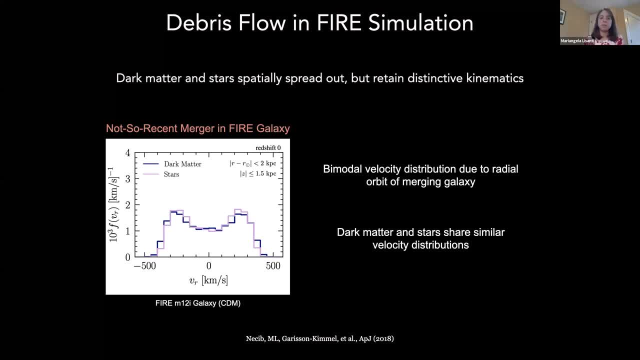 And that's really heartening from an observational point of view, because it tells us that if we can go out and actually map the stars in these kinds of substructures, then we have good reason to believe that the dark matter from the same mergers would follow very similar distributions. 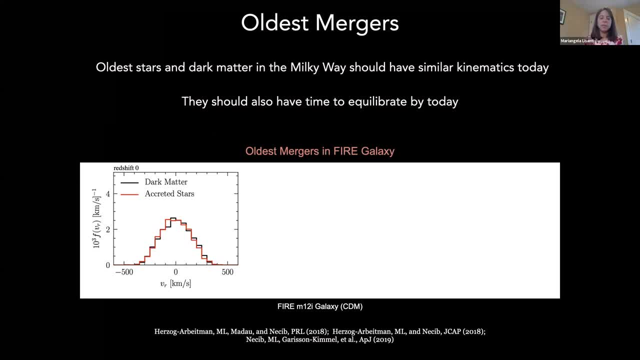 And lastly, let's consider the case where we have these satellites, these satellite mergers, but they essentially evolved to the point where everything got completely disrupted. So we had our galaxy fall in, it's made a lot of orbits and now it's just totally disrupted. 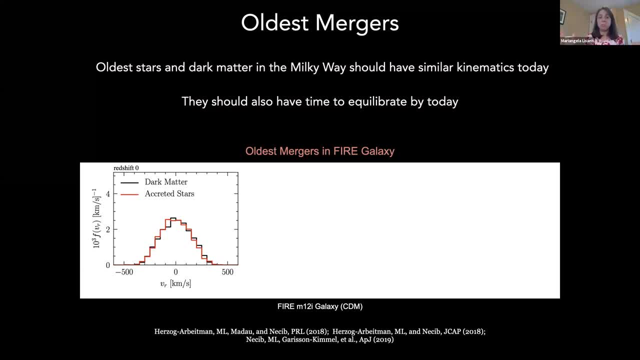 And we're just left with the material that's left behind. So these would be examples of the oldest stars and dark matter in the Milky Way And when we go, look in simulations at the really old components of the stars and the really old components of the dark matter. 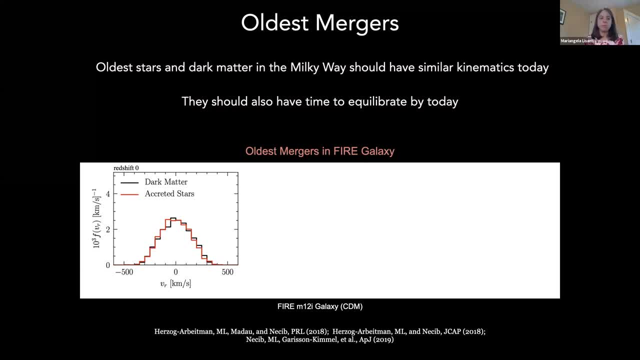 what we find is that they've all kind of come into equilibrium by the present day. And if we look here at this distribution equilibrium- here I mean that like everything looks fairly Gaussian, Kind of boring, no interesting shape to the distributions, And indeed actually when we look at all components of the velocity, 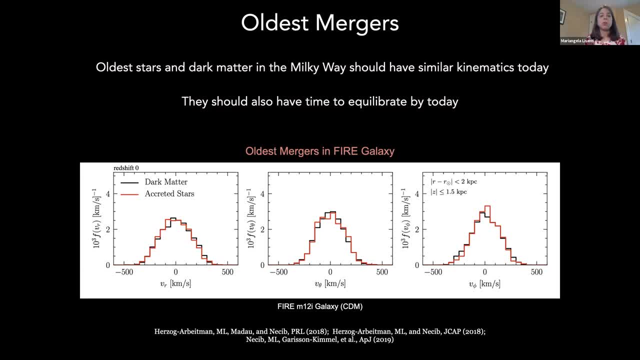 they all look fairly isotropic And in addition, all of the dark matter and the stars here have an extremely good correspondence with each other And that tells us that the dark matter that came from these really old mergers is tracked really well by the stars from those same mergers. 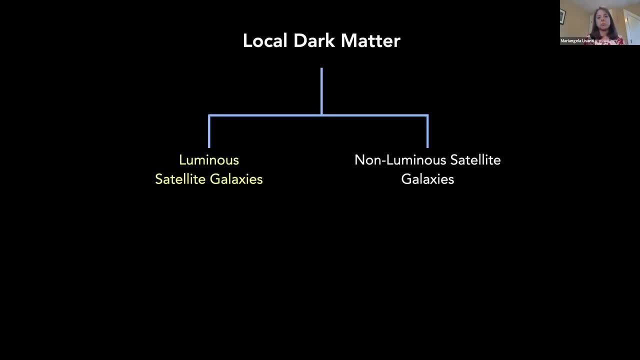 Okay, so let me kind of summarize the philosophy that we're going to take moving forward. The goal here is to try to come up with a distribution, a mapping, for the local dark matter near the solar position. The reason we want to do this is because that mapping is going to have a direct 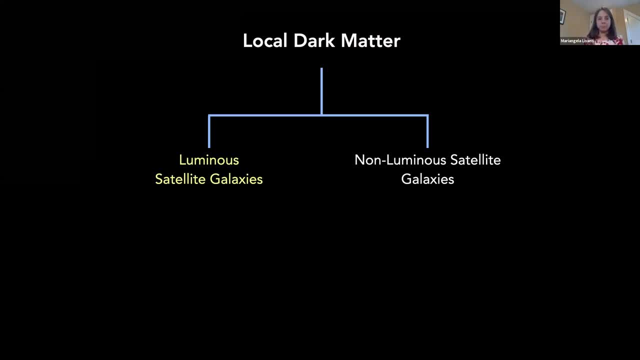 direct implication for any terrestrial search for the dark matter. The dark matter near us essentially came from these satellite galaxies that merged with our own. Some of the satellites that come in will have stars in them, and we're referring to those as luminous galaxies. 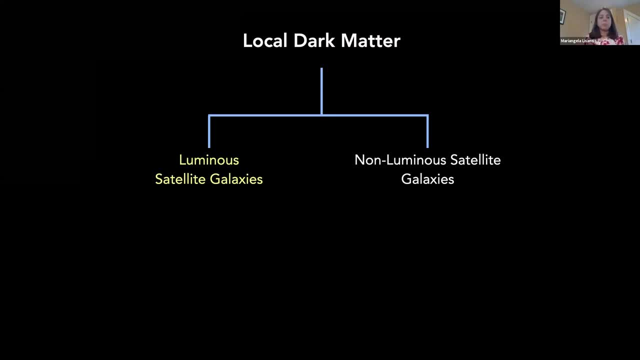 and then some of them don't have stars in them. Where we're going to get some traction moving forward is we're going to start looking, start trying to understand the dark matter that came from these luminous satellite galaxies. That's going to give us a way forward. 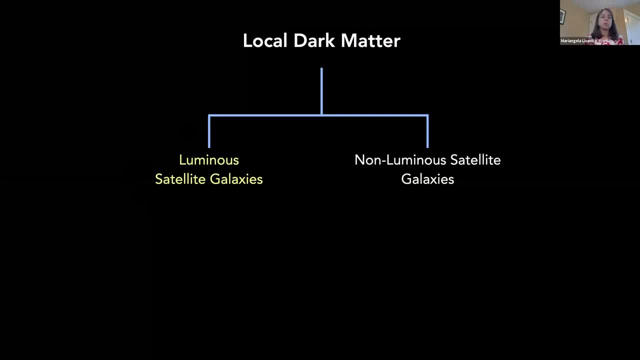 because we can use the stars from those galaxies to infer the fact that the murders actually occurred, And our task in going into the data is going to be to try to figure out what fraction of the dark matter came in from the really old mergers. 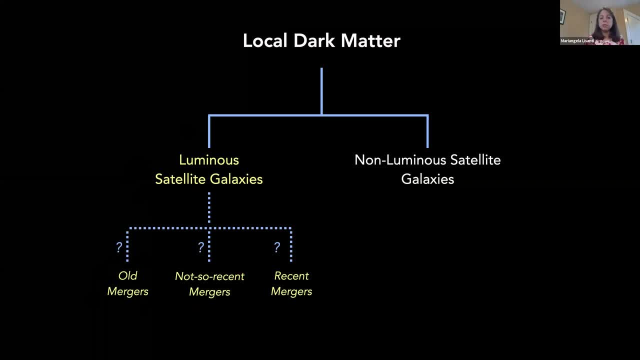 what fraction is in substructure from some of these not so recent mergers and what might have come in much more recently, Because the velocity information, the spatial distribution of the dark matter from each of these different classes would look different and would also have different kinds of implications for the experimental searches. 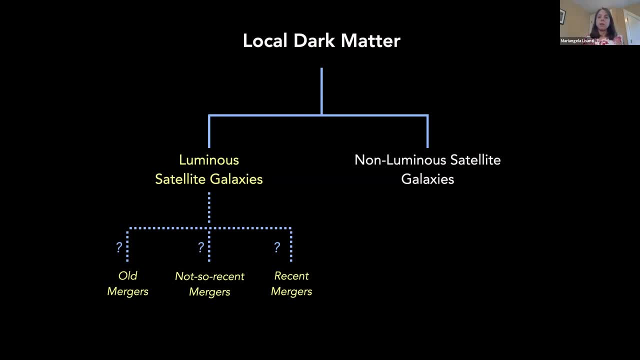 So we're in a really fortunate position that we have an amazing new data set that is actually allowing us to do this for the first time, And what I want to do now is just introduce a bit this data set and talk about how we can go in and mine it for this information. 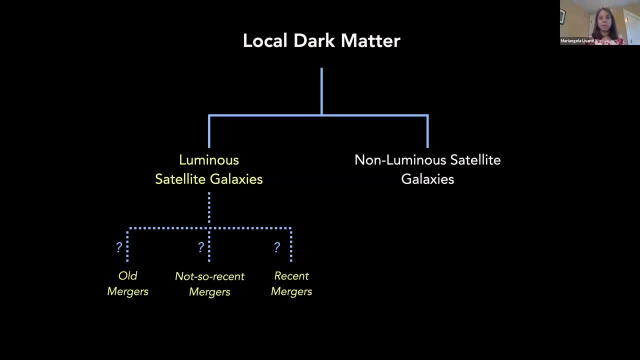 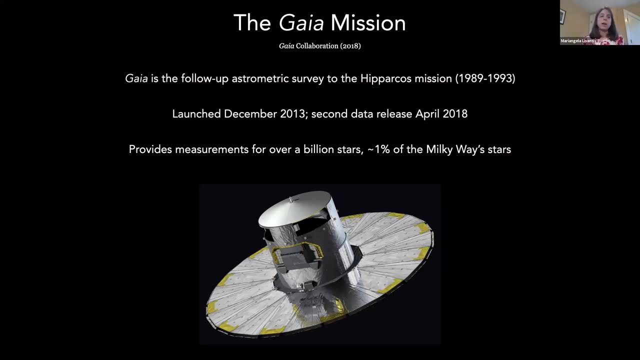 so that we can actually fill in this part of the diagram. So the data that I'm referring to is coming from the Gaia satellite. Gaia is the follow-up astrometric survey to the Hipparcos mission, which occurred in the early 90s. 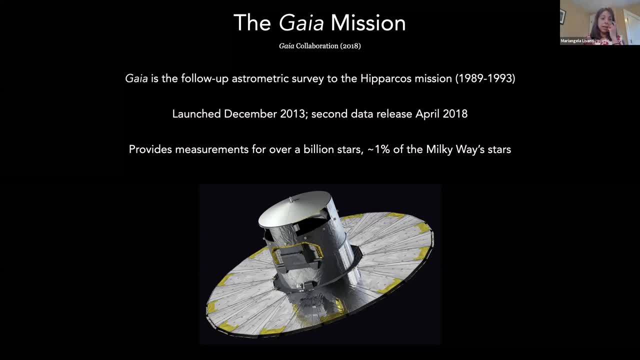 It's shown here on the slide. The satellite launched in December 2013, and the second data release occurred a couple years ago. The third data release is going to happen later this year: The mapping that Gaia does, which provides about a billion stars in the Milky Way. 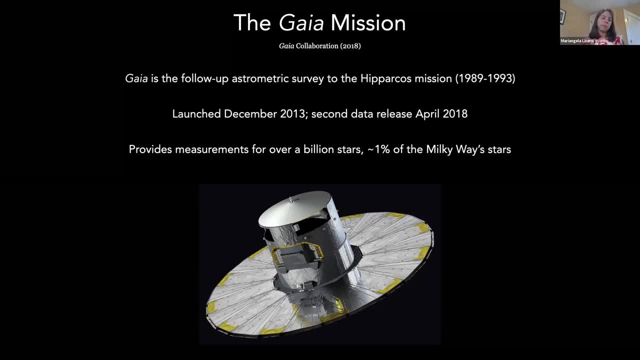 is unprecedented. This is about 1% of all of the Milky Way stars, which may seem like a small fraction, but it's actually the largest amount of data we've ever had on stars in the Milky Way, So that 1% is actually a huge advance forward. 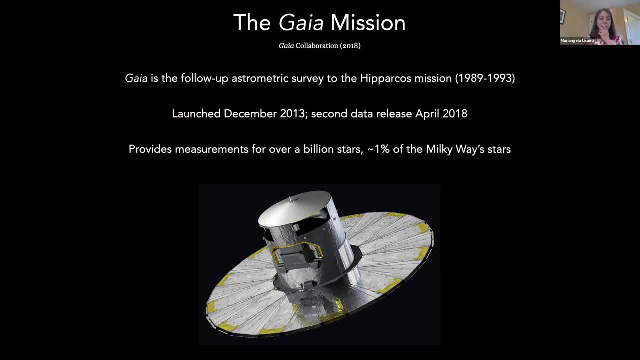 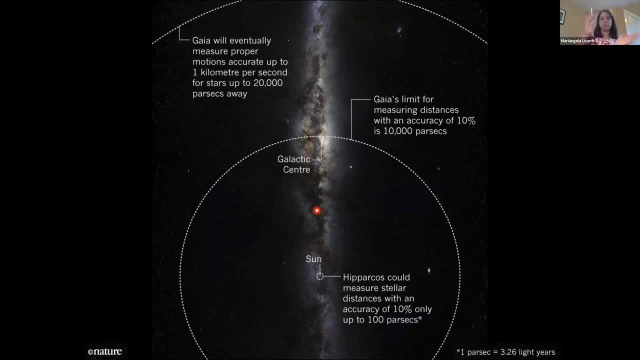 We've never had that many stars. And to kind of put this in perspective, this is an image of the Milky Way disk, but rotated, so it's vertical. So here's the center of the galaxy, and our sun is here, And the sort of region where Hipparcos had given us really good data. 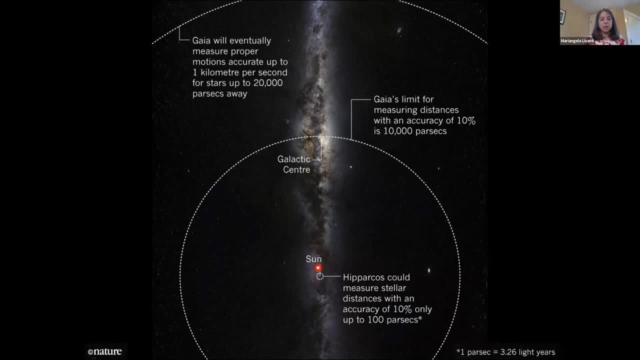 is indicated by this small little dash circle in here, And where Gaia gives us data that's of comparable accuracy is indicated by this circle here. So huge improvement in terms of area being covered And actually eventually Gaia is actually going to be able to give us. 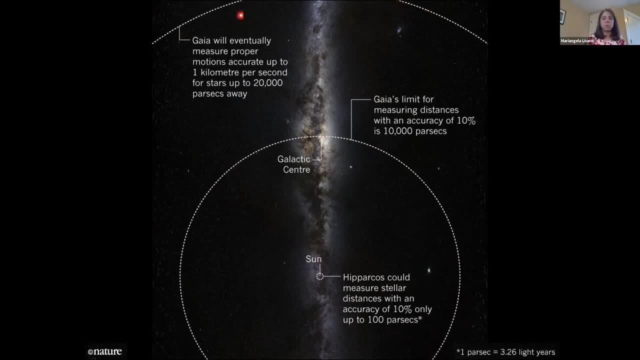 some really great, proper motion data all the way out to this outer circle. So, with this unprecedented data, what we want to do is essentially go on something of an archaeological dig in our galaxy. So, in the same way that when fossil hunters are looking for hints, 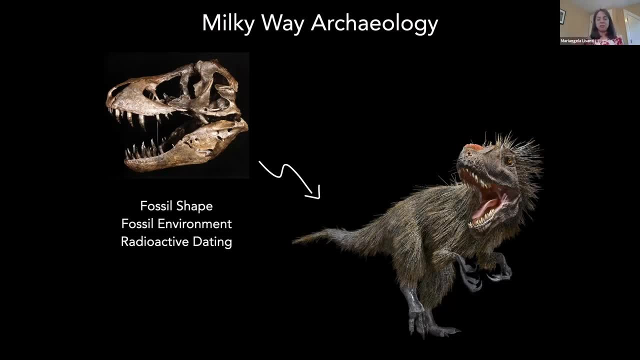 that some creature walked around our Earth many, many years ago. they'll go out if they find a fossil. they'll use information about the shape of the fossil, the environment it was found in. Perhaps they'll do some radioactive dating to try to guess at the creature that that fossil originated from. 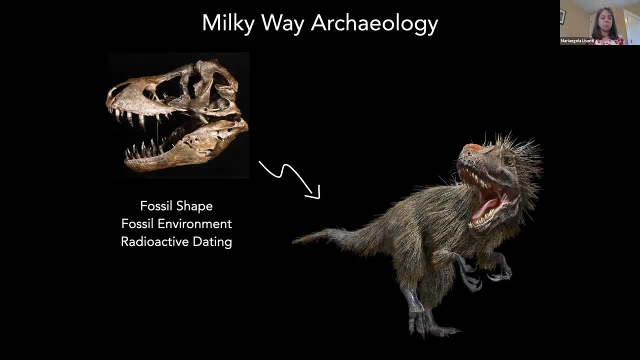 So we can go from this picture here of a pretty boring bone structure to a much more exciting image. This is a representation of a Tyrannosaurus rex with feathers, which I hadn't fully appreciated until I was working on this slide that there's a lot of debate going on in the community. 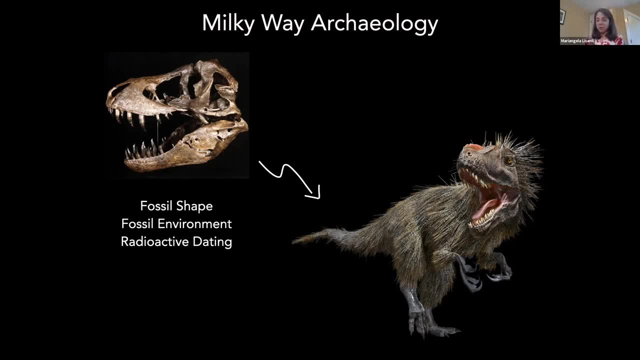 about whether or not a T rex should have feathers or not, But apparently there is a subset that does believe that Tyrannosaurus rex should have feathers, and this is what it would have looked like. In any case, what we want to try to do with the Gaia data is: 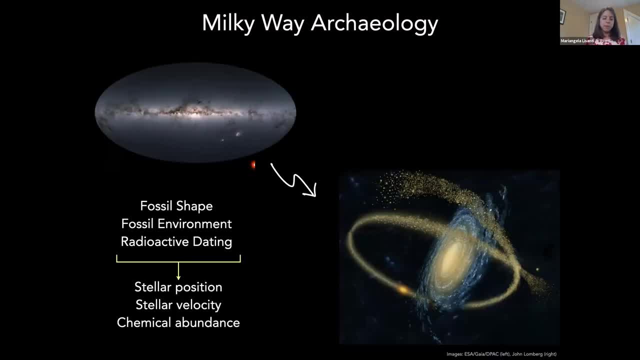 kind of similar to this. so we want to start with the map of all of the stars as determined by Gaia. Then, using information about the position of those stars, their velocity and perhaps any chemical abundance information of those stars, we want to then make this jump. 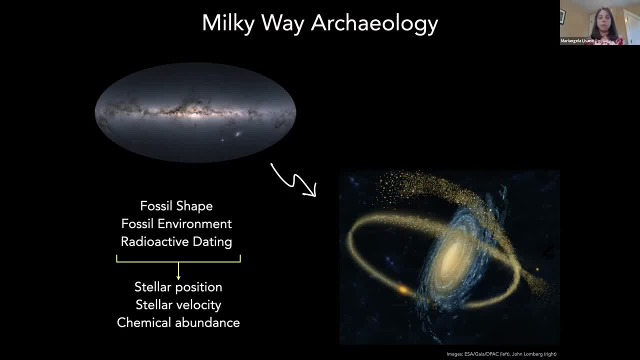 to infer something about the distribution of where those stars came from and whether or not there was some early galaxy that they originated from that fell into our galaxy and is being disrupted in our galaxy Now, this archaeological expedition that we're going to go on. 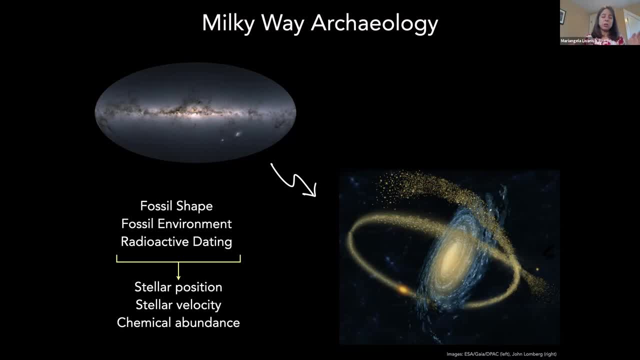 is extremely challenging. It's essentially a rare signal search And you can sort of see this here in the sense that when you look at the Gaia map up in the left-hand corner, most of the stars that you see, so where the map is lighting up, 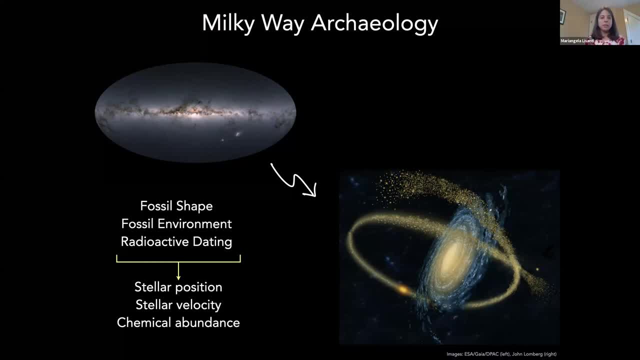 is right here along the disk plane And what we're actually interested in are going to be stars that are coming from these satellite galaxies that merged with ours. So the stars that are going to be coming from those mergers are kind of spread out in different locations. 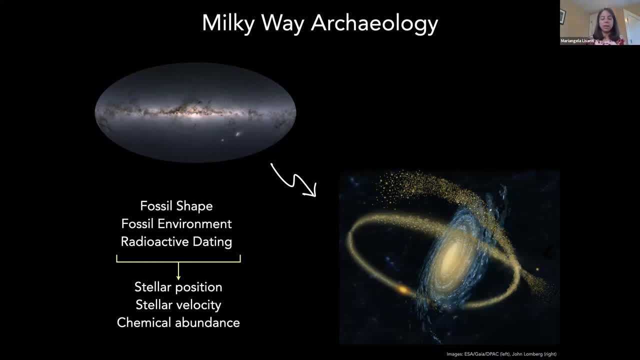 They're not necessarily concentrated in this disk plane And they're just comparably many fewer stars in the data set that correspond to this versus the stars that are actually in the Milky Way disk. So the task at hand is really like trying to figure out. 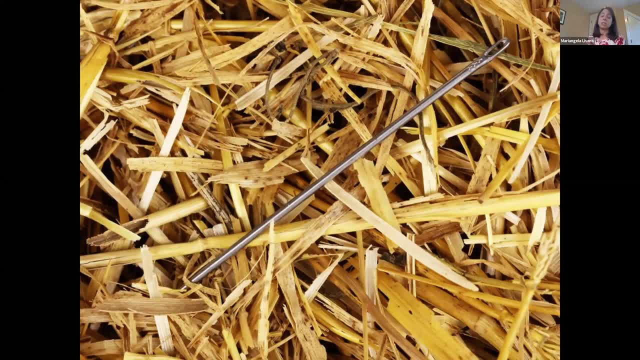 can I find a needle in a haystack? Because you're really trying to dig into this extremely large data set to find the sort of few special stars there that would tell you that something special happened in our galaxy. So we've taken several approaches to doing this over the years. 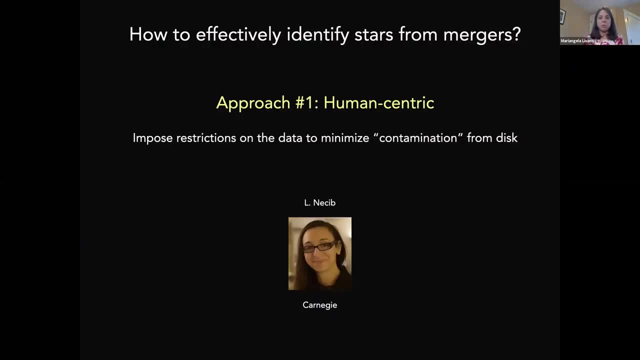 And I'm just going to highlight for you some of the results that we've gotten both ways. So the first approach I'll refer to as human-centric, which is perhaps a bit of a strange name, but that's meant to sort of emphasize the fact. 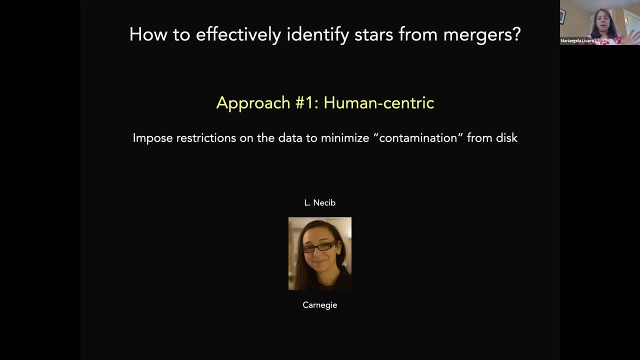 that with this approach we're really going to try to by hand impose a lot of restrictions on the data that will minimize as much as possible any contamination from the Milky Way disk. So I'll show you what we've gotten, how far we got using this approach. 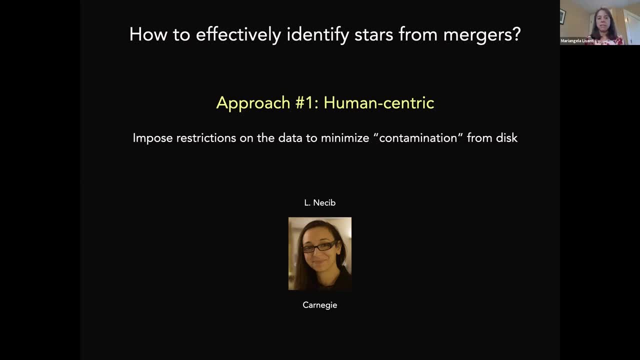 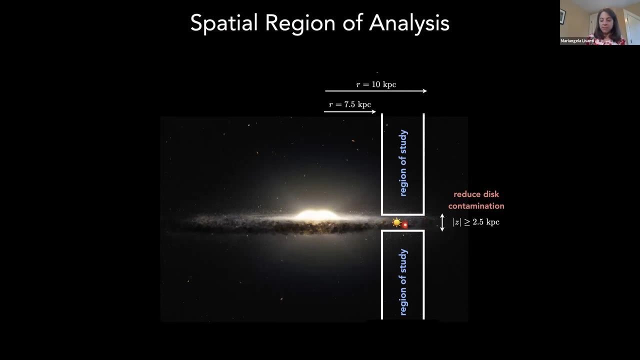 This was really spearheaded in large part by a postdoc, Lina Nassib, who will be starting a faculty position at MIT in the next year. She's currently at Carnegie Institute. Here's the region where we looked at the data, So we were specifically trying to avoid this area here in the galactic disk. 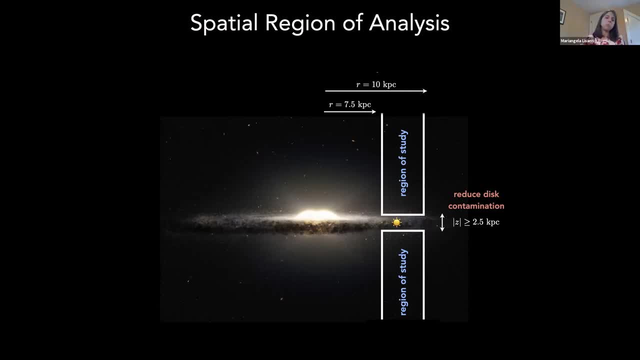 because, as I said, we were like specifically trying to remove as much data as possible from the region where we know there was going to be a large contamination. So we focused instead on these regions up and below the galactic plane. Even here, when we by hand remove, 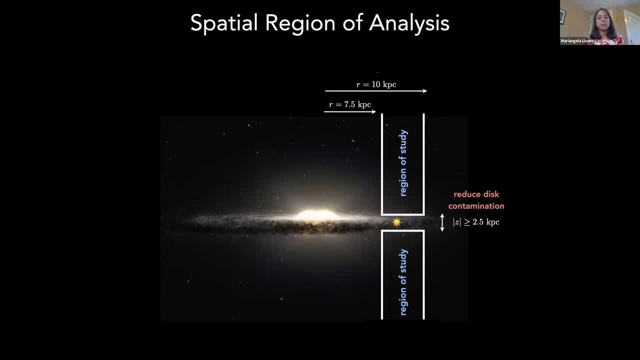 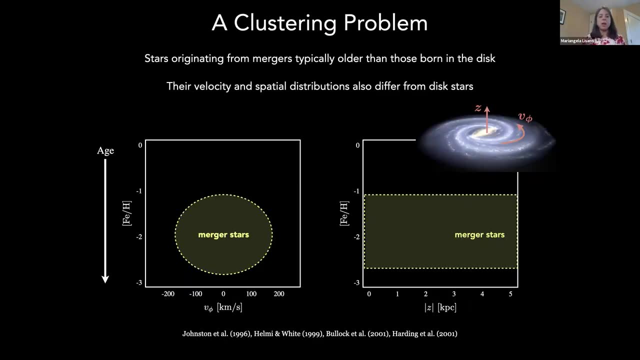 the dominant background. it's still a bit challenging to identify structures that could be coming from these mergers. Essentially, the problem boils down to doing it's a clustering problem. So what we have is a multidimensional space where each dimension in that space is set by data that we have. 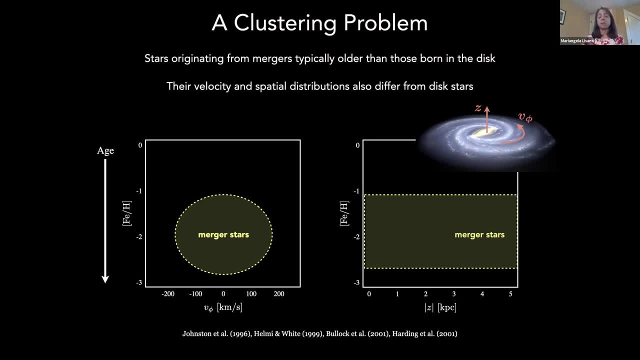 So, in particular in this case, we have information about the velocities of the stars and also some information about their chemical properties, So you can think of each of those as different axes in this multidimensional space, And then what we want to do is essentially find groupings. 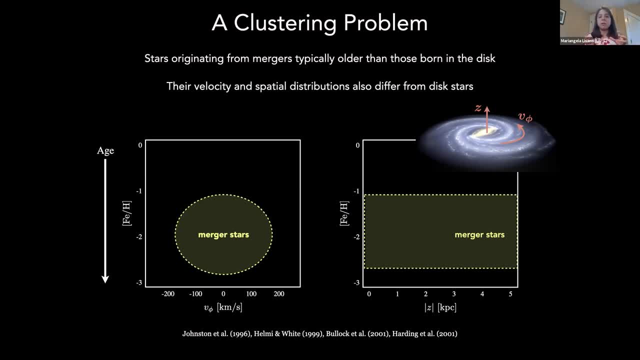 in that multidimensional space that we think are associated either with the disk or with some of these other interesting mergers. So what I'm showing here on this slide is just a schematic of how we approach the data, So we plot it in this multidimensional space. 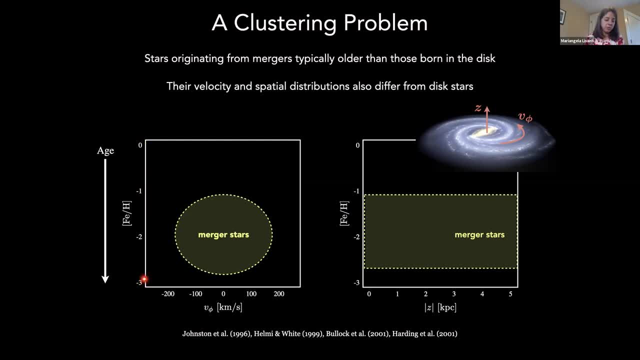 So here's a projection of it. Here's a chemical abundance here on one axis- This is rotational velocity on the x-axis, And what I'm showing here is roughly the region where we'd expect stars from these mergers to land. And, in comparison, here's the region. 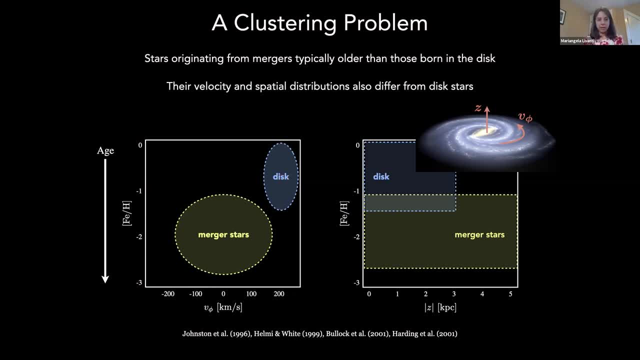 where we'd expect stars from the Milky Way disk to land, And so if our clustering algorithm works as we'd like it to work, it should efficiently separate out this grouping here from this other grouping here that would be coming from the disk. Now, obviously, as I've drawn this here, 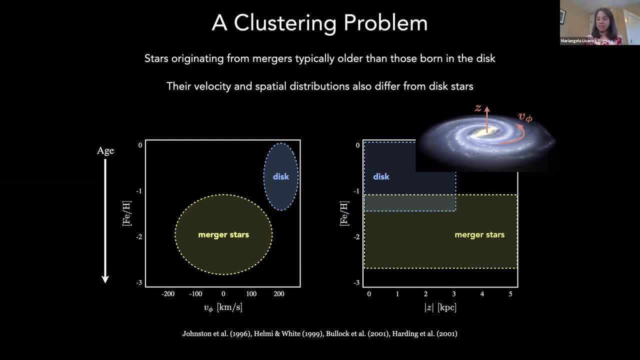 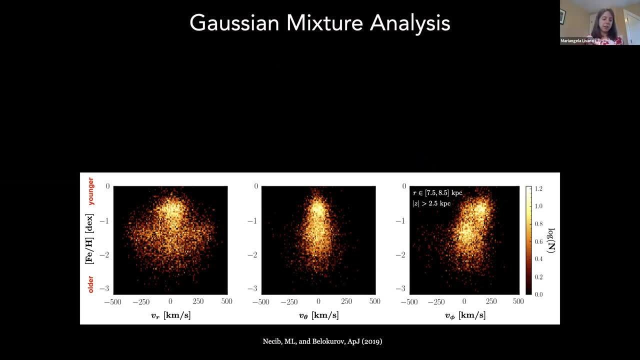 I was trying to make this seem very clean and clear cut. This is what it actually looks like when we open up the box And this is just the data plotted on these axes. So vertical axis here is just chemical abundance of stars. Horizontal axis is different components. 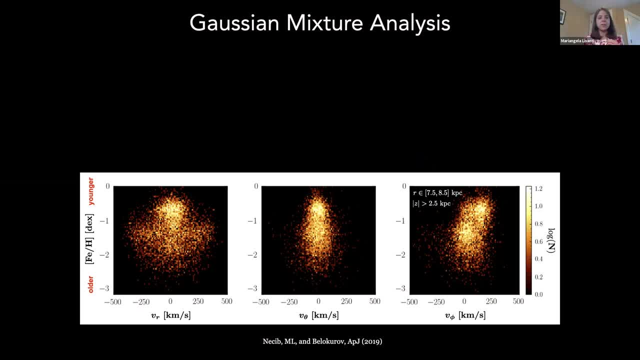 of the velocity of the stars, And you can see that when we actually look at the data, this seems like it becomes a lot harder. This actually just looks like one big blob, But what we really want to know is whether or not there's any statistical preference for breaking up. 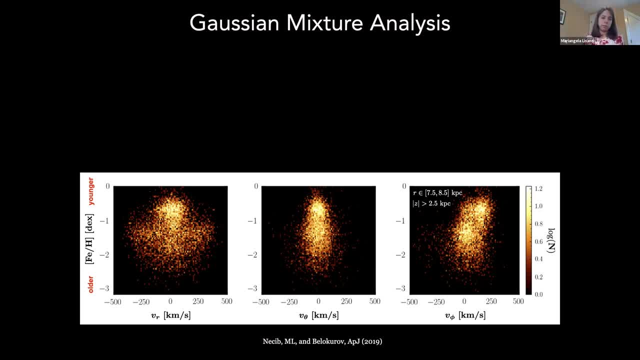 all of this information here into distinct components. To do this we apply a full Gaussian mixture model analysis, So we have a likelihood function that's set up to account for different components that can be added to the model, And then we run this likelihood on the data. 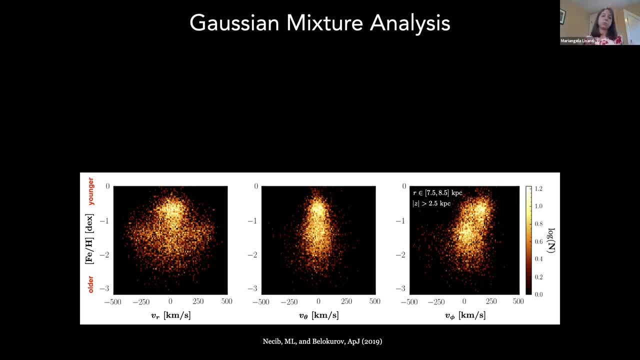 and see how many components are preferred and what their distributions should be. Here I'm showing you the result of that likelihood analysis. So these curves, these circles as drawn overlaid on this data diagram, are actually from the likelihood analysis. They're not curves that I've drawn myself. 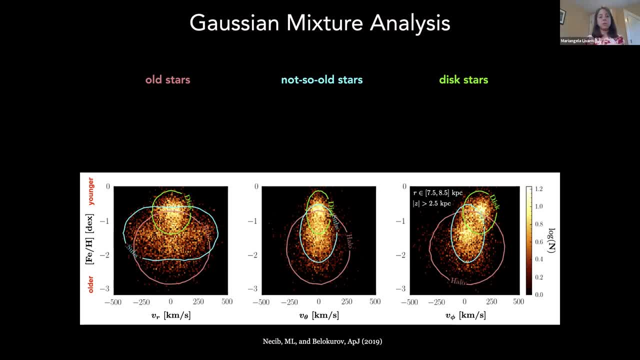 And what you can see is that there are essentially three different components that the mixture model analysis picks out. So it's picking here. This green circle is actually identifying stars that belong to the Milky Way disk, And the way you can see that is that these stars 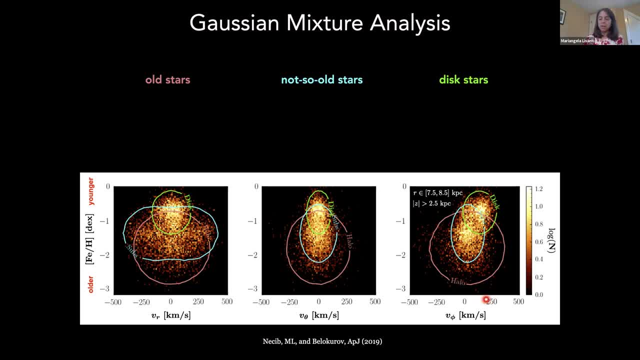 are kind of clustered around rotational velocities that correspond with the rotational velocity of our disk. So that's good, That part makes sense. Then we have the pink curve In each of these panels. that contribution is the oldest. This vertical axis, as I said, is chemical abundance. 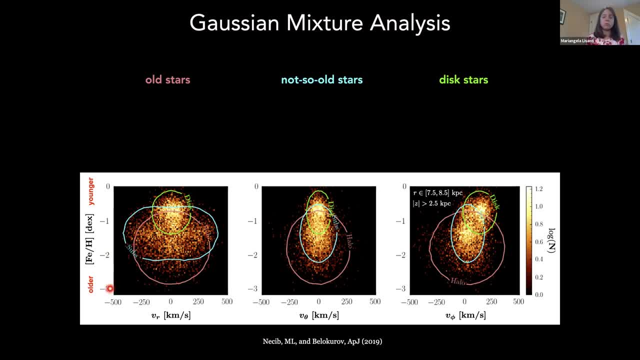 But as you go down here you're going to older stars. essentially It's a proxy for age. So the lower value of this chemical composition, the older the stars is. So this pink region, here are the stars that are the oldest ones. 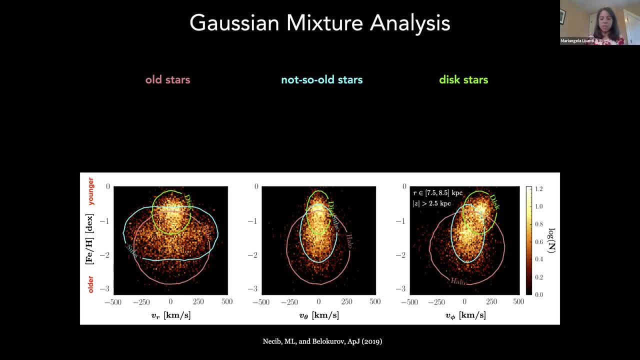 They're also roughly isotropic. So if you look at it in velocity space, the dispersion isn't very different in each of the velocity components. Then there's a third contribution that the algorithm finds, which is this blue region here. That's the one that's actually quite interesting. 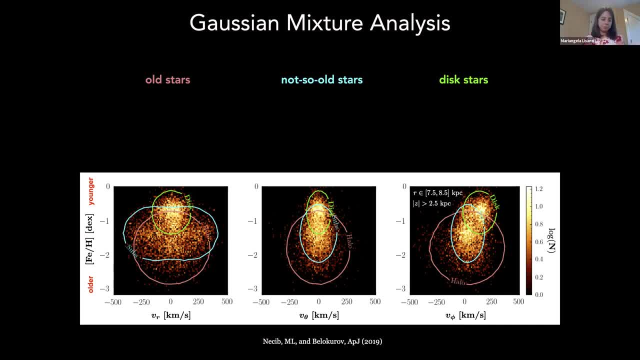 because that's like an intermediate set of stars. They're not so old. So for our purposes, where we want to kind of try to understand what this all means for dark matter, the way this corresponds is these old stars, the ones circled in pink. 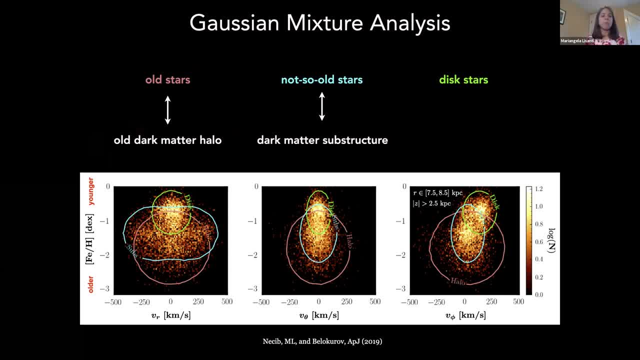 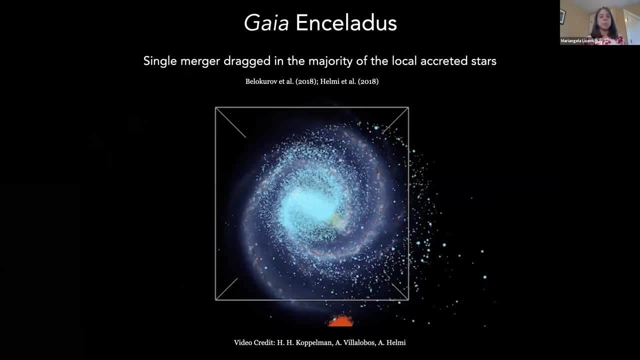 would be mapping out the dark matter that came from very, very old mergers And then the stars circled in blue would be indicating dark matter that came in from a more recent merger. And actually that more recent merger is quite interesting And people have only discovered this once: the second, Gaia. 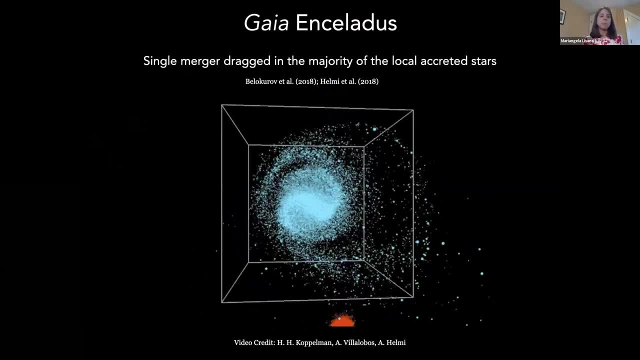 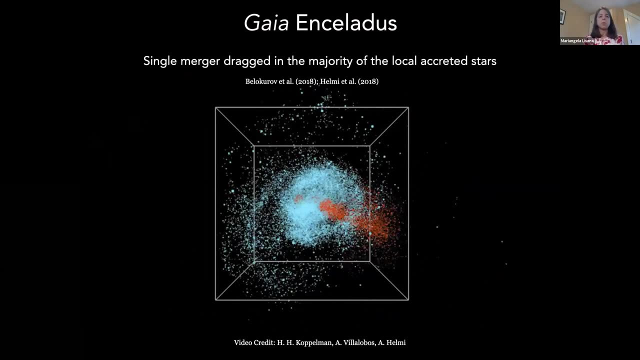 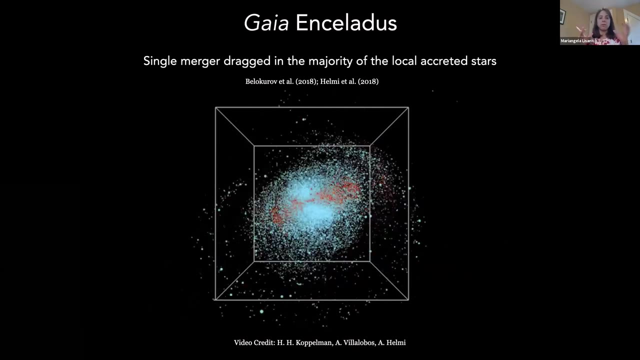 data release became public. This was first noted by the Center for Astronomy, Silly Belokurov and collaborators and Amina Helmy and collaborators. What they found was that there's essentially a single merger that dragged in the majority of the stars in the inner part of the Milky Way. 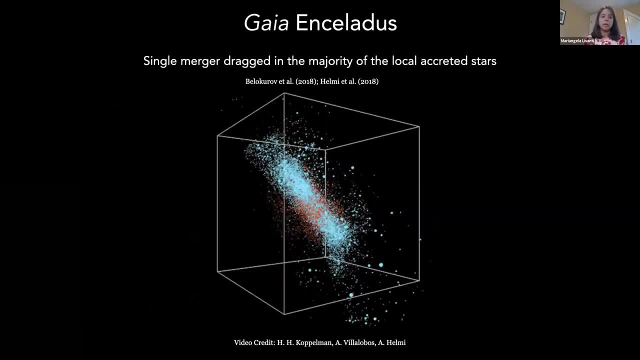 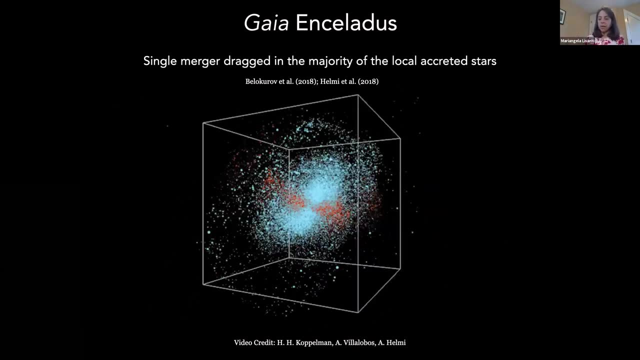 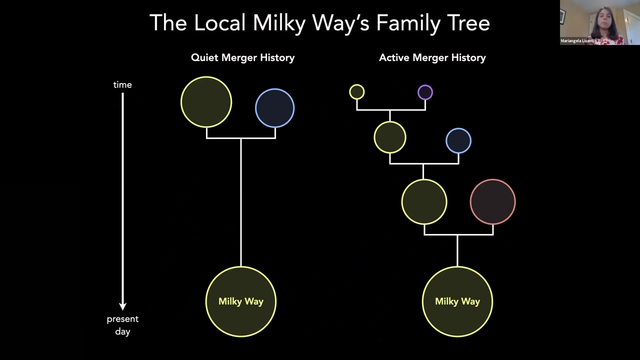 And that's what's being shown here in this simulation, That merger event, that galaxy is called Gaia Enceladus, And it allows us to come back to our family tree that we started off at the beginning of this talk And actually make some progress forward. 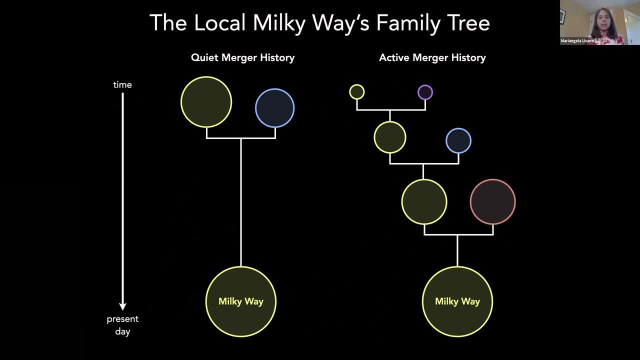 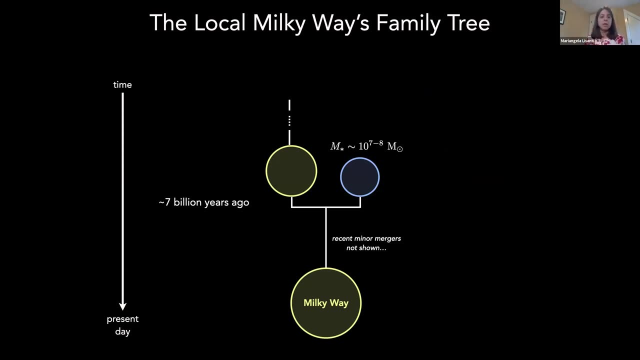 and pin things down a bit. So we had this, these two extremes that I presented, one that was really quiet, quiet merger history, another one that was very active merger history with the discovery of Gaia Enceladus. that actually sort of pins down some relative that we have. 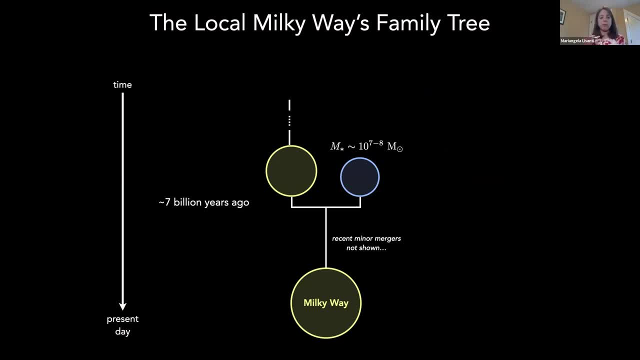 So we now know that there was a definitely a fairly significant merger. that happened early on in the Milky Way's evolution, so about 7 billion years ago, And the galaxy that collided with our own had a stellar mass of roughly 10 to the 7,. 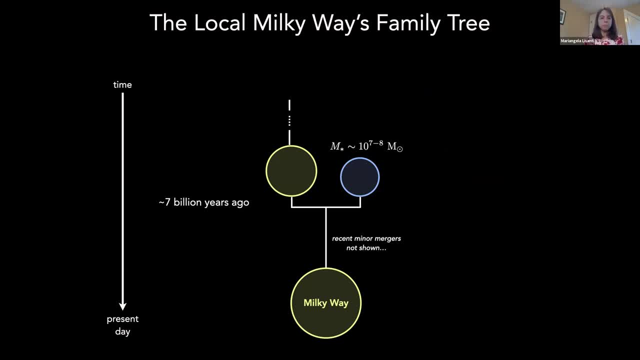 10 to the 8 solar masses at that point in time. So this is kind of like finding an old relative in your family tree. Gaia Enceladus is an old relative of ours in the Milky Way, and now we've been able to see. 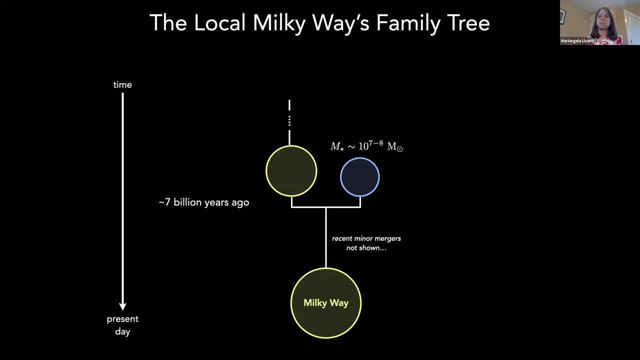 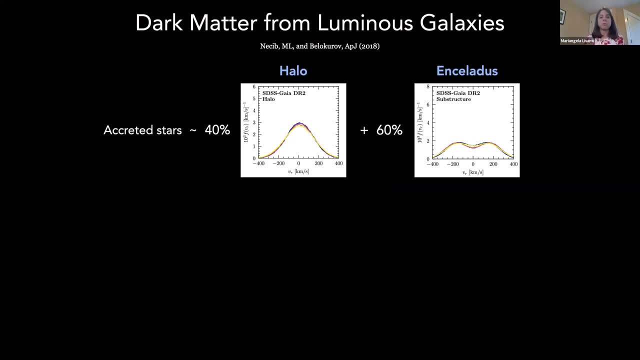 discover it, based off of the residue of the material that it essentially left behind. And the Gaussian mixture analysis that we performed lets us do a much a pretty careful accounting for how much material came in from Gaia Enceladus, and then also allows us to do a mapping from 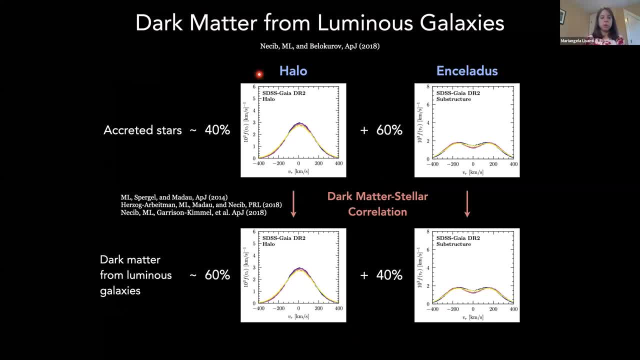 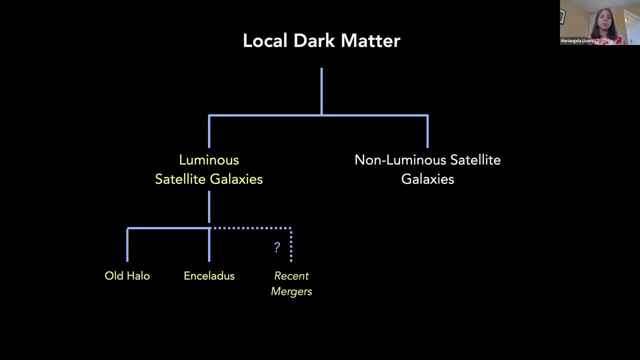 the material that we're seeing, from the stellar component to the fractions that we expect in the dark matter. So how much of the dark matter came in from the earliest mergers and how much would have also come in from Enceladus. So putting this back onto our little schematic diagram here, 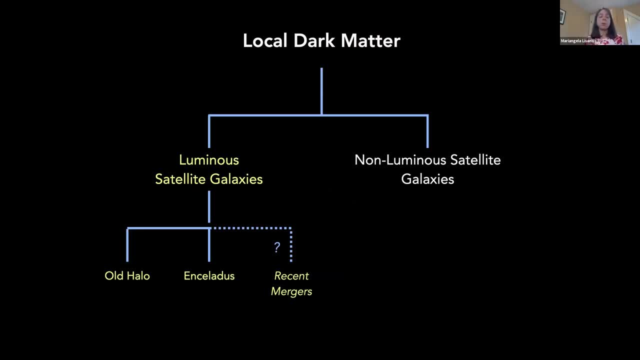 we see that even in this first attempt at looking at the Gaia data we've already made a pretty significant step forward in our understanding of how the local dark matter is distributed. We now know that it's not just dark matter from all very old mergers that we have that component. 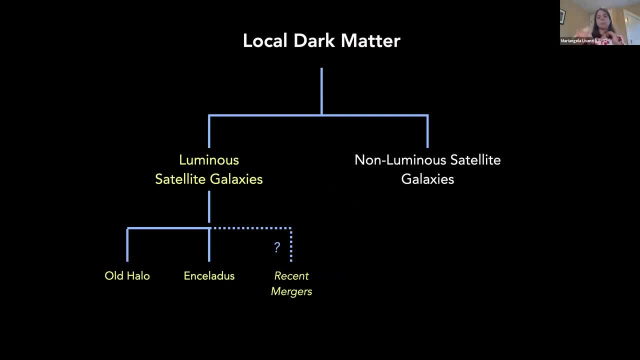 but we also have a component of the dark matter that's coming from this new relative, Gaia Enceladus, that came in about 7 billion years ago. So can we do even better than this? And the answer is yes, And the way we can push this forward is by taking advantage. 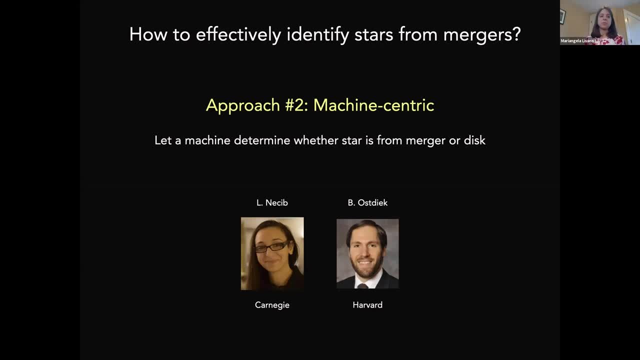 of some machine learning techniques. So this takes us to approach number two, which, in contrast to the first one, is more machine centric. This effort was led by both Lina as well as Brian Ostiak, who's a postdoc at Harvard. 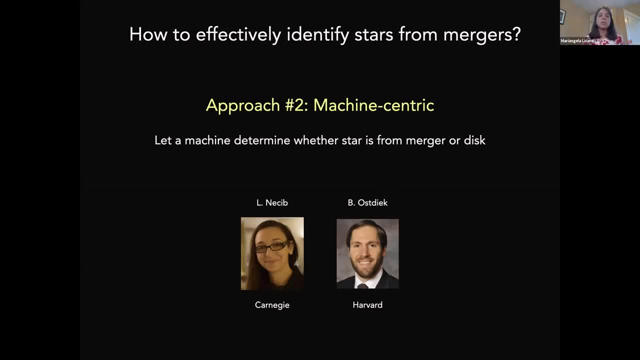 And the goal of of this part of the work was to see whether or not we can just let a machine determine whether or not a star is born in our galaxy or whether or not it comes from one of these satellite mergers, And if we're going to let the machine do this, 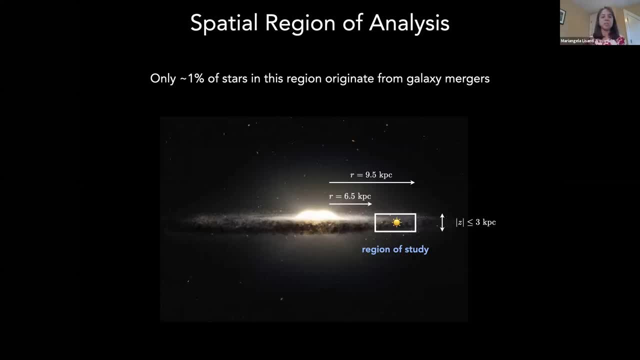 we might as well let it do it in the region where it's going to be hardest to try, but also the region where it's going to be of most interest. So what we're going to do now is apply this neural net that we're going to develop. 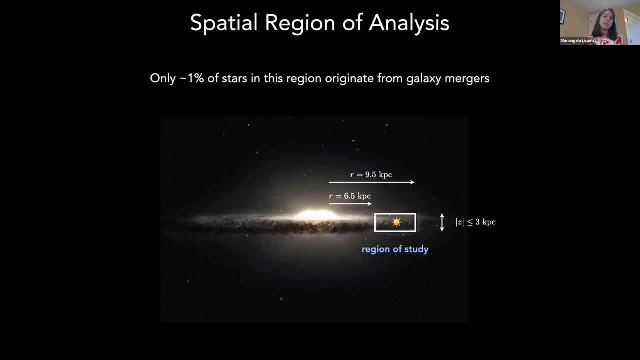 in this area that's concentrated right in the disc plane, So precisely the region we were trying to avoid before, because we know that there's going to be a lot of disc contamination there, And but it's also the region that's of most interest. 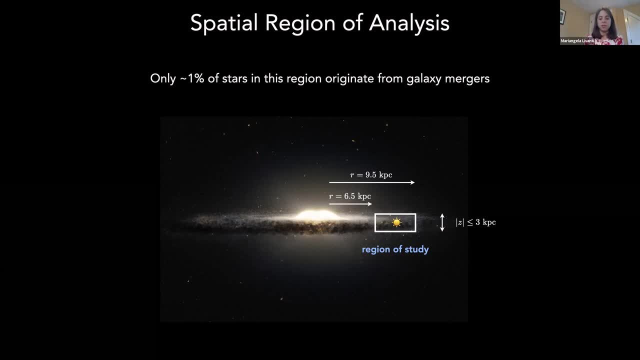 for any dark matter direct detection experiment, because we want to have the dark matter mapping close to where we are, So near near where the sun is. The challenge here is that only about 1% of the stars in this region that I'm boxing in here. 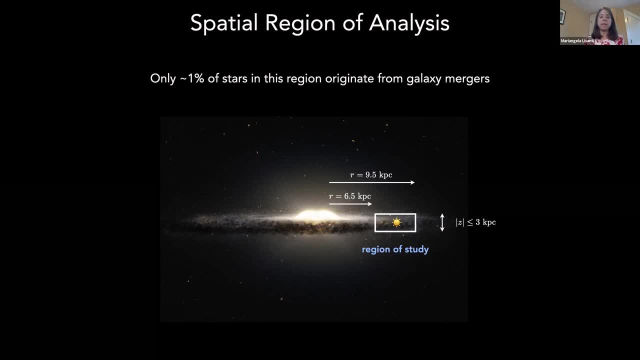 are coming from these galaxy mergers. The other 99% are what we'll consider to be background. So the background here are just the stars in the disc, the stars that were born in the Milky Way galaxy. So that's the challenge that we're essentially putting forward to the machine. 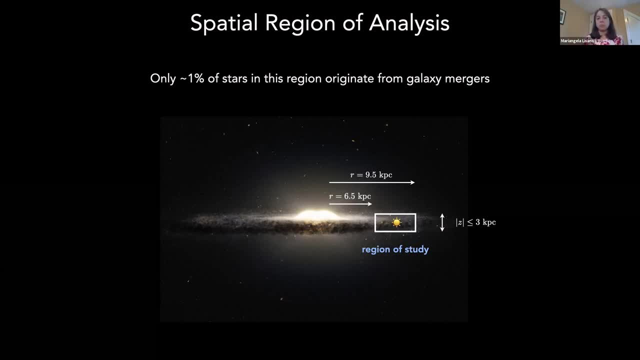 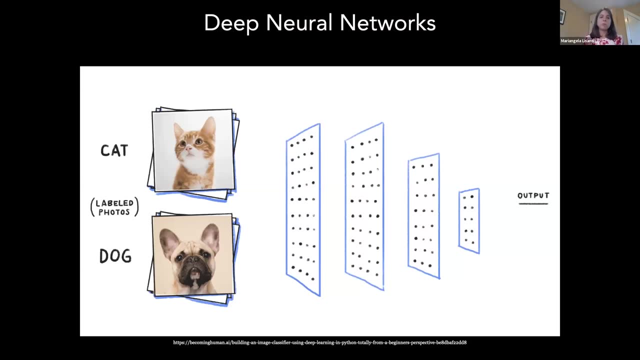 Can you accurately identify the 1% of stars in this region that came from these, these mergers? So we're going to use deep neural networks to do this. In this kind of approach, you train the network on labeled photos. So in this cartoon, 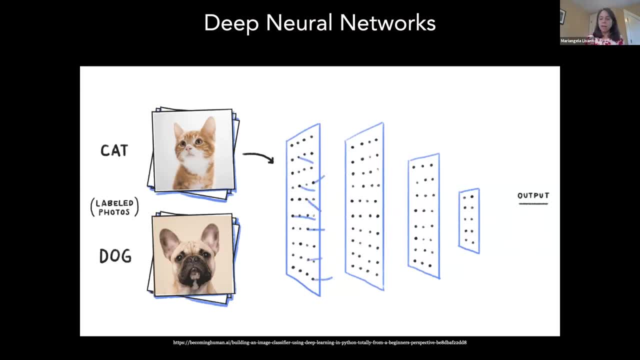 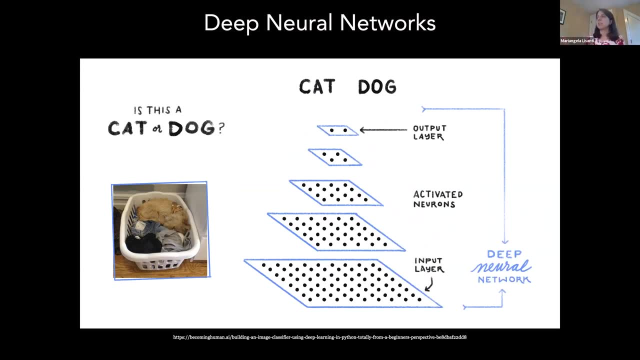 it's being trained on images of a cat and a dog And then afterwards, after that training period, you then test, you can apply your network to an arbitrary photo, So in this, this image of a creature inside this laundry basket. and then, based off of what the network learned from the training, 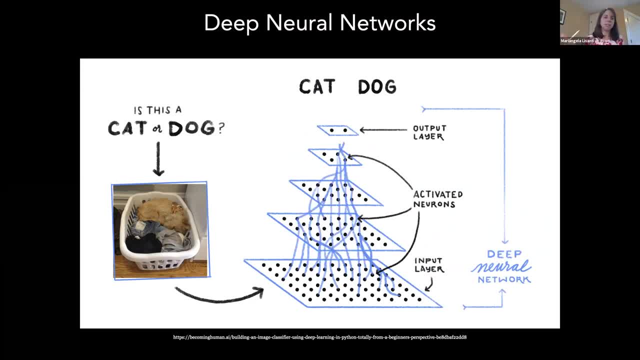 it then decides and guesses whether or not that creature is a cat or a dog. Now, obviously, what we're dealing with are not pictures of cats and dogs. What we're dealing with is data concerning stars that are either born in the galaxy or not born in the galaxy. 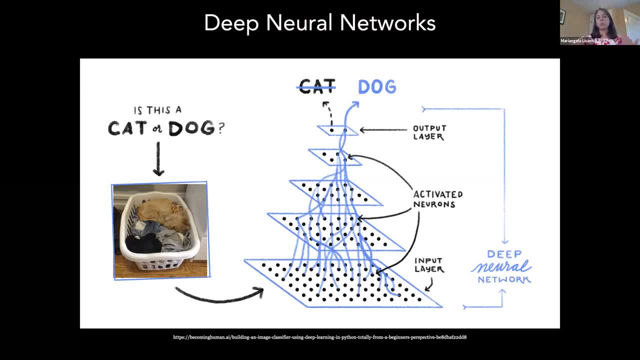 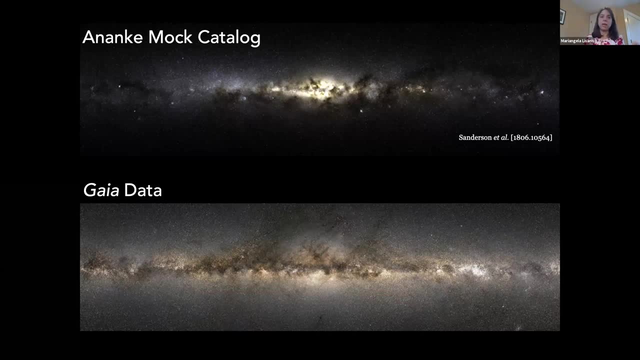 But the approach we're going to take is going to be kind of similar, in the sense that we're going to train our neural network on simulations where we know what the truth is, So where we can label each star with whether or not it's a galaxy star or a merger star. 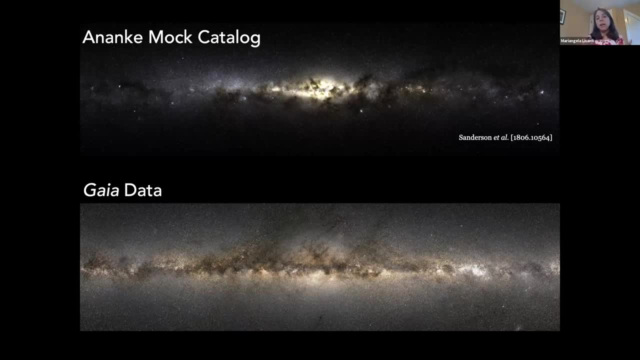 And then, after training the network on these simulations, then we can apply it to data from Gaia and see what it gives us. The only way that this can work is if the simulations that you're training the network on are doing a good job at reproducing what's in our galaxy. 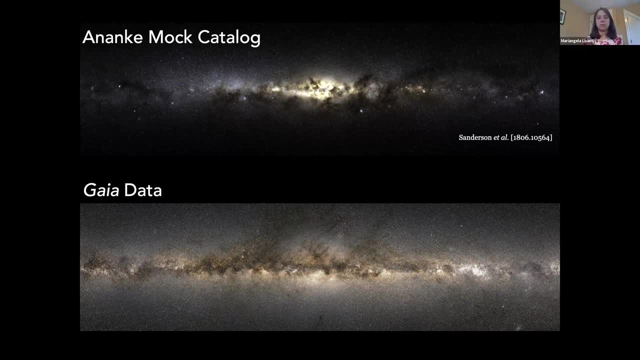 And if we were doing this 10 years ago, there would have been no way that this would have even had any shot at working, because the simulations were just not at that stage. When people were first starting to run these galaxy formation simulations, they couldn't even get stable disks to form. 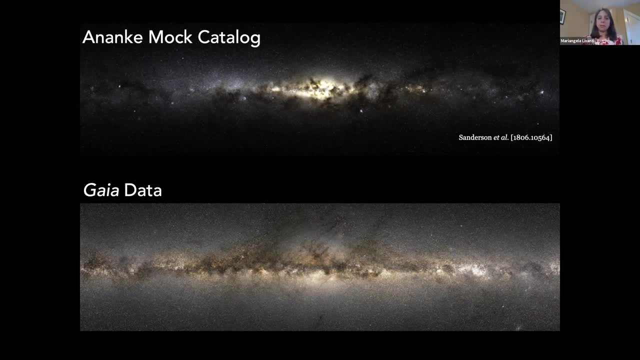 And it's just been incredible the level of progress that has happened to get us to where we are today. So what I'm showing here in the top panel is a simulation results from one of these simulations, So it's a mock catalog, referred to as the Ananka mock catalog. 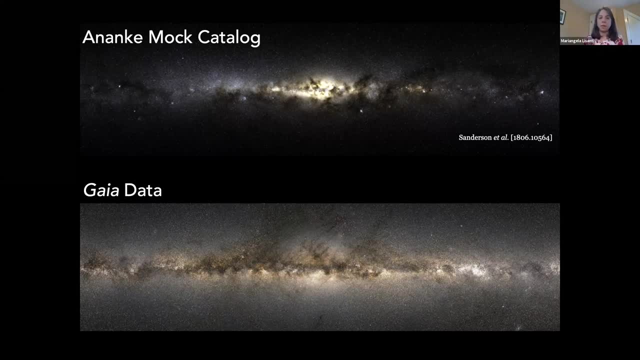 And just for comparison. below it I'm putting the data from Gaia And you can see by eye that there's a lot of features that are reproduced in the mock data. It's not a perfect correspondence and we don't expect it to be a perfect correspondence. 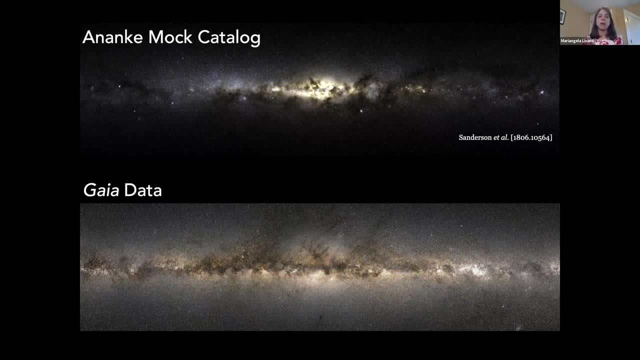 but it's roughly getting the general behavior correct, And that at least gives us a hope that this approach has a shot at being able to work. I'm seeing that there's a question, So maybe I can pause. Juven, Yes, Can you hear me? 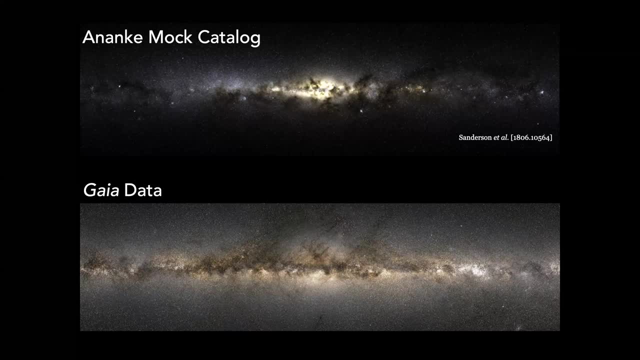 Yes, I can hear you. I was going to ask earlier. Earlier, you said that 1% of the star is from the merger star. Well, 99% is galaxy star. Is that correct? I just wonder how the data is obtained. 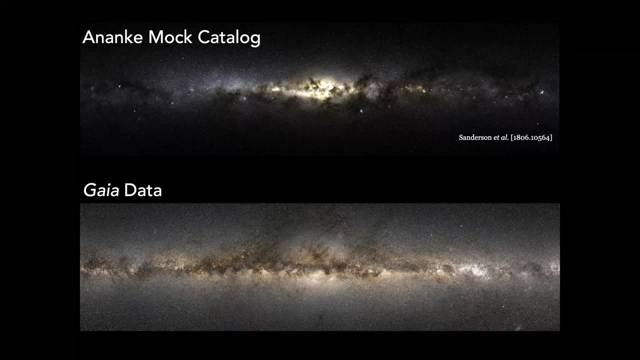 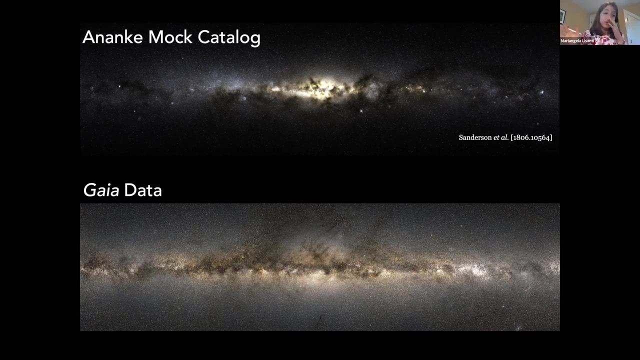 How do you know this? This 1%, how is that determined? Yeah, that's a good question. Yeah, so that's determined. If you have a, I'm sorry, let me take a step back. So the Gaia data itself is huge. 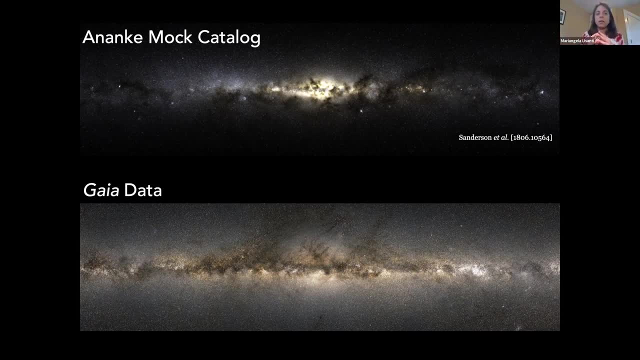 So it's about a billion stars, but only a small fraction of that actually has are stars that have- let's call it- a more complete amount of information. So if you have stars that have really good kinematic observations coupled with really good chemical abundance, 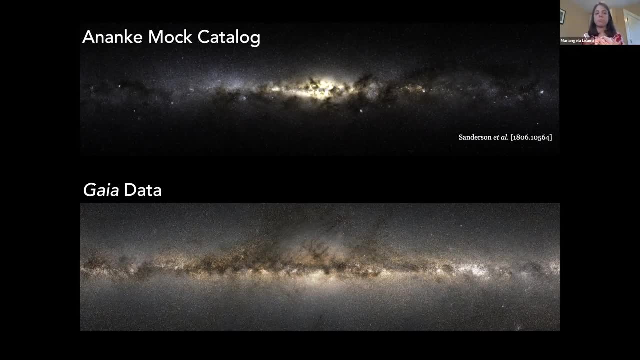 information. so you also need some information about just their chemical properties. If you have that, then you have an ability to be able to determine, a much better ability at being able to determine whether or not the stars belong in the disk or whether or not. 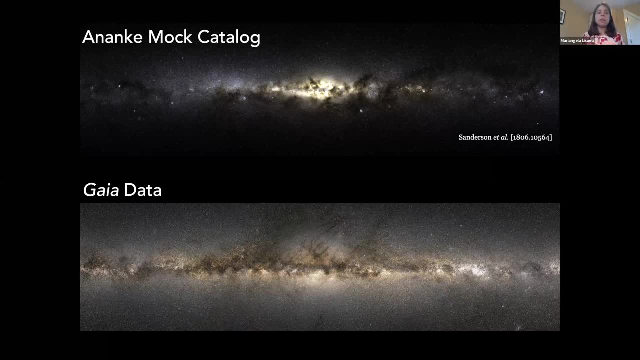 they came from the merger. So you can't infer that 1% from the entirety of the Gaia data. but what you can do is look at the small subset that's particularly clean and where you have this additional information, this additional spectroscopic. 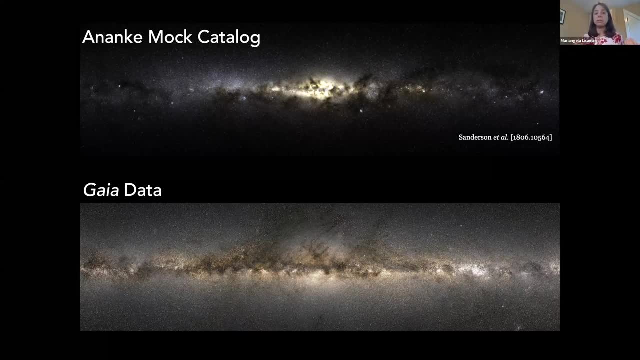 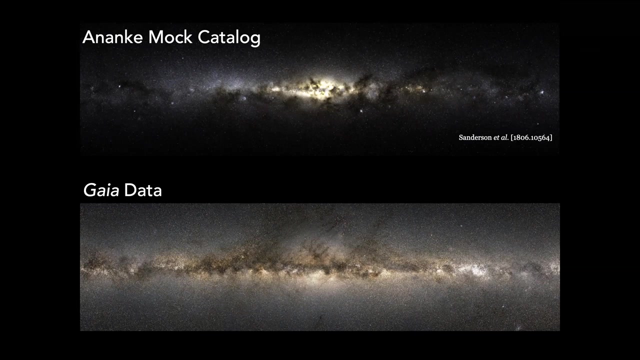 This additional spectroscopic information that has the chemical abundances And then, based off of that sort of smaller, very clean and pure data set, you can estimate what the fraction should be. Okay, Does that answer your question? Yes, but there seems to be something. 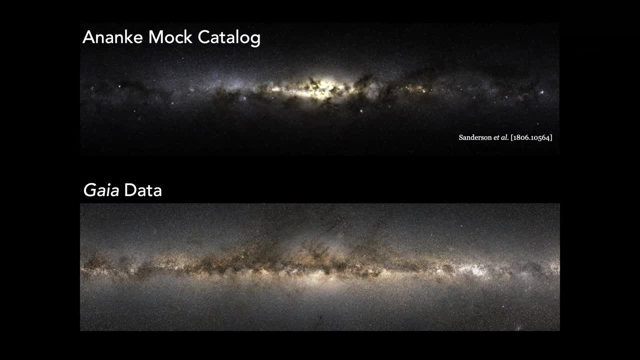 Let me see. It seems like earlier you said perhaps there's 1%. so the data is rare, so there could be some difficulty to spot them. I'm just trying to understand the logic. Do we have 1% first? so the data is hard to collect. 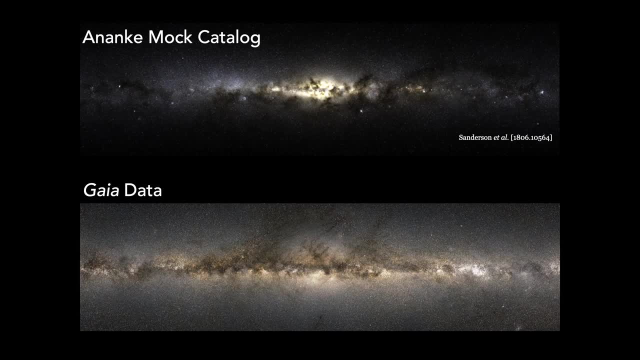 or is that we collect data and we find out it's 1%? Maybe just the logic between which one we know first. So we estimate that 1% first from much smaller, much smaller data sets. So there's other, and before Gaia: 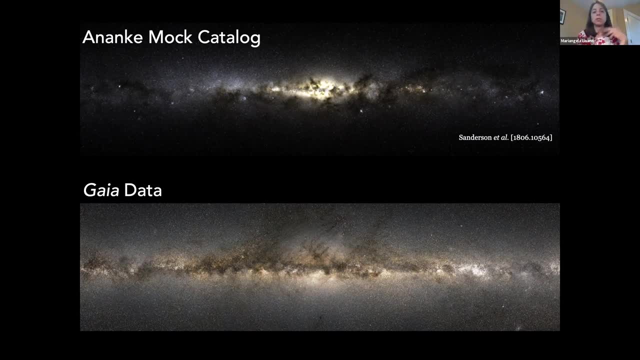 there were also. there's other sort of spectroscopic surveys like Sloan et cetera, that have a much. they're looking at a much, much smaller number of stars overall, but the stars that they do look at they have more information about. 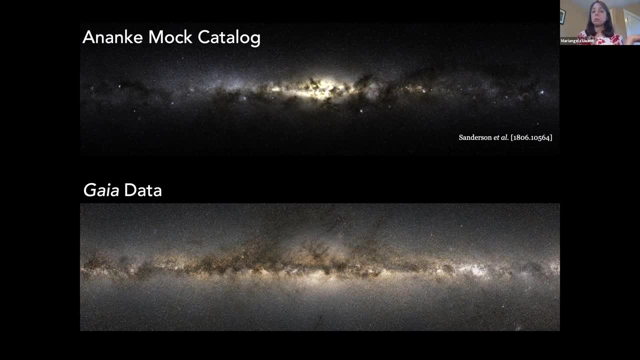 And so, based off of studies that were done with these earlier surveys, like Sloan, we can estimate that only about 1% of the stars in the disk are coming from the mergers. But that's it's a rough estimate from these smaller data sets. 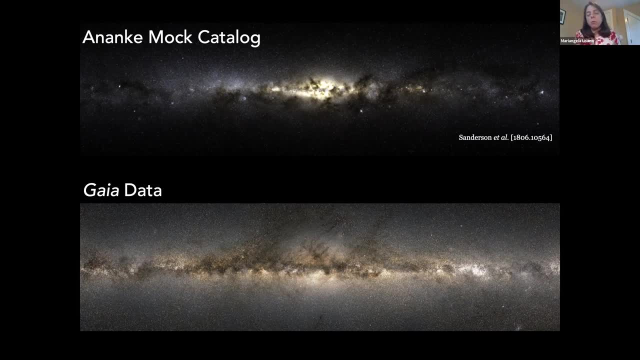 And so what we- I mean what the process that I'm about to explain to you- is actually going to be a much better. I mean, this is how we can actually get that new fraction from the Gaia data. Okay, thank you. 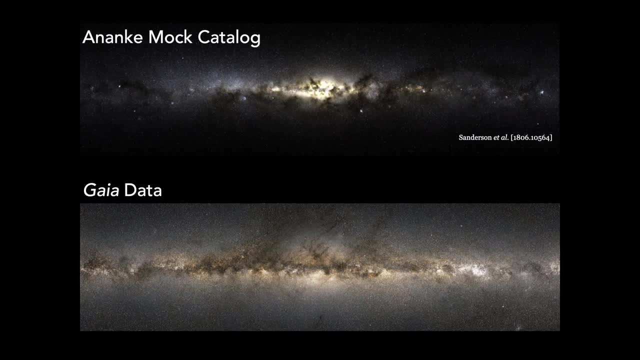 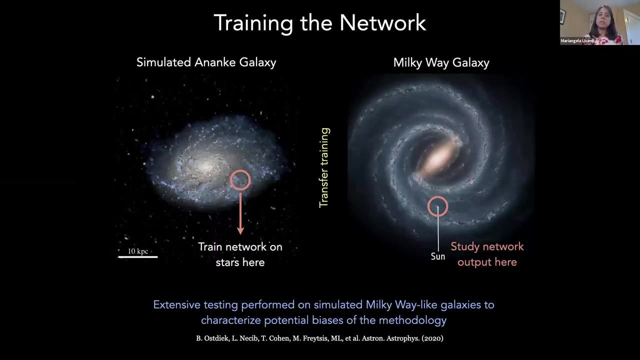 Yeah, Okay. so what I'm showing you here is essentially the. the top is the simulation that we're going to use to train the network and the bottom is the data, The. I won't have time to go into the details of the network configuration, but just very broadly. 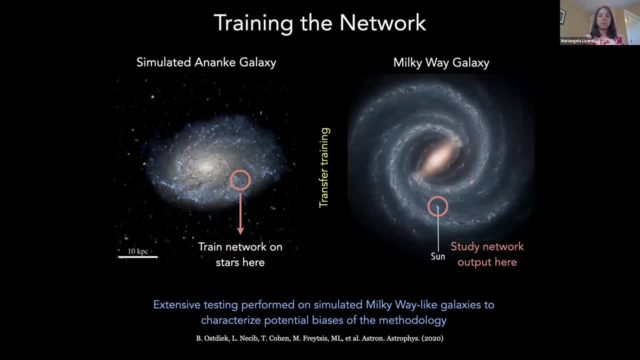 what we do is we train the network on one of these simulated galaxies. Then we apply a transfer training step where the last layer of the network is retrained on some small subset of data from the Milky Way galaxy, where we have high confidence that there are stars that would have come from these mergers. 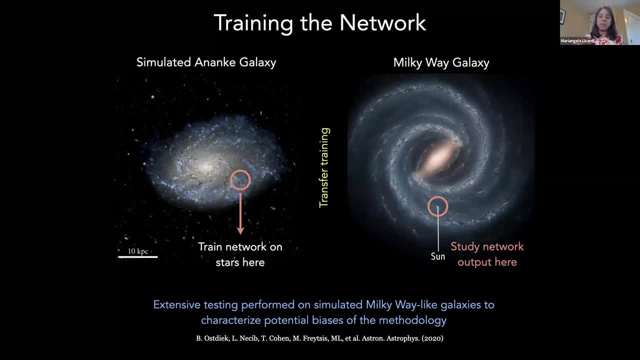 And then we apply the network to all of the data in the Gaia catalog. Now there's obviously a lot of concerns that arise when you are using or training a machine learning algorithm on a simulation and then applying it to actual data. One big concern is what happens if the network 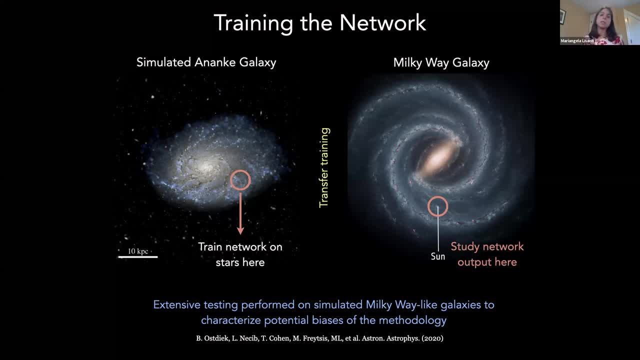 is learning something specific about the simulated galaxy that actually is not consistent with our own galaxy. We performed an extensive amount of testing on these simulated galaxies to better understand the biases that come from applying this network training, And I'd be happy to discuss more of this afterwards. 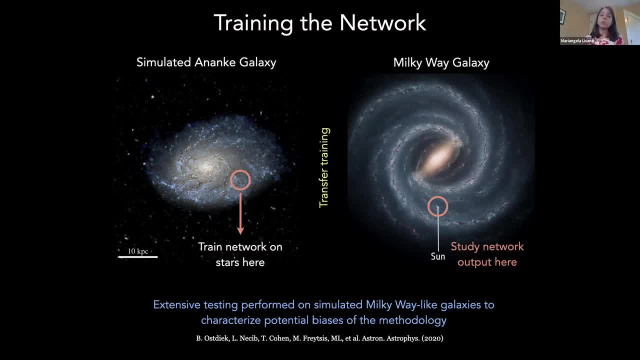 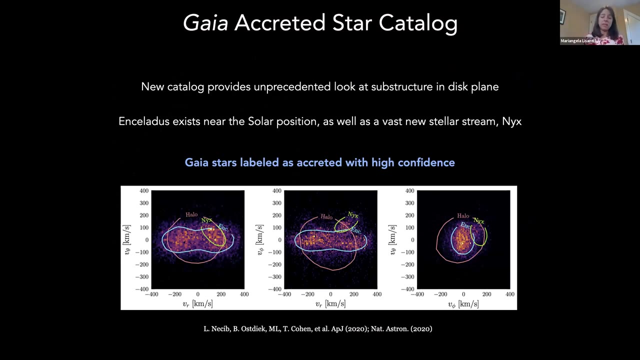 if there's any questions. But for now let me just show you the results of what we get after applying the neural network to the Gaia data. So the network output, essentially, is going to tell us the stars that have the highest probability of coming from one of these mergers. 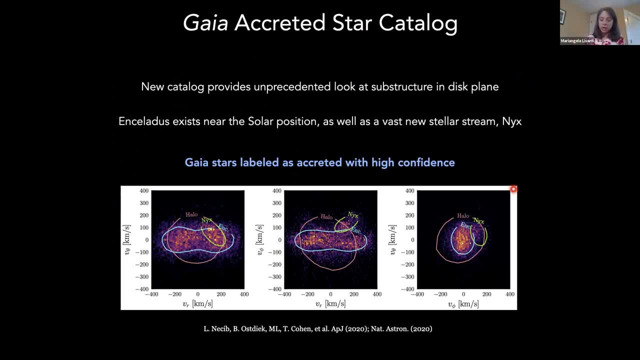 And what I'm plotting here in this panel are essentially distributions of those stars where the network is most confident of their origin, And I'm making these plots on different projections in velocity space. Based off of that network output, we again perform another mixture model analysis. 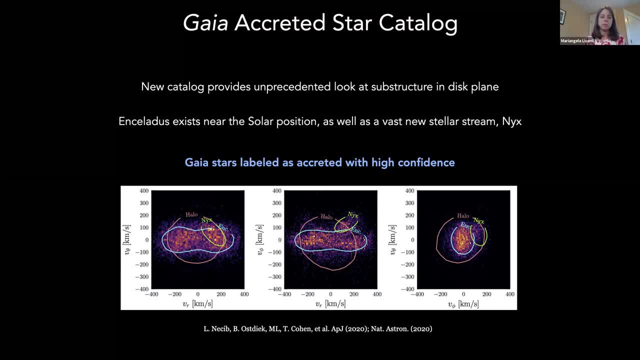 to see how many different components seem to exist in that data. And here we're finding three components. So the pink here is the part that's mostly isotropic in velocity. Those are the stars we think are coming in from the very, very old mergers. 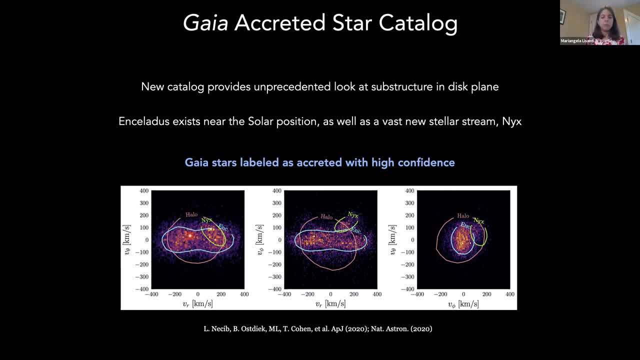 The blue thing that looks a bit like a peanut here, that's the kinematic distributions of this blue component here actually match the expectation for Enceladus, so our new relative that we discussed earlier. So what this shows us actually quite explicitly. 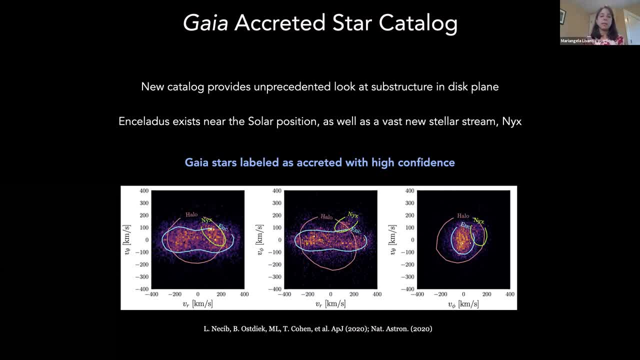 is that material from that Enceladus galaxy has actually landed close to where the Sun is, So we do expect that dark matter from the Enceladus galaxy should be present near the Earth. In addition, however, the clustering algorithm finds one additional component, which is circled in green. 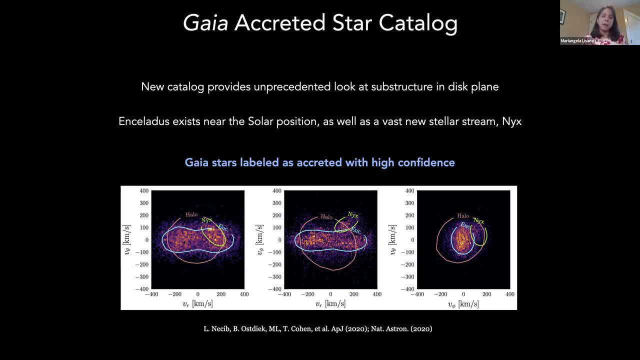 And that's what we're calling nix. Nix is mu. We didn't see it earlier And we need to try to understand what it is. It's not a few stars, So it's about several hundred stars all kind of clustered together here. 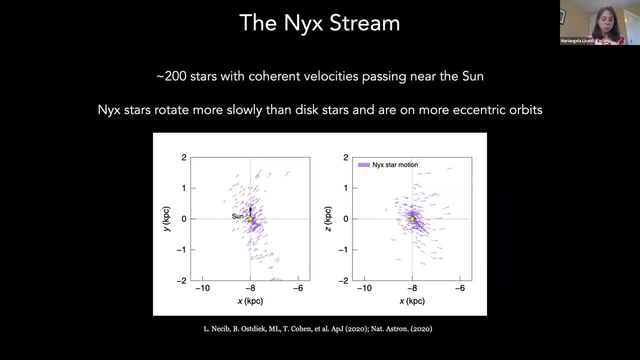 This is what the stars look like. This is how they're moving around where the Sun is. So if the Sun is located here and moving this way, these nix stars are kind of moving diagonal relative to that position. You can see that their motion is pretty coherent. 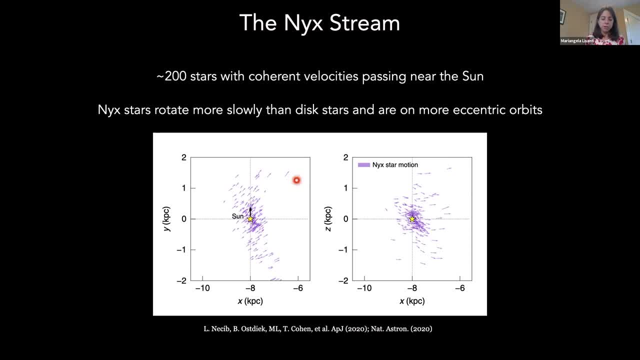 All of the stars, the arrows here are all pointing roughly in this direction here. So we have this large cluster of stars, like 200 stars. They're moving with these coherent velocities past where the Sun's location is And their velocities are extremely. 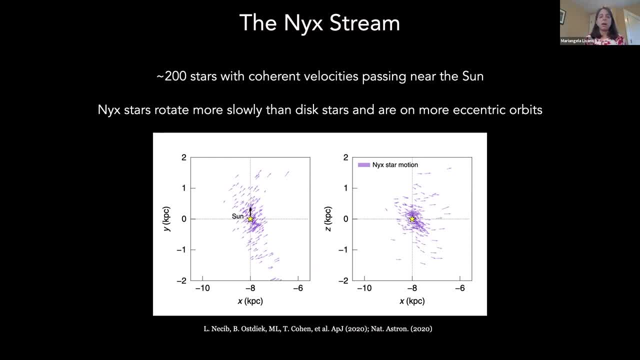 they're very eccentric. So the stars are on very eccentric orbits And the kinematics of this is hard to explain unless the stars came from a separate merger. It could be that this is a stream of stars that's associated with some perturbation of the Milky Way disk. 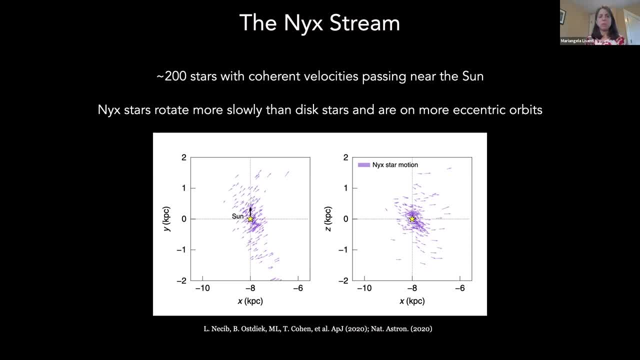 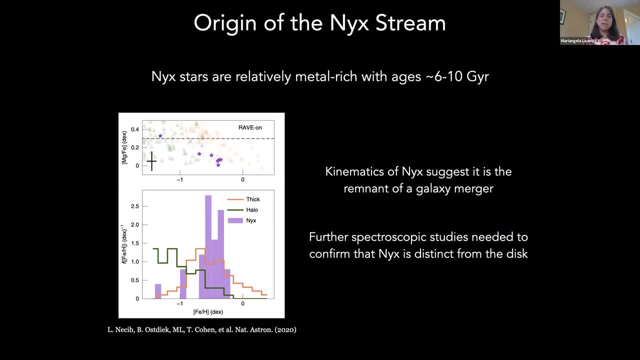 But it's a lot harder to be able to explain their kinematic distributions that way. So nix might end up being one of the largest streams discovered that's passing through the Sun, And because it's so large we really need to understand exactly. 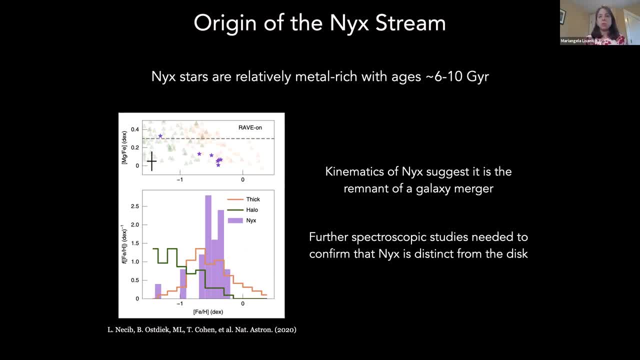 what its origin is. In order to do this, we're going to need to use need to do some follow-up spectroscopic studies that will allow us to get better chemical abundance information about the stars That will help us differentiate them from the disk more effectively. 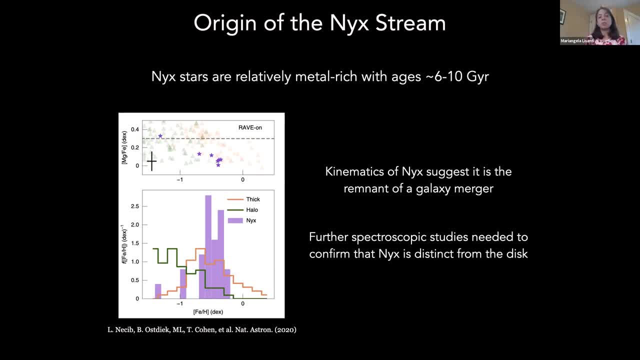 We can also get better measurements of the ages of the stars, which would also provide an important probe in understanding whether or not they came from these mergers. So these follow-up observational studies are all in the works to improve both the chemical abundance information we have for the stars and also their ages. 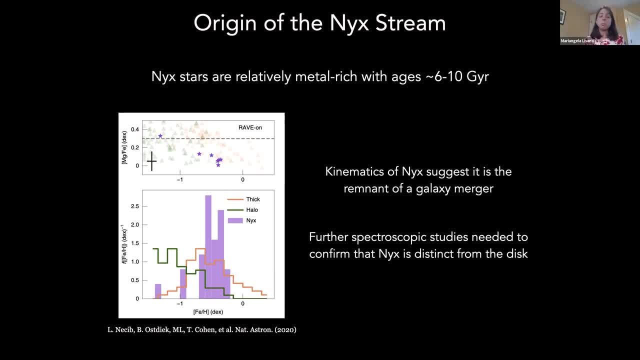 And, as I said, both of those things taken together will really help to clarify the picture of where the origin for this new, extremely extensive stream that's passing by the solar position. The ramifications of this are significant because we know from simulations that streams like nix 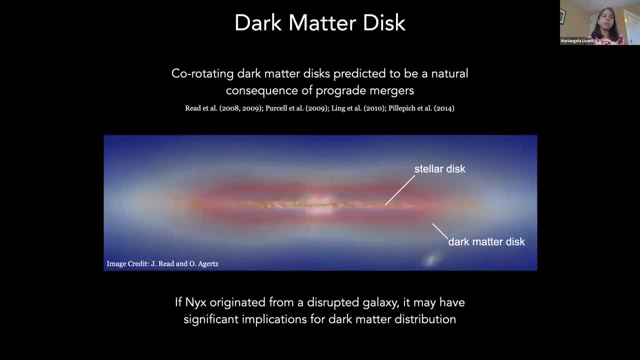 if they're formed from some of these mergers would actually be an indication that there is a rotating disk of dark matter in the Milky Way galaxy. So there were some initial theory works on this from about a decade ago showing that for certain types of mergers, 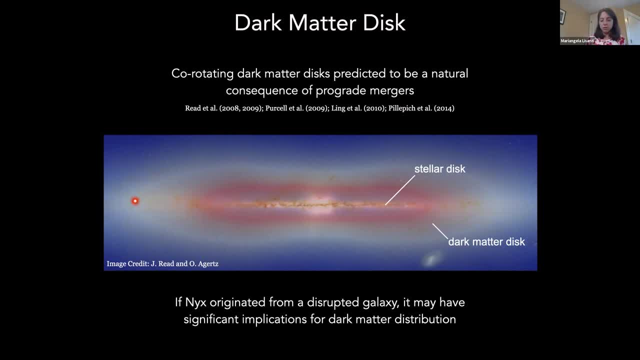 you'd expect there to be this kind of fluffy dark matter disk that forms surrounding our stellar disk. This is a pretty dramatic change from the picture I showed you very early on, where we think about the dark matter distribution as just being a single halo. Now, if this is correct, 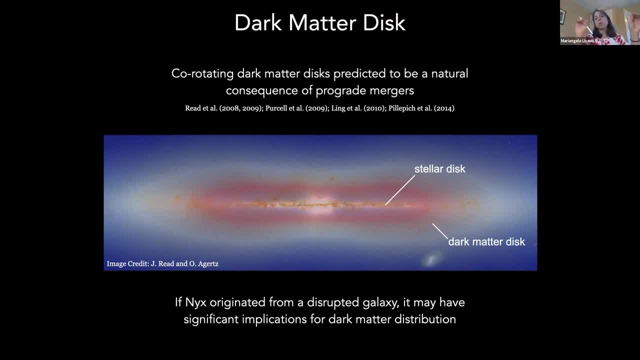 we have this picture of a halo in addition to a disk component that's kind of rotating along with the stellar disk in the Milky Way And then, of course, where our experiments would be running, we'd be sitting right in the middle of this dark matter disk. 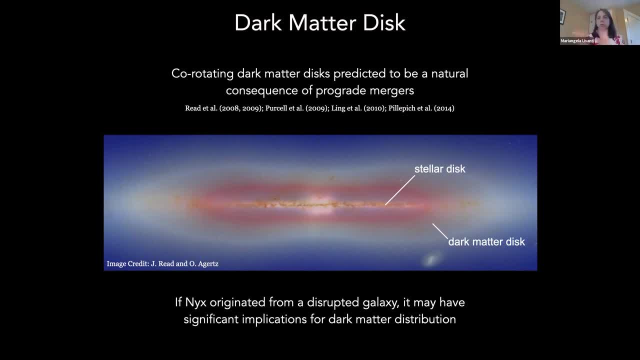 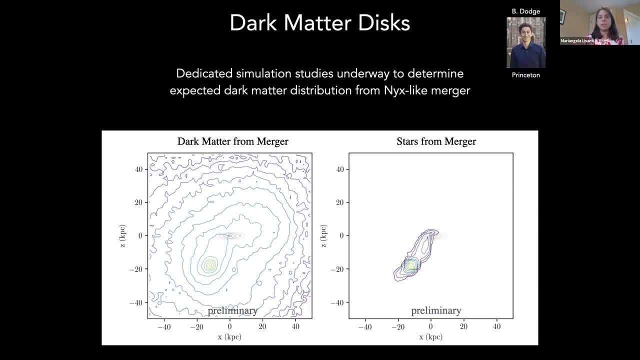 surrounded by this material that's kind of this dark matter material that's rotating around in the galaxy. So one of the things that we're trying to understand now- this is actually work that's being led by an undergraduate here at Princeton- is how do these dark matter disks form? 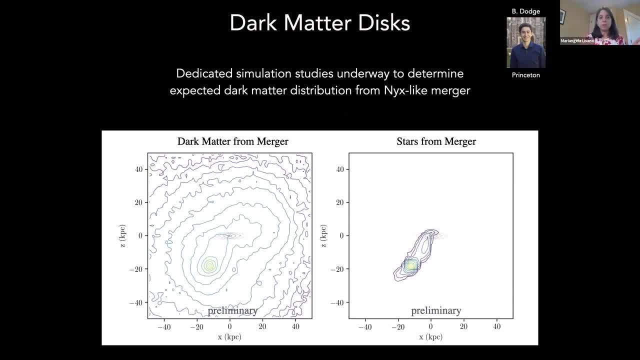 And are the formation. when these disks do form, do we end up getting things that look like nicks that get left behind? This work will allow us to actually be able to say much more specifically what the associated dark matter distribution that you would expect from a merger that's like nicks. 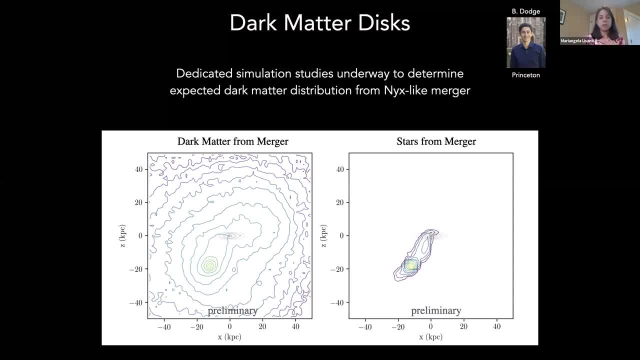 So this is just very preliminary results from the initial simulations that Ben has been running. The little regions here, the gray regions, show the Milky Way disk. On the left panel shows dark matter from one satellite galaxy as it's falling in, And on the right are the stars. 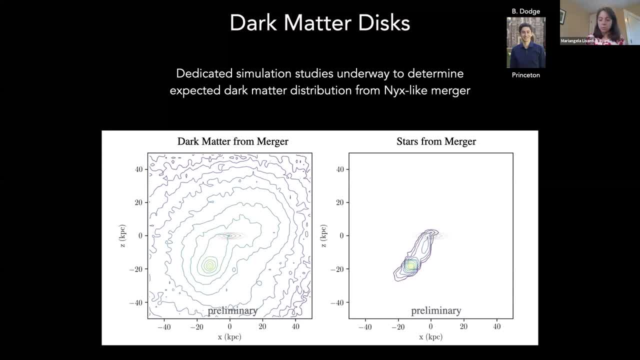 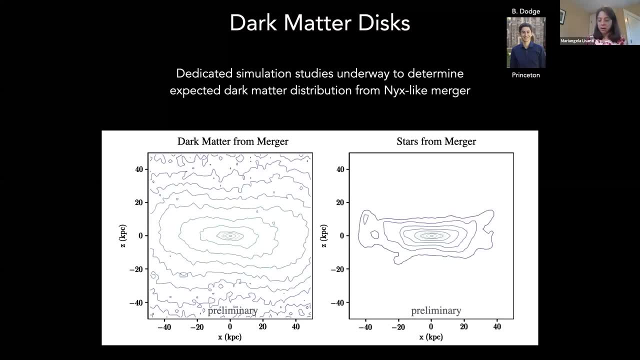 from that satellite galaxy And as time progresses you can see the satellite gets totally disrupted And what it ultimately ends up leaving behind are stars that are kind of concentrated near where the stellar disk is, and then also this dark matter disk here on the left panel. 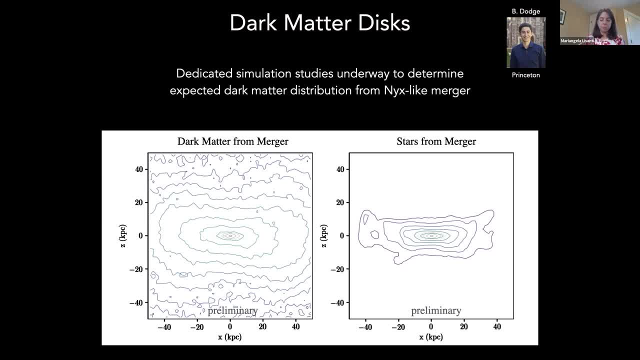 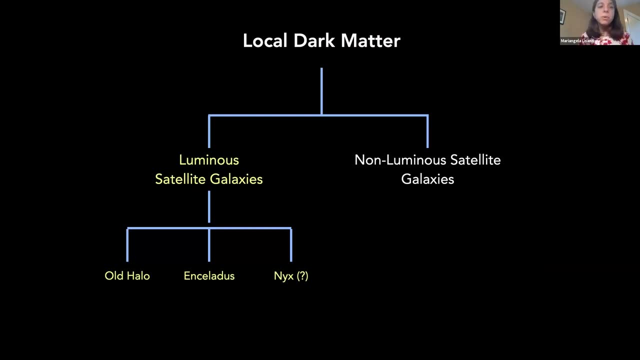 And what this doesn't, these particular plots don't show, is that both the stars and also the dark matter in this disk are essentially rotating around. So that takes us essentially to the conclusions. This is about as far as we've gotten. We've been able to harness this data. 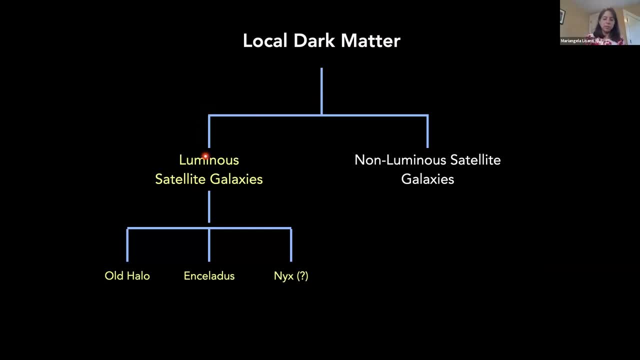 from Gaia to fill in the branch of this, this diagram here, where we're mapping out the dark matter that came from these galaxies that hosted stars, And by digging deep into this extremely large data set, what we're finding is that the dark matter 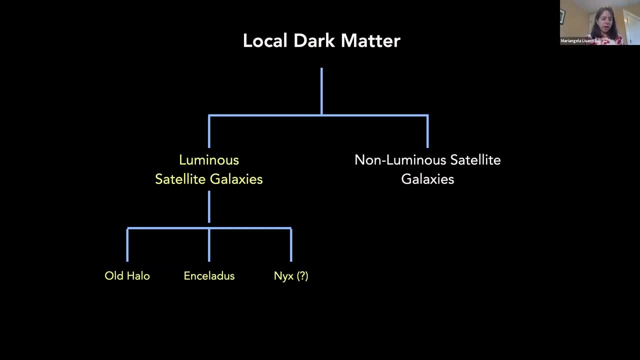 near the solar position has three, what appears to be three- contributions. So it has a component that came in very, very early on, so from the oldest mergers. It has a component that came in from our new Milky Way relative called Enceladus. 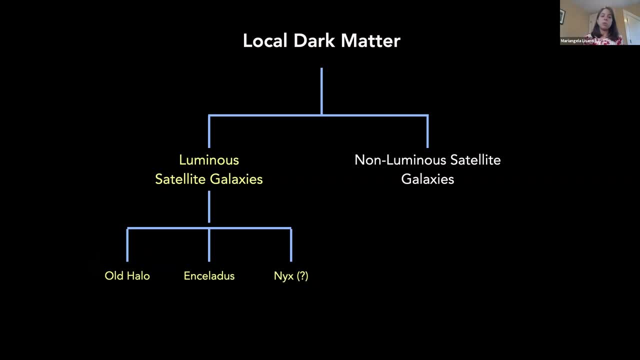 And then it may also have this additional component that came in from this Nix merger- And I've left a question mark here because this is pending confirmation from these additional spectroscopic studies that are currently being done. So we've made a lot of progress. 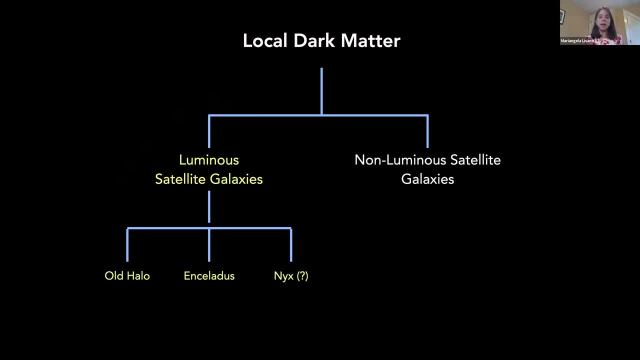 in this direction. To really complete the mapping, we're going to need to start facing this arm of the diagram here which we haven't quite tackled yet, but we have some ideas for how to start doing that And then, taken together 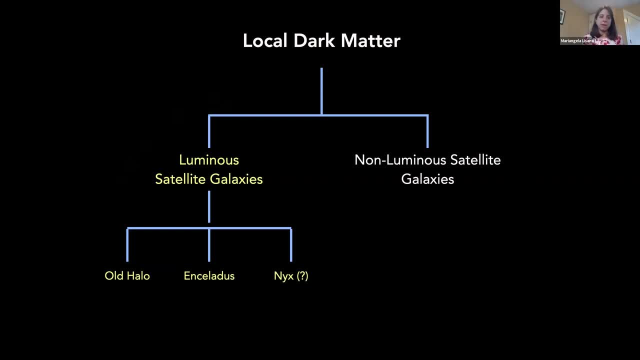 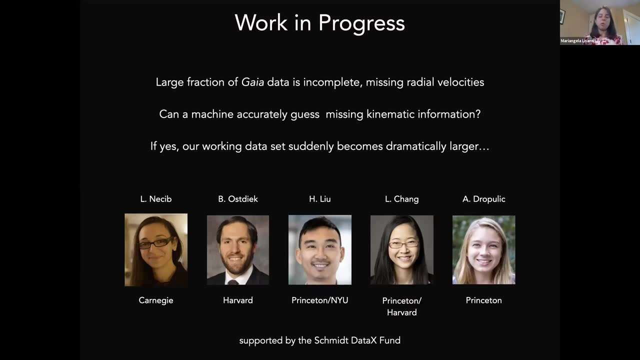 then that will give us our complete mapping. We're also pushing forward on trying to further develop a lot of these machine learning techniques. One particular direction that I'm really excited by is the following: We have this team here with Lena, Brian, and then postdocs. 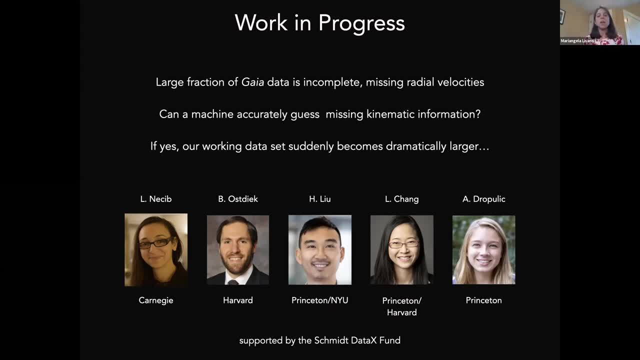 and graduate students at Princeton who are all working on this. What we're asking is whether or not a machine can fill in some missing information in the Gaia data. So the large fraction of the Gaia data is incomplete and, in particular, is missing. 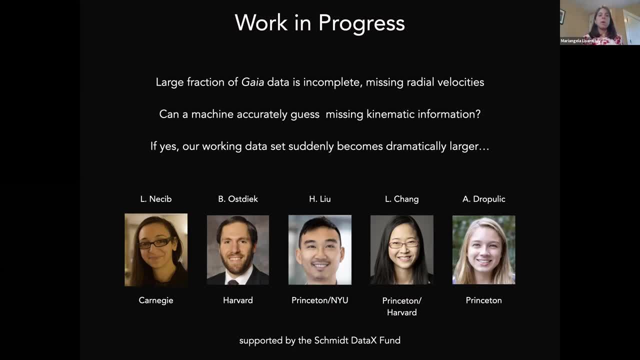 the radial velocities for the stars, And what we want to know is whether or not a machine can actually accurately guess those velocities and provide us with its level of confidence in its guess. If we can do that, then our working data set will suddenly become significant. 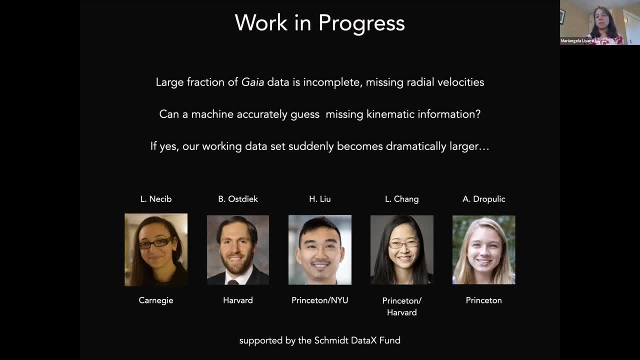 larger and we can essentially repeat the type of work I've described to you today with this larger data set. So that will improve the number of candidate stars we'd get for Nix, but also allow us to see if there's any additional structures. 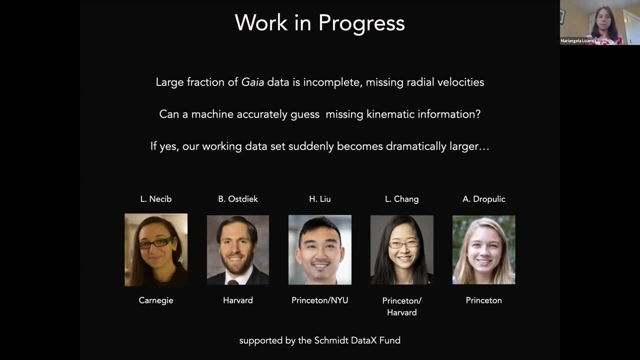 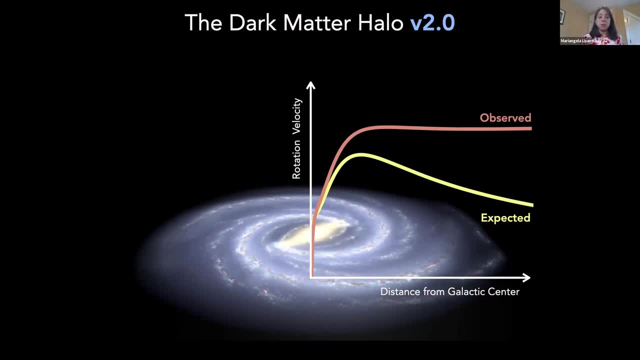 that are there beyond, for example, Nix and Enceladus. Okay, so let me just conclude by going back to where we started. So, as I began this talk discussing flat rotation curves in the Milky Way and how that initial discovery 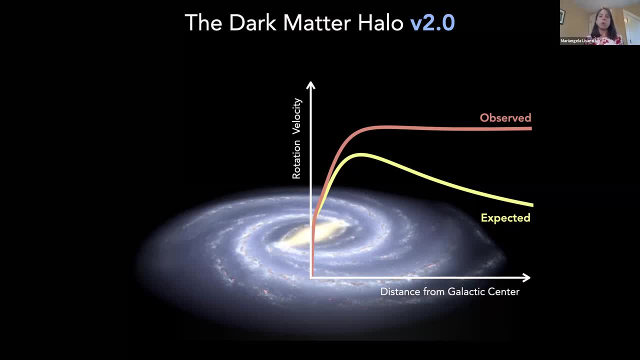 in the 1970s and early 1980s prompted the first models for how the dark matter is distributed in the halo, And the picture that came out of that initial work was a fairly simple model for that dark matter distribution. We assume that everything. 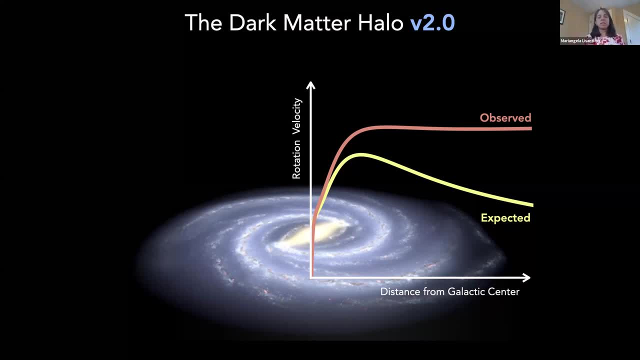 is in steady state, So it's a very- it's essentially just a one component model for that dark matter halo. Fortunately, with new data, it allows us to go back and revisit these models and to see what more might exist. And, as usually happens, 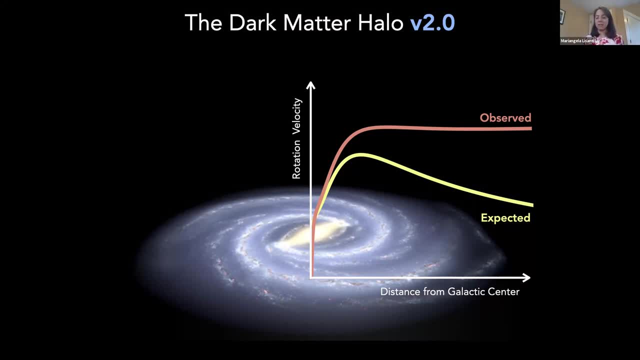 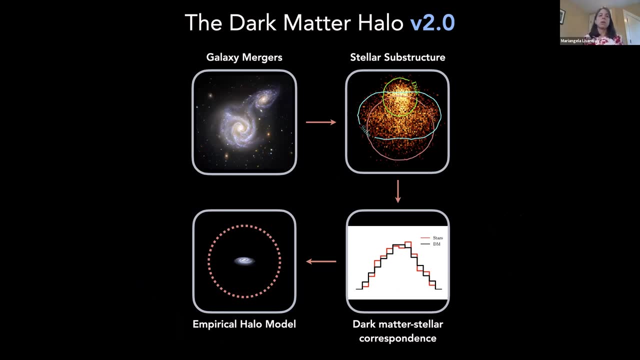 when you have more data, you end up finding some new and unexpected things. So by digging deep into the Gaia data, we've been able to get information about galaxy mergers that built up the Milky Way galaxies. We've done that looking at substructure. 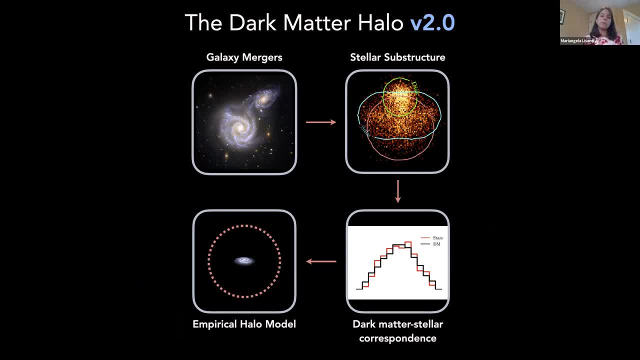 in stellar distributions and then, based off of theory work, looking at simulations and how dark matter is correlated with stars from these mergers, we could then end up mapping all of this into a halo model for the dark matter. We still have a lot of work to do. 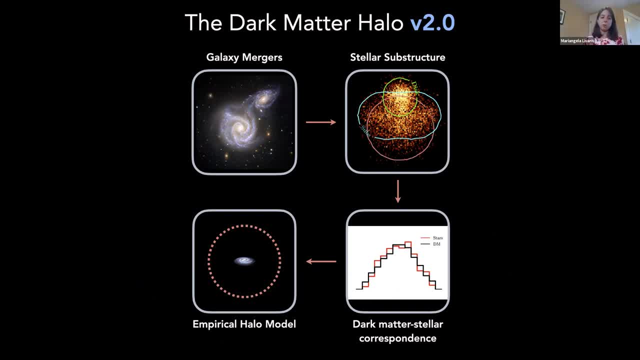 in understanding the components that are going into this empirical halo model. but we've been able to make a lot of progress so far with the data at hand, So I'm quite optimistic about what we'll be able to do in the coming years. So with that I'll conclude. 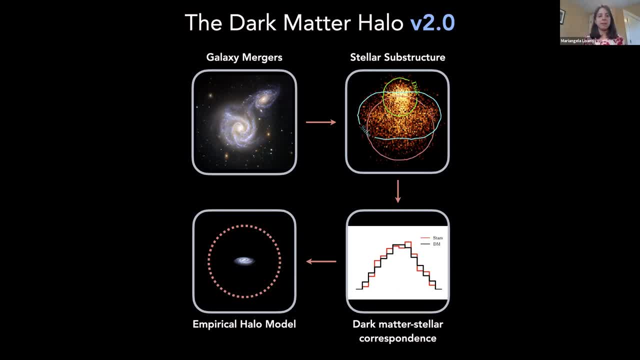 and I'm happy to take any questions that might arise. Thank you very much, Angela. If you have questions, please just unmute yourself. You can go ahead. Yes, thank you. Thank you for the wonderful talk. beautiful talk. There's a data. 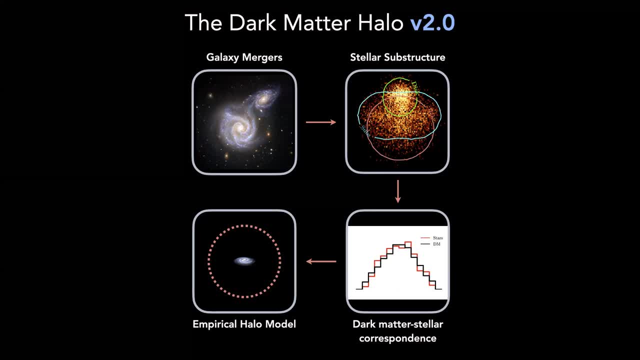 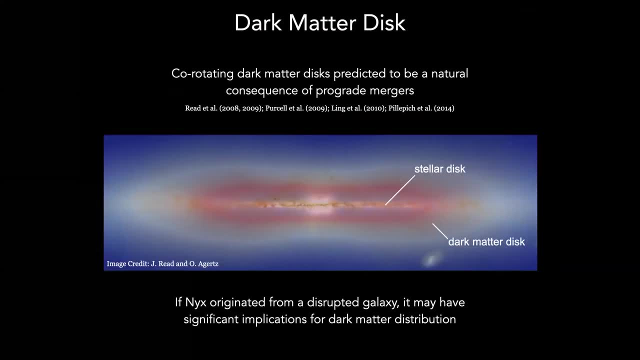 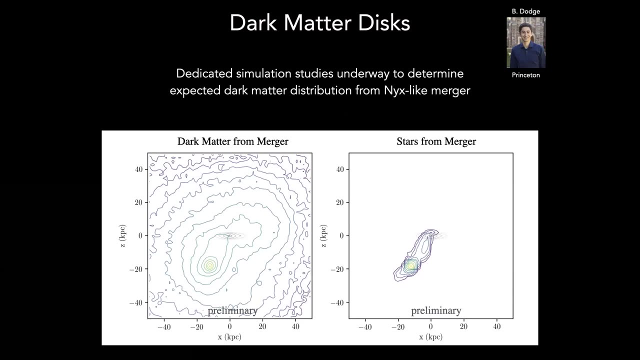 I think you show done with Princeton undergrad about the dark matter disk? I think there's. So the key message is that the stars from the merger will be localized in some region, while the dark matter from the merger will be spread around but still has some core on the stars. 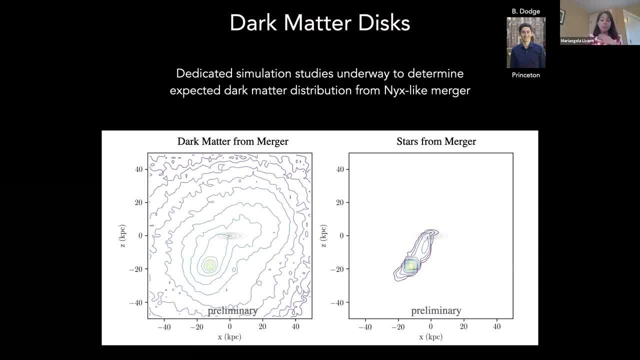 Is that the message you want to convey here? Yeah, that's right. So in general, the dark matter distribution will be a bit more spread out than the stellar distribution of the stuff that gets removed, And so here I'll just run through this. 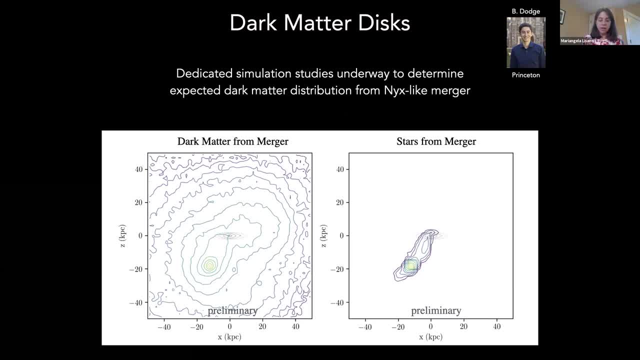 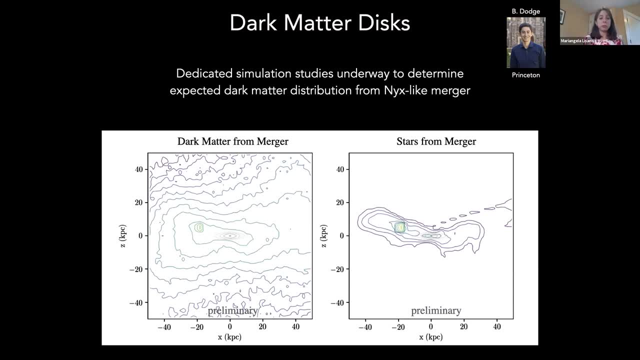 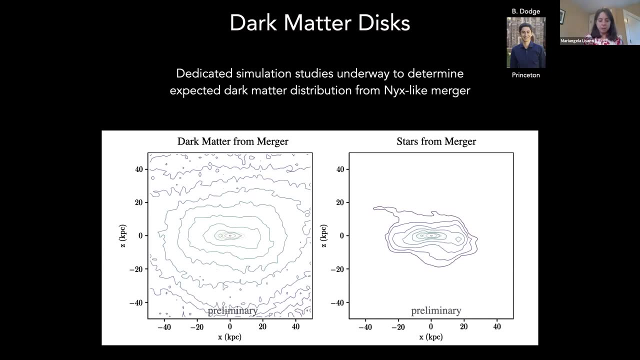 these clips again, so kind of pushing forward in time, And you can see in each of these time steps the dark matter distribution is more extensive than the stellar distribution but does track the central regions where the stars are concentrated, And then here at the end. 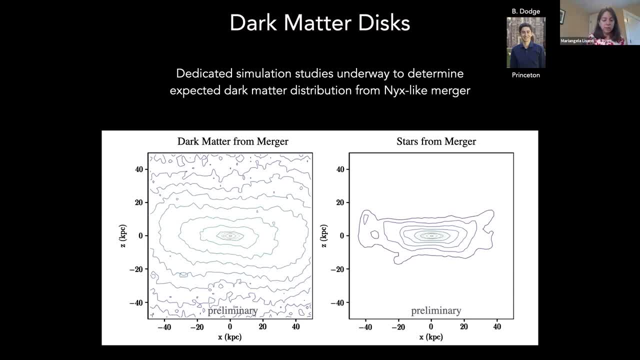 so that is what we're left with And for sure like there's definitely the dark matter, distribution is broader, but again, it's concentrated Roughly where the stars are here. So the stars are, I mean, they're not a perfect tracer. 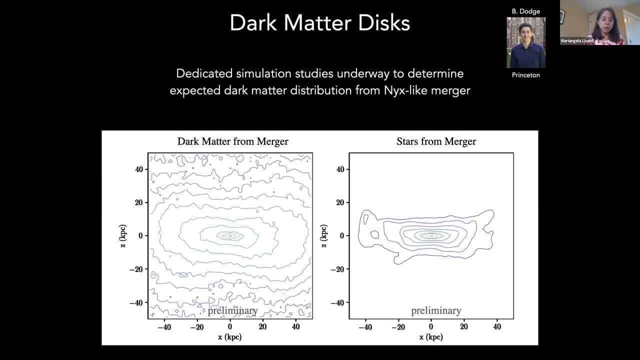 for the dark matter, but they would be an indication that you would also have a component in the dark matter that's behaving in a similar way. Thank you, Another question. I think you'll begin with a talk to mention the dark matter. hello, hello, version one. 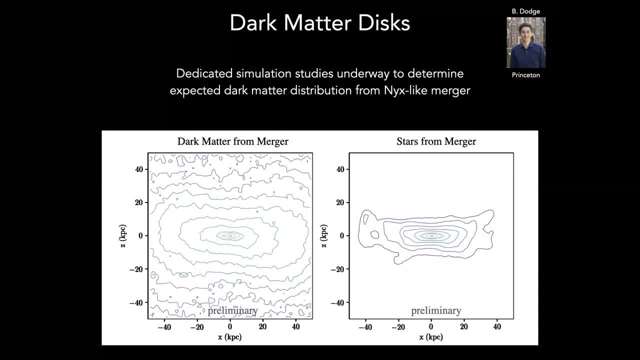 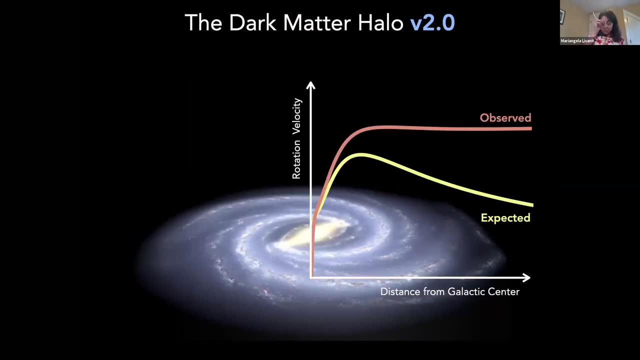 And with dark matter. hello version two. Just make sure, when was the transition from one to two? I mean, that was kind of- perhaps somewhat- heuristic here, but I don't think we're done with version two. put it that way. 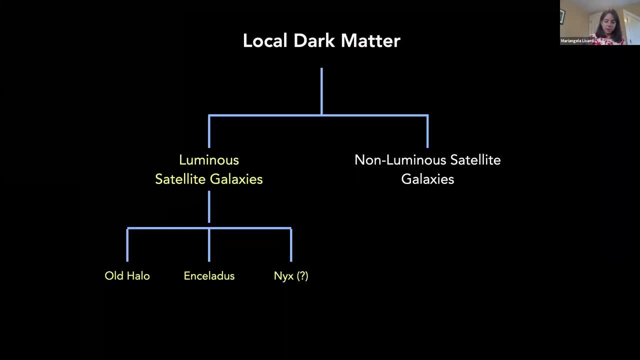 So version two is in progress. I mean here, I mean here's where we're at right. So I think, when I would claim that version two is done, when we have a solid understanding of the dark matter that came from the luminous satellite galaxies, 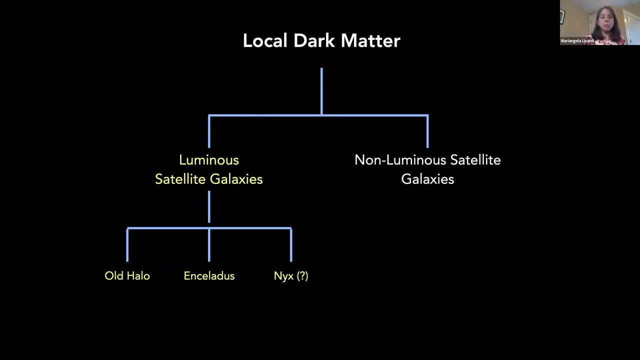 I think that's a big step forward And I think we're getting there, especially because we've been. the big boom there came from the Gaia data, So those advancements really just came in the last two years following the second Gaia data release. 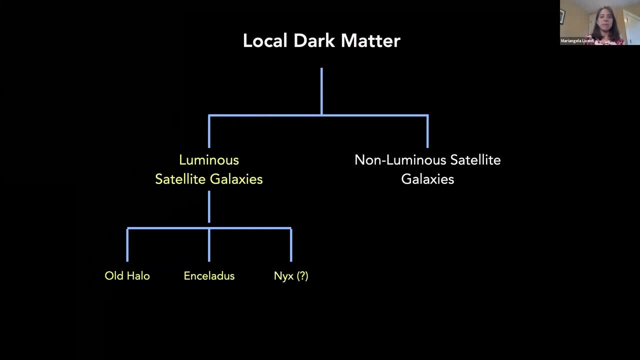 I would argue that version three, which we have yet to embark on but is going to be the more complete picture, is going to include the dark matter that comes from these satellite galaxies that don't have any stars in them. The challenge there is obviously that. 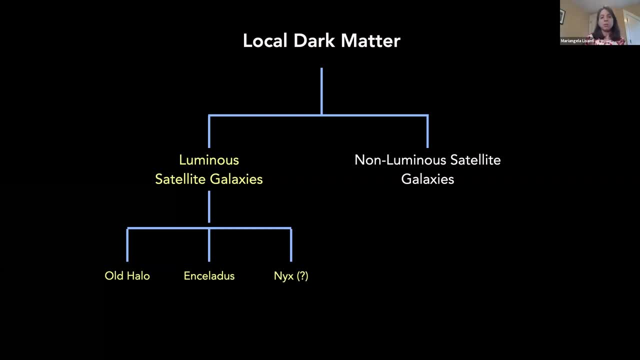 you know, what we've been able to, the thing we've been able to harness, to make progress, is really the fact that we have some kind of tracer in these galaxies, the stars, and we can see those tracers. The challenge with this arm here. 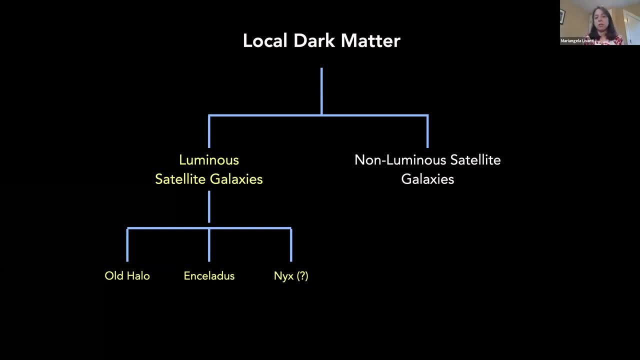 is we no longer have the stars as being the tracers for those galaxies, So we're going to have to figure out other ways of tackling it. Thank you very much. I have one more question, but in case there are other people who want to ask, 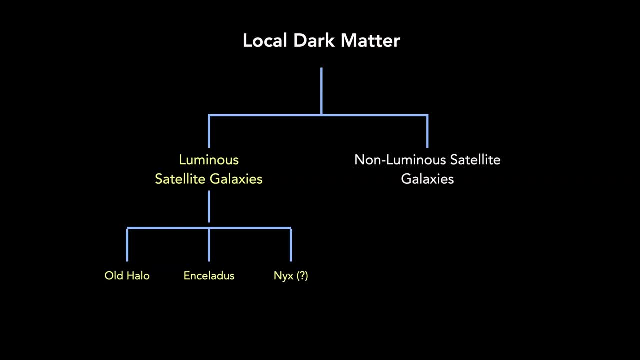 maybe they should ask first, Otherwise I can ask one more question. Maybe I'll go ahead first. So the dark matter, version one. I think the simulation data is using the collisionless fluid and with some phase-based solution such as Maxwell-Boltzmann distribution. 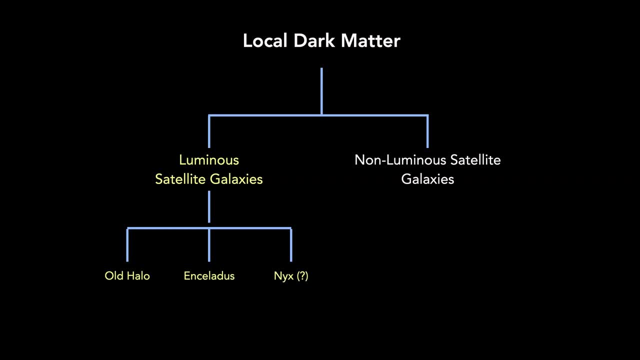 isosimilar density, et cetera. I wonder how the fitting is constrained by maybe the universality cost of the data, the input that you need to input, Like if you vary a bit the distribution. does that matter And how is that compared to further analysis? 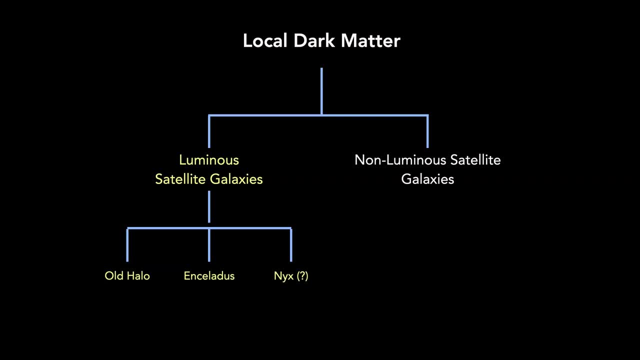 that you did later, when you try to maybe simulate dark matter, Do you always start with this type of model, this collisionless fluid? Yeah, that's a really good question. So all of the simulation data that I've shown here has been making the assumption. 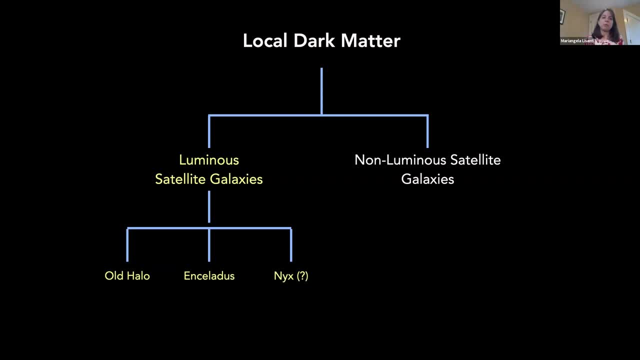 that the dark matter is collisionless. The model we refer to the model as cold dark matter model. That's the dominant paradigm, but there's certainly very well-motivated modifications on that. So, for example, you can consider the case where the dark matter is allowed. 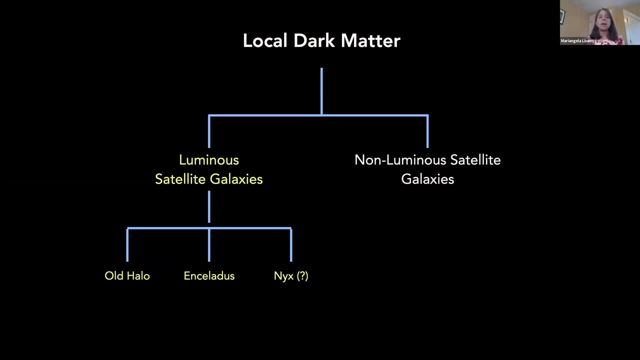 to interact with itself. So it's like a self-interaction. And we have started looking at what happens to this picture if the dark matter model is not cold and is instead, for example, self-interacting, or perhaps if there's some certain amount. 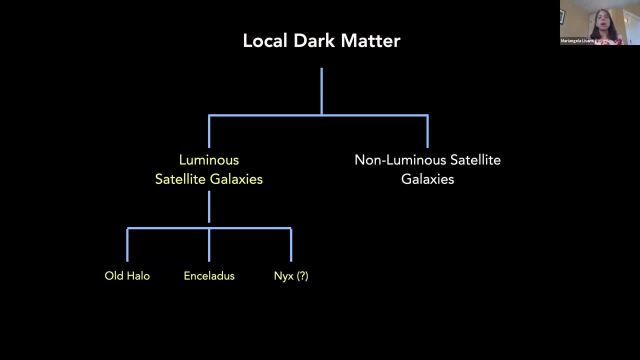 of dissipation in those self-interactions And it will end up changing the correspondence between the dark matter distribution and the stellar distribution. So one of the reasons why you get such a nice mapping between the stars and the dark matter in the case of cold dark matter. 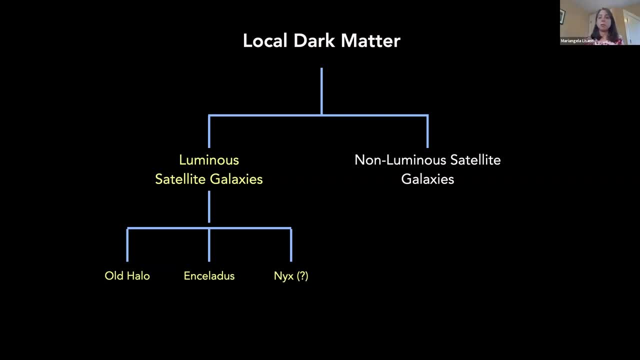 is because both the stars and the dark matter are collisionless- effectively collisionless- So they act very similarly in their evolution. Now, if you change the dark matter model so that it's, for example, self-interacting, then you're breaking that tie. 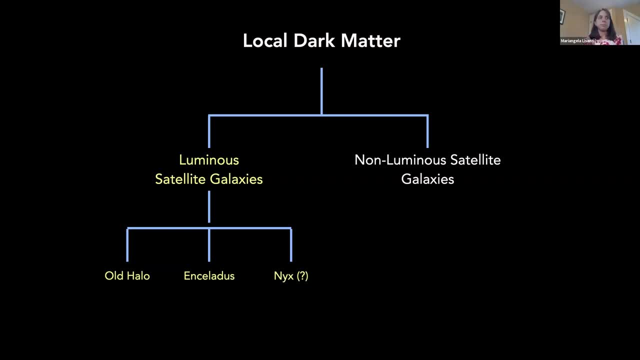 between the two, And in that case you will end up seeing some differences in the distribution. So that's work in progress, But it's really important to understand exactly how these conclusions are affected by the properties of the dark matter model, So it's something that we definitely 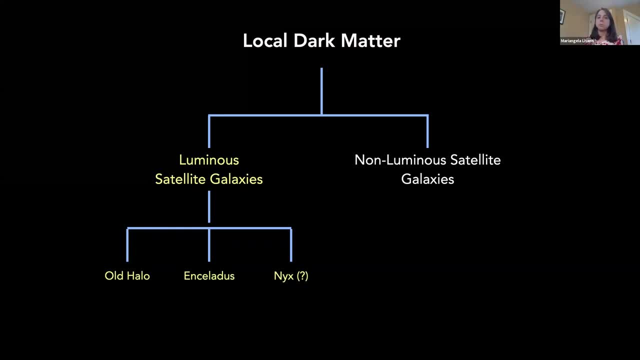 need to explore further. Fortunately, we have the tools to be able to do so, because we can model these self-interactions and also these dissipative interactions in the simulations. Yeah, that's exactly the point, Just how much the methodology of the model of your dark matter. 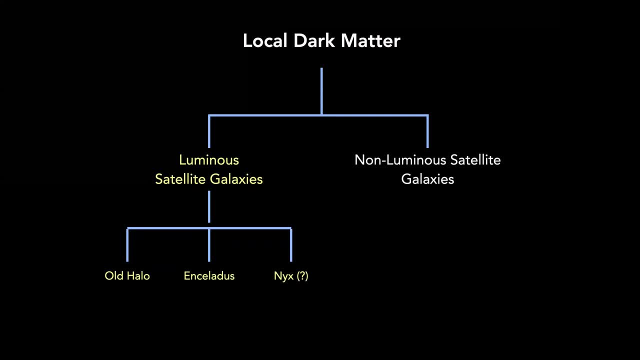 affects your conclusion. I think that's the thing I want to maybe understand or separate. Maybe there are some more universal conclusions, independent from which dark matter model you use, or part of the how, part of the conclusion might be affected by the model you use. 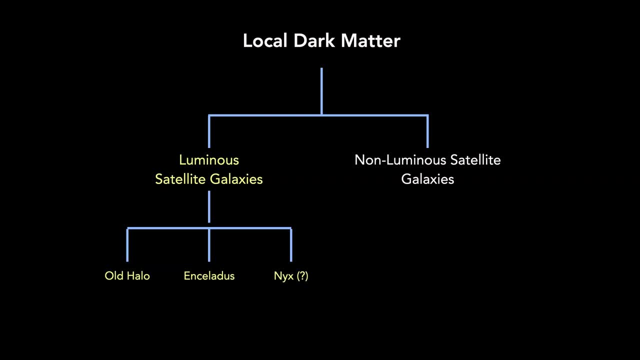 Is this possible to be stated? So what the what I'm sketching here on this slide? these conclusions won't be any different. So there will still be components of dark matter. The relative fractions of the components of dark matter coming from these different origins. 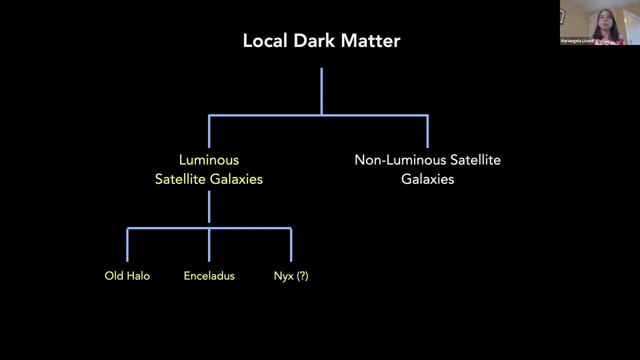 would still be the same, regardless of whether or not the dark matter is self-interacting or cold, for example. What may change is the actual velocity distribution of the dark matter, let's say from Enceladus, If the dark matter is self-interacting. 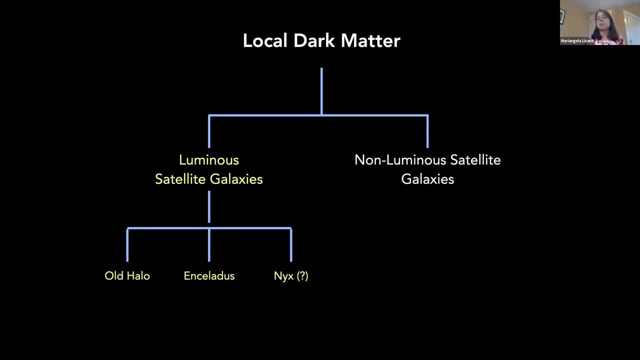 versus cold, the velocity distribution of the dark matter from Enceladus will look different. But all that means is that when we sort of put forward like a final distribution of that local dark matter map, we could just have several different like categories, right? 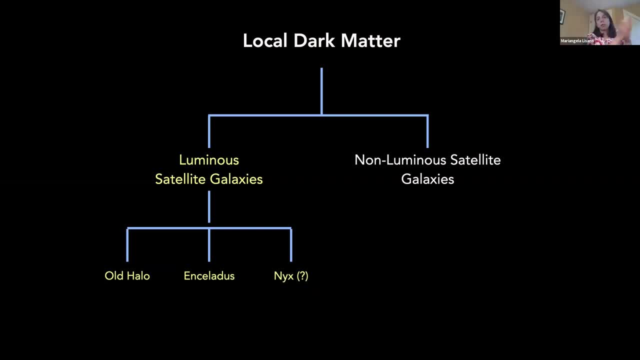 If the dark matter is cold and we expect the distribution to look like this, If it's, if they're self-interactions, then we can predict a distribution that looks like this right. So when we look at the dark matter, we should be able to get: 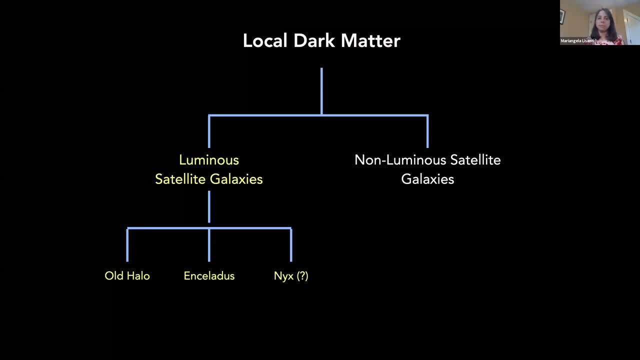 a good handle on that from the simulations. But what I've drawn here on this slide here, that won't change if you change, if you, let's say, switch from cold dark matter to self-interacting dark matter. Yes, thank you very much. 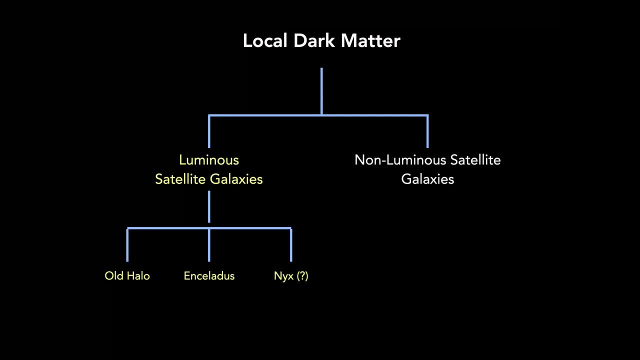 Actually, one last thing, Since dark matter is, in general, maybe defined in a way, they are matter but not belong to the standard model sectors. So if we have a like experimental data, is there a way we can just interpret dark matter by its own, independent from? 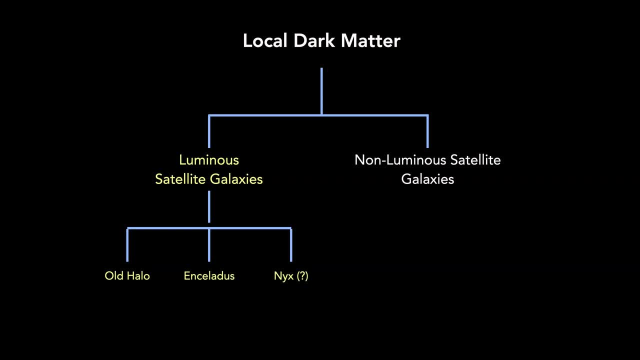 what model we are using, But it seems like some of the analysis depends on the data input that we need to assume certain dark matter model. So that's the part I feel like I'm not understand enough: Which part we need to assume that there is certain dark matter model. 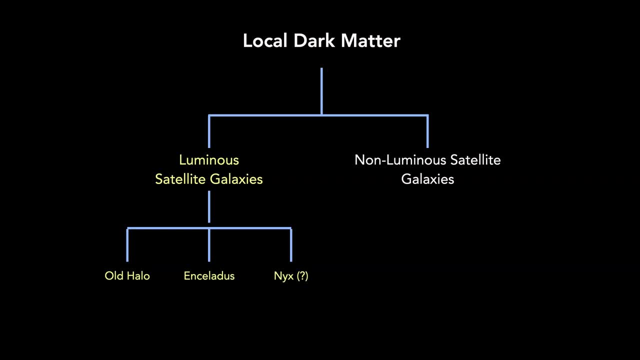 need as an input and which part we can just interpret from the experiments, Based on the fact that dark matter doesn't interact at this, doesn't interact to the strong force and electromagnetic force, can we already read from the experiment data that we can just tell? 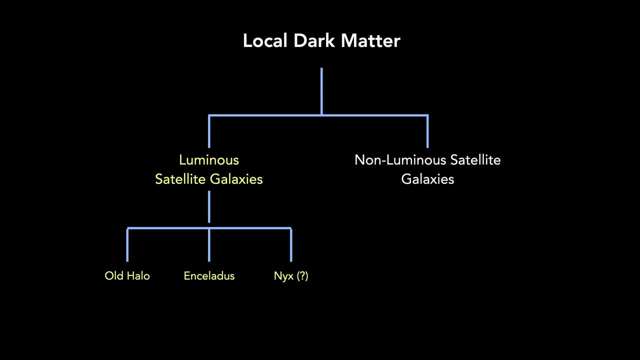 which part is from the dark matter. It seems like there's an input that you need to, you need to, you need to consider when you do the analysis. So, from this, from this angle, where we're trying to build up that dark matter distribution, 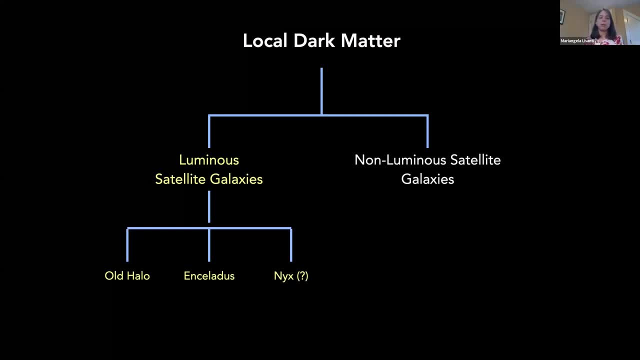 from astrophysical observables. what we'll ultimately end up having is options for what that dark matter distribution will look like, depending on the properties of the dark matter particle, You know. so it'll be like option A, B, C, where A might be like. 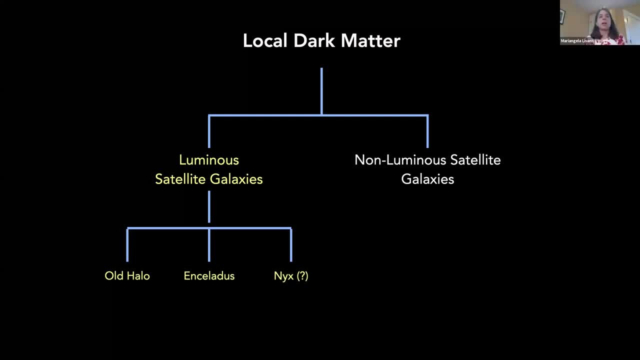 if it's cold, B if it's self-interacting, et cetera. Then let's say that you have an experiment, a terrestrial experiment, that runs and actually sees a signal And, based off of the signal that they would see, they can get.